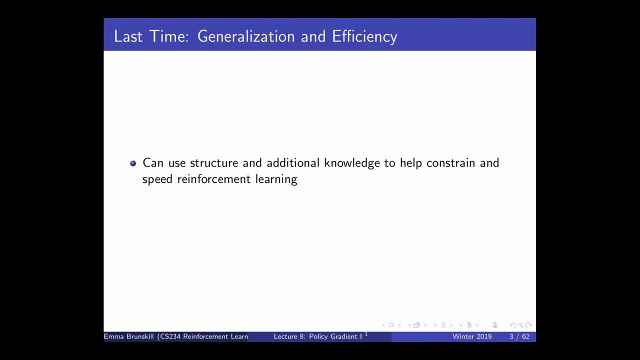 could try to learn how to do things faster, And imitation learning was one way to provide structure or support by leveraging demonstrations from people, And we've seen other ways to sort of encode structure or human prior knowledge when we started talking about function approximation. So when we think about how we define Q, like when we define 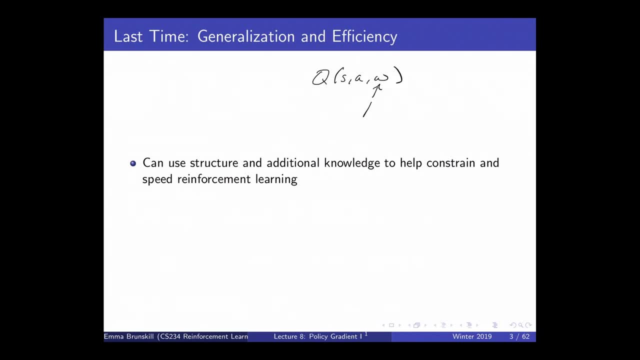 Q as S, A and W, where this was a set of parameters. we were implicitly making a choice about sort of imposing some structure in terms of how we were going to represent our value function, And that choice might be fairly strong, like assuming that we're going to be able to do this. 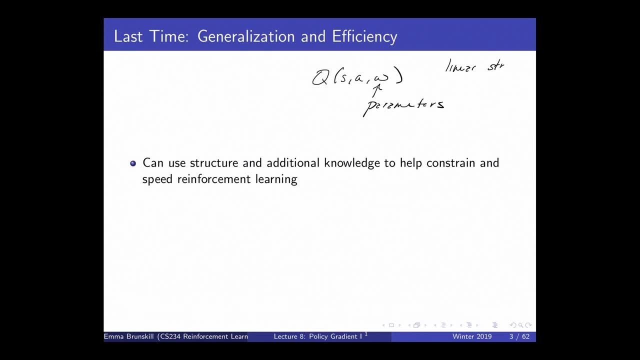 by assuming it was linear. So this is sort of quite a strong assumption. Or it might be a very weak assumption, like using a deep neural net, And so when we specify sort of these function approximations and representations, we're sort of implicitly making choices about how much. 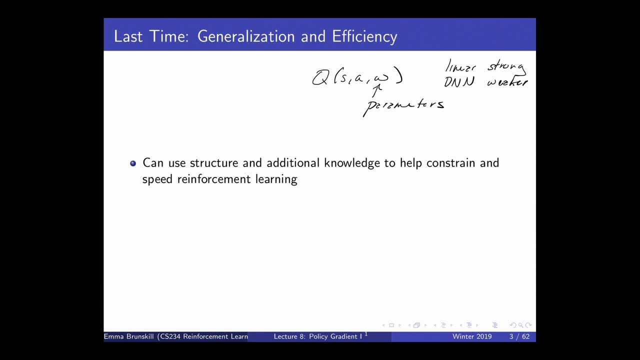 structure and how much domain knowledge we want to put in in order for our agents to learn. So what we're going to start to talk about today, and what we're going to talk about this week, is policy search, which is another way to do this, And it's a very, very important thing to do. 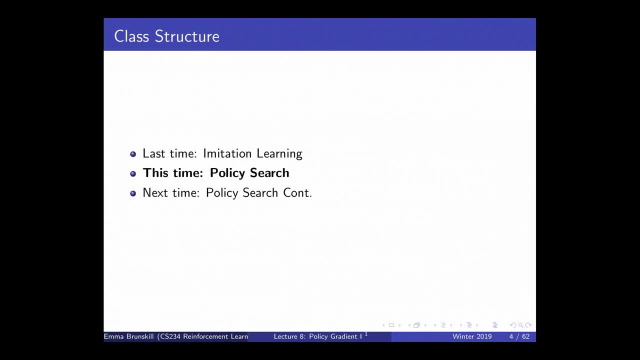 It's another place where it can be very natural to put in domain knowledge- And we'll see that in some robotics examples today- And it can be also a very efficient way to try to learn. So, as I was saying before, we sort of were approximating when we were doing model-free. 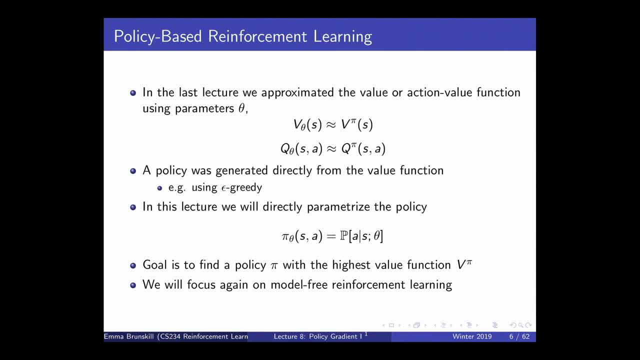 reinforcement learning and when we started to try to scale up to really large state spaces. I've been having several different people ask me about really large action spaces, which is a really important topic. We're not going to talk too much about that in this quarter. 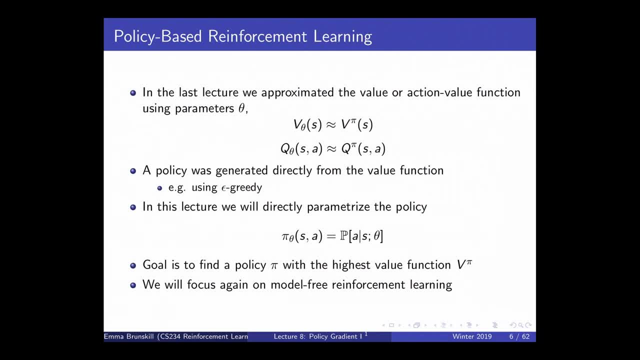 Though we will talk a little bit about when your action space is continuous but low-dimensional, But we have started to talk a lot about when the state space is really high-dimensional and and and really large, And so we talked about approximating things, um, uh, with some sort of 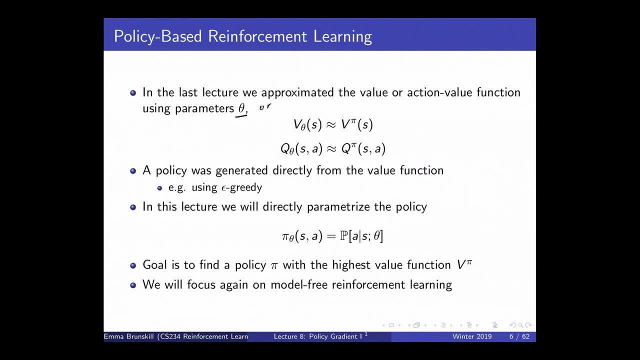 parameterization, like whether it be parameters theta, or we often, or we often use w, But some sort of parameterization of the function, And so we used our value function, um, to define the expected discounted space, and then we used our value function to define the expected discounted space. 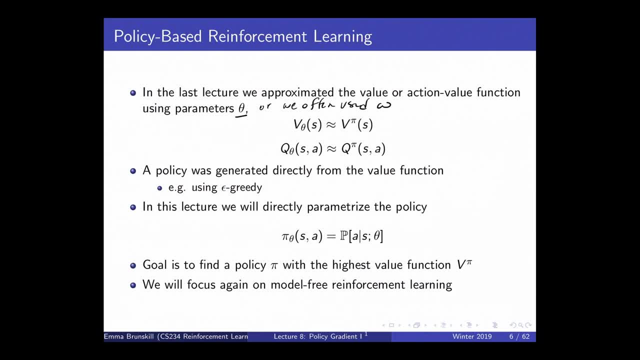 And so we could take some of rewards from a particular state or state action, and then we could extract a policy from that value function, or at least from a state action value function, And instead what we're going to do today is just directly parameterize the policy. 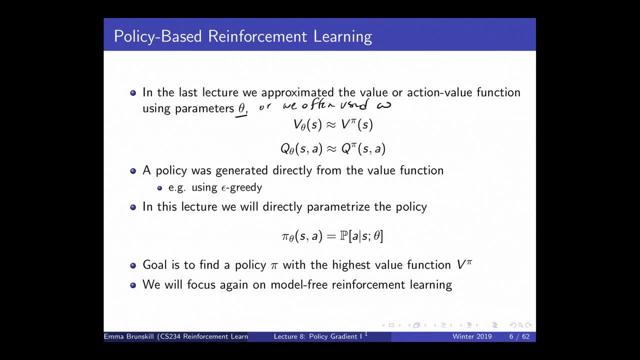 So when we talked about tabular policies, our policy was just a mapping from states to actions And in the tabular setting we could just look- do that as a lookup table For every single state. we could write down what action we would take. 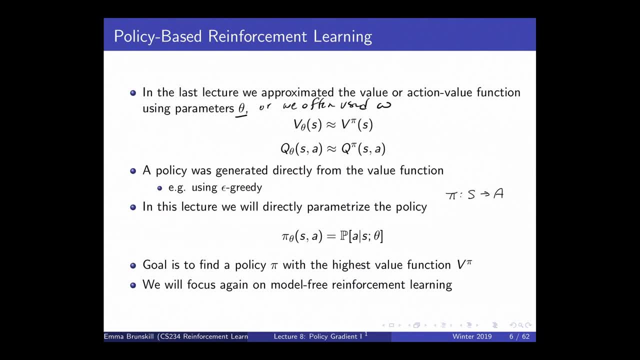 Um, and what we're going to do now is to say: well, it's not going to be feasible to write down our table of our, our policy, so instead, what we're gonna do is parameterize it And we're gonna use a set of weights or thetas. 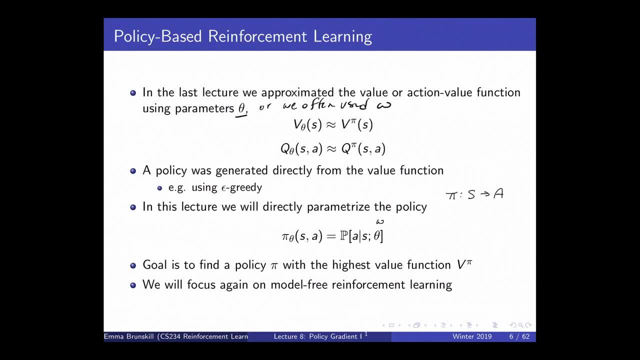 Today we're mostly gonna use thetas, but this is- could equally well think of this as weights- Um, just some way to parameterize our policy, And we'll talk more about particular forms of parameterization. Um, but, just like what we saw for state action value functions. um, this is gonna have a big implication because this is effectively defining the space that, um, you can use. So, um, we're going to take some of that data and then we're gonna look at a set of weights or thetas. 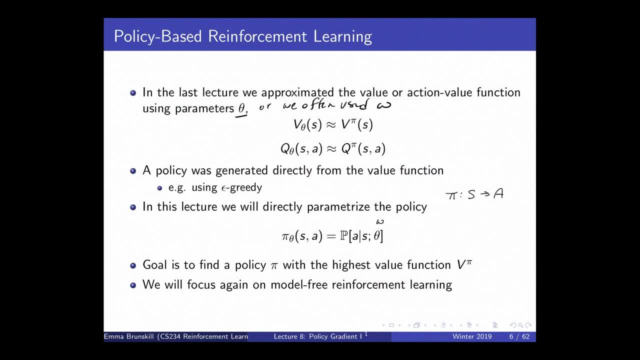 Um, but this is gonna have a big implication because this is effectively defining the space that you can use in your policy, mining the space that you can learn over. So it's sort of um, it's determining the, the class of policies you could possibly learn. 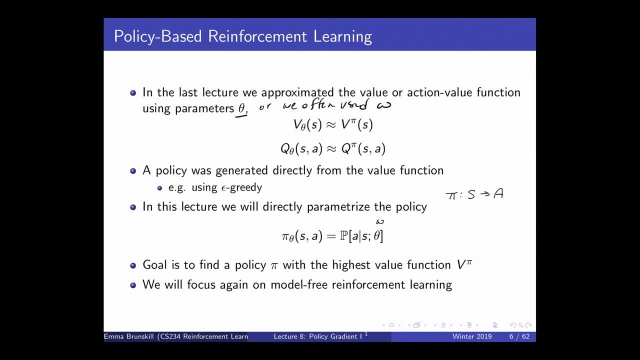 Um, and we're again going to sort of focus on model-free reinforcement learning, meaning that we're not going to assume that we have access to an a priori model of the dynamics or reward of the world. So we had sort of some of these diagrams up at the start of the quarter. 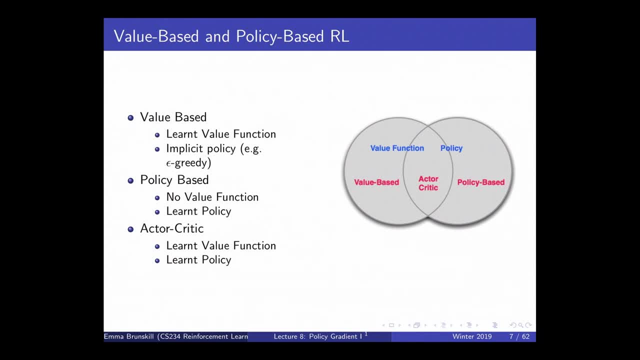 I just want to go back to it. Um, we've been talking about sort of value. We we haven't talked so much about models. The models are also super important, Um, but we've been talking a lot about sort of value, function-based approaches. 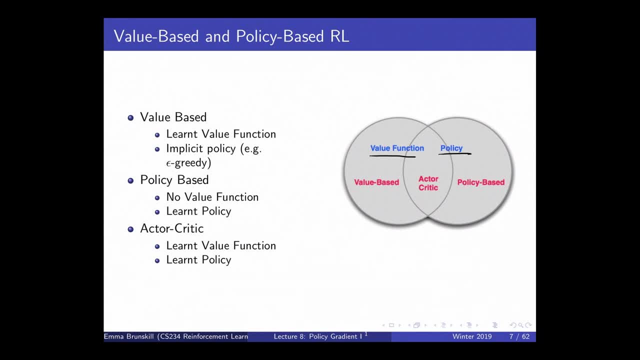 which is this, And now we're going to talk about policy, um direct policy, search methods, And, as you might expect, there's a lot of work which tries to combine between the two of them, And these are often called actor-critic methods. um. 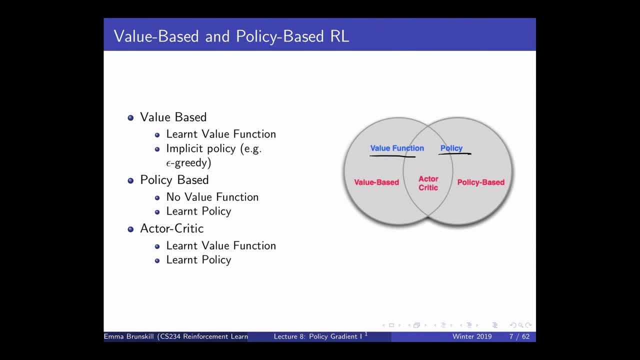 where you try to explicitly maintain a parameterized policy and explicitly maintain a parameterized critic or value function. So this is the policy and this is a Q, Okay. So we're going to start today and we're going to be talking about policy-based methods. 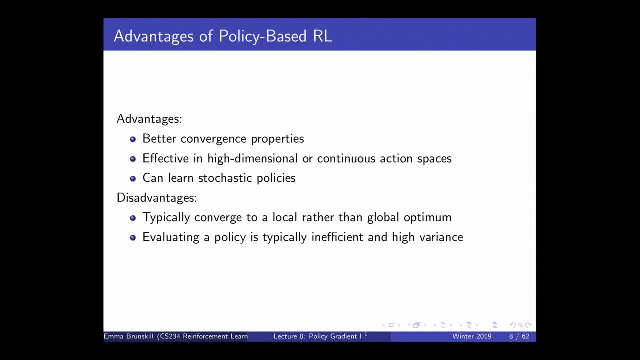 So why would you want to do this? Um well, uh, it actually goes back a little bit to also what we were talking about last week with imitation learning. For imitation learning, we talked about the fact that sometimes it's hard for humans to write down a reward function. 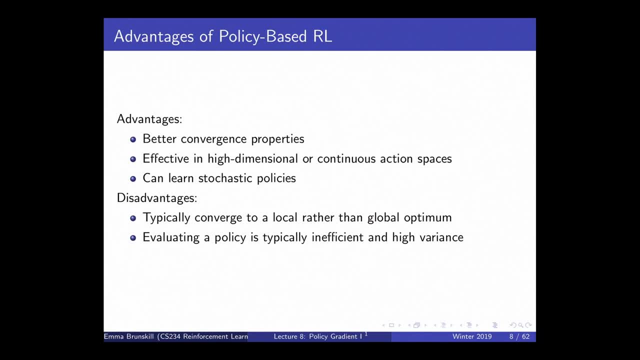 and so it might be easier for them just to demonstrate what the policy looks like. Similarly, in some cases maybe it's easier to write down sort of a parameterization of, um, the space of policies than it is to write down a parameterization of the space of state action value functions. 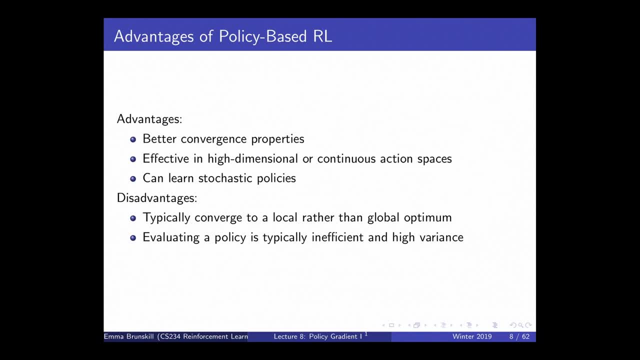 Um. in addition, they're often much more effective in high-dimensional or continuous action spaces and they allow us to learn stochastic policies, which we haven't talked very much about so far, but I'm going to give you some illustrations about where we definitely want stochastic policies. 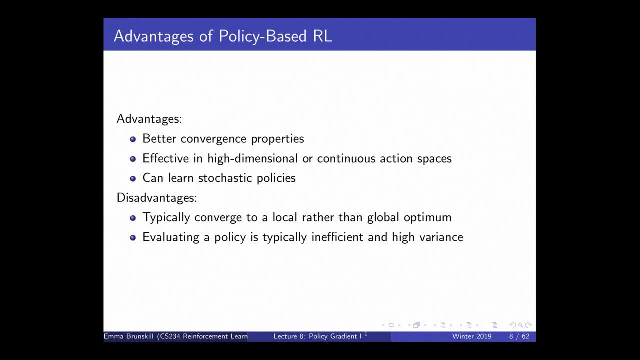 Um, and they sometimes have better convergent policy- convergence uh properties. Um, that can be a little bit debated. It depends exactly what uh, whether we're comparing that to model for your model-based approaches and how much computation we're doing. 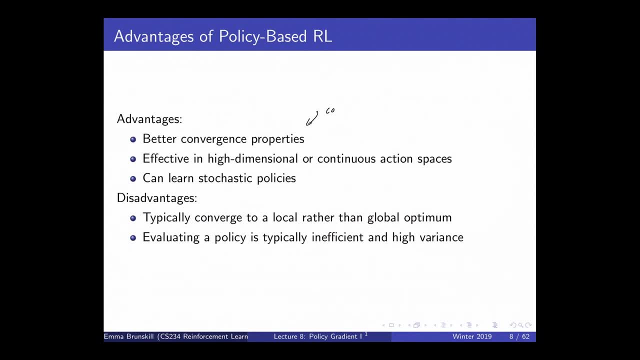 Um, so this can be a little bit of a function of computation too. Computation can matter. One of the really big disadvantages is that they are typically only gonna converge to a local optima, So we're going to converge to something that is hopefully a pretty good policy. 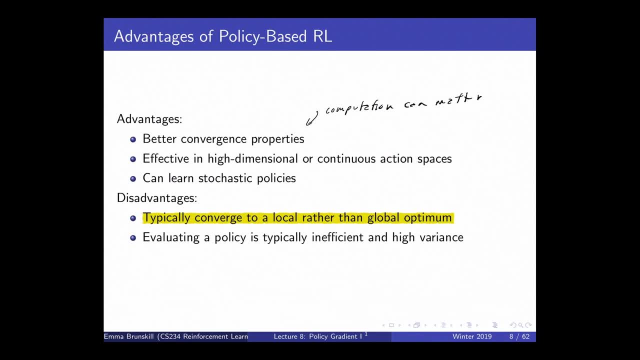 but we're not generally guaranteed to converge to the global optima. Now there are some techniques that are guaranteed to converge to the local optima, to the global optima, and I'll try to highlight some of those today, but generally, almost all of the methods that you see in like 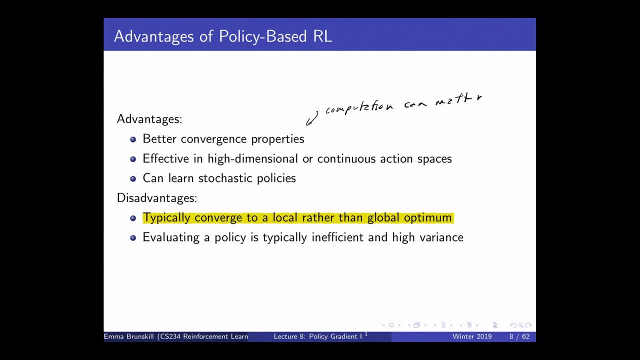 deep reinforcement learning that are policy gradient-based um only converges to a local optima Um. and then the other challenge is that typically we're going to do this by trying to evaluate a policy and then estimate its gradient, and often that can be somewhat sample inefficient. 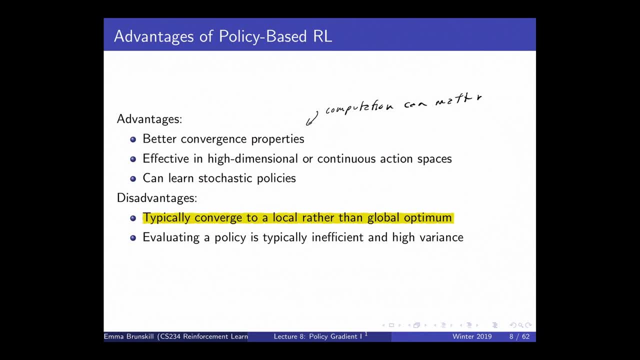 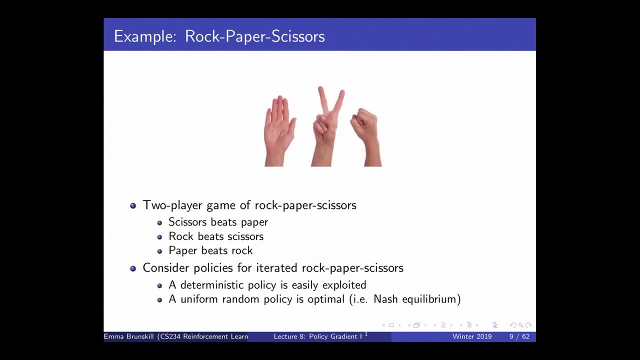 So we might need quite a lot of data to estimate, um, what that gradient is when we're taking a gradient-based approach. So why might we want sort of a stochastic policy? So in what I mentioned before, um in the tabular setting? 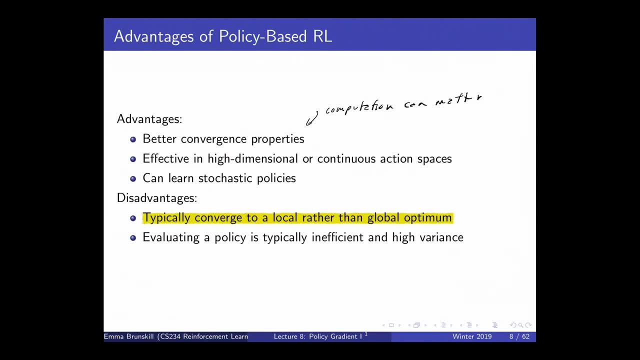 so let me just go back to here. So, in um, you know why do we want this? Do we want this If you think back to sort of the very first lectures? um, what I said is that if we have a tabular MDP, 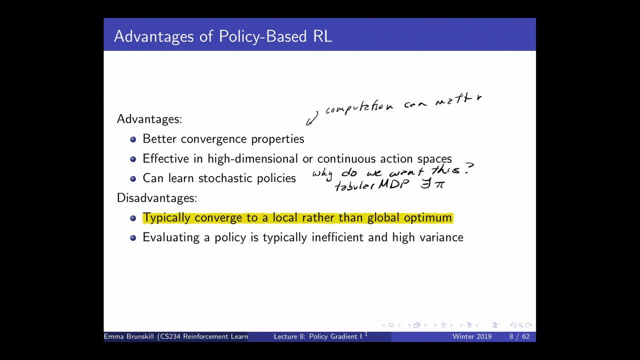 there exists a pie which is deterministic and optimal. So in the tabular MDP setting we do not need um uh, deter-, we do not need stochastic policies, because there always exists a policy that is deterministic, that has the same value as the optimal policy does. 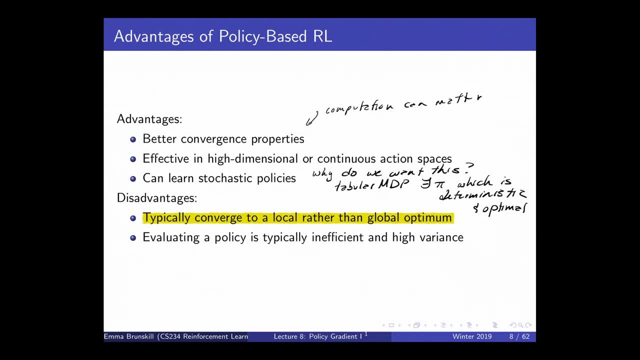 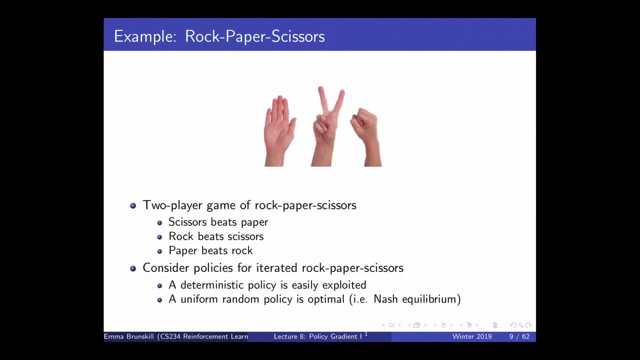 So this is not needed in the tabular Markov decision process case. But we don't always- we're not always- acting in the tabular Markov decision process case. So as an example: um, uh, who here is familiar with rock-paper-scissors? 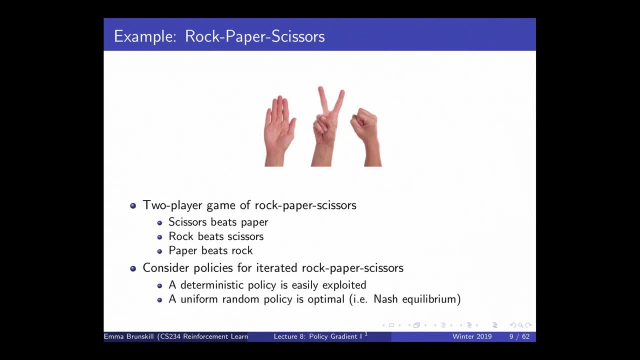 Okay, Most people. Um, uh, possibly, if you're not, you might have played it by another name. So in rock-paper-scissors, uh, it's a two-player game. um, everyone can either pick uh, paper or scissors or rock. 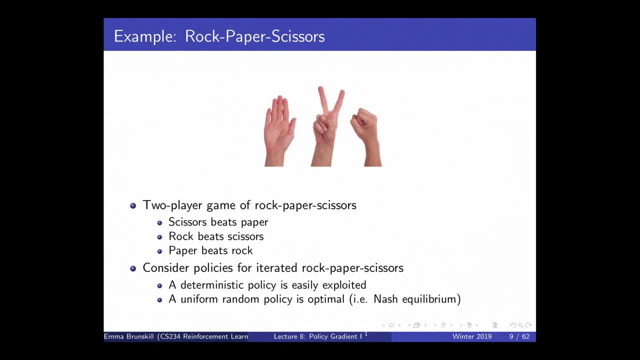 and you have to pick one of those. and scissors beats paper paper- rock beats scissors and paper beats rock Um. and in this case, if you had a deterministic policy, you could lose a lot. You could easily be exploited by the other agent. 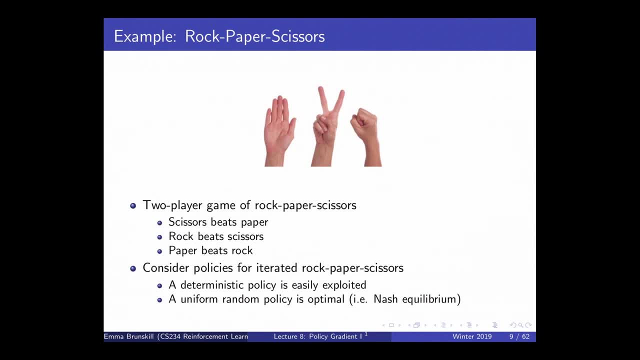 Um, but a uniform, random policy is basically optimal. What do I mean by optimality In this case? I mean that you you get a, say a plus one if you win, and, um, let's say zero minus one if you lose. 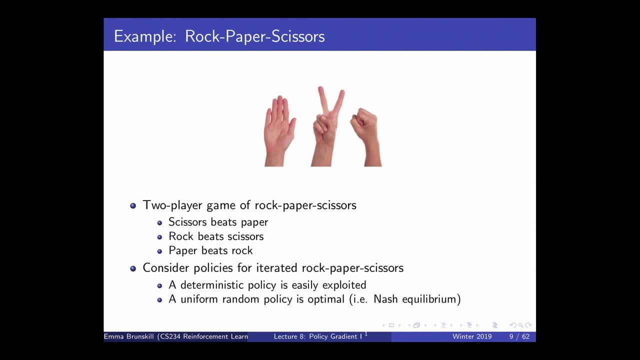 Now we're not gonna talk too much about multi-agent cases um, uh, in this class, but it's a super interesting area of research. Um, and in this case, um you know, the environment is not agnostic. Um, the environment can react to uh. 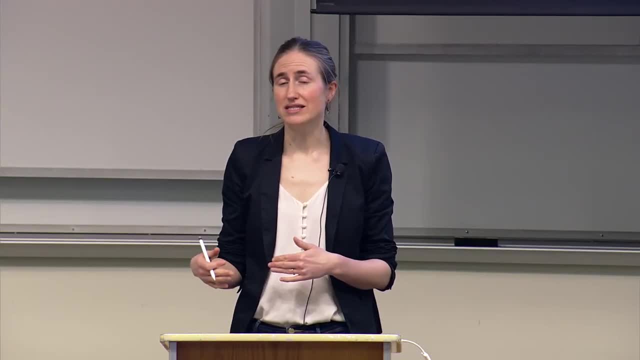 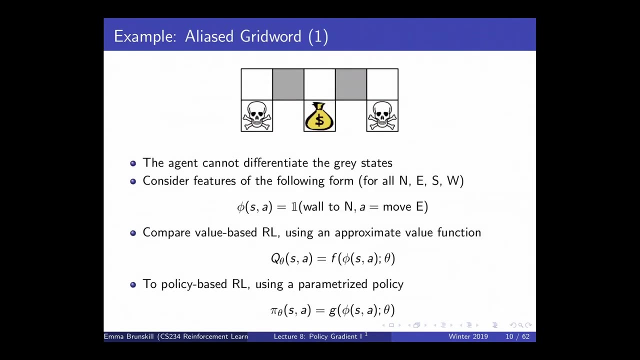 the policies that we're doing and and can be adversarial, And so we want a policy that um is robust to an adversary. So a second case: um is alias grid world, So um. so in this case, 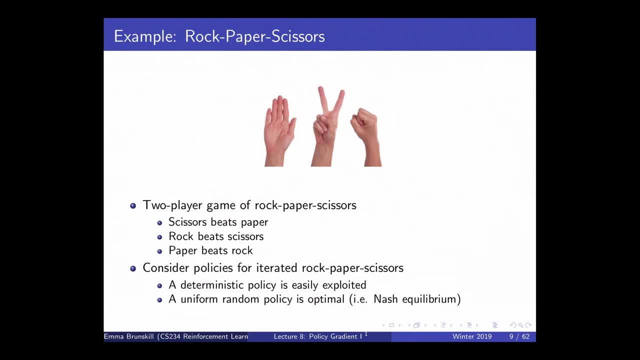 so why? you know why is being stochastic important here? Well, because we're not really in a stochastic setting. we're in an adversarial setting and we have another agent that is playing with us and they can be non-stationary in changing their policy in response to ours. 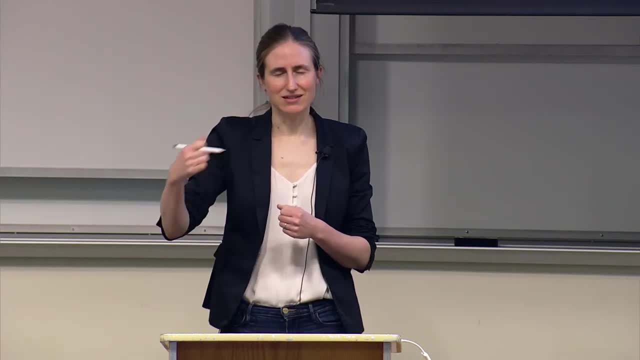 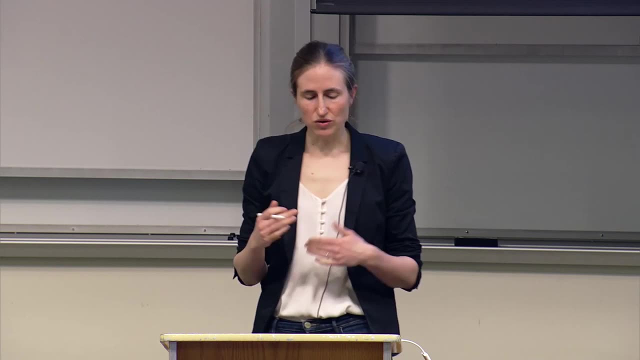 Um. so it's not a- the environment doesn't pick the next- it doesn't pick rock paper scissors, regardless of our actions Um in the past. it can respond to those Um. so it's sort of got this non-stationarity or adversarial nature. 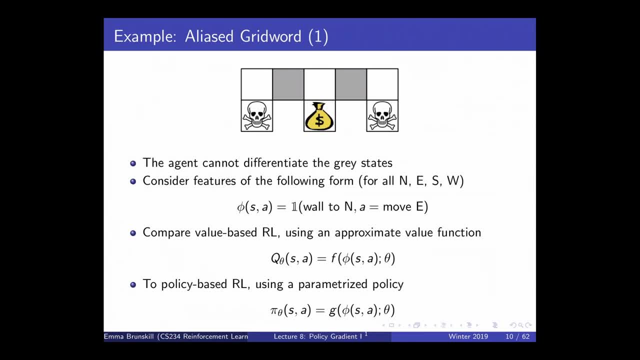 Um, another case is where it's not Markov, So it's really partially observable and you have aliasing, which means that we can't distinguish between multiple states in terms of our sensors. So we saw this before a little bit when we talked about robots. that 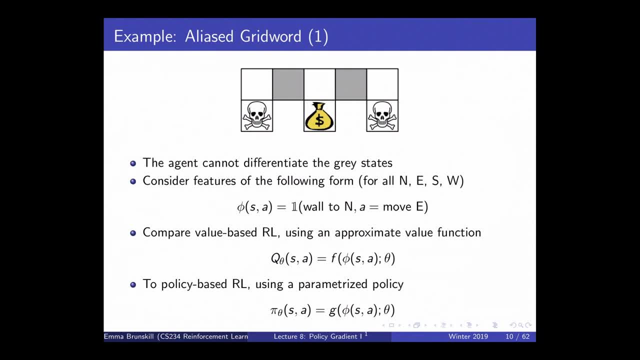 you know, could have laser range finders and sort of tell where they were in a hallway by how far away each of the um the- the first point of um uh uh obstacle was for all of their 180 degrees. 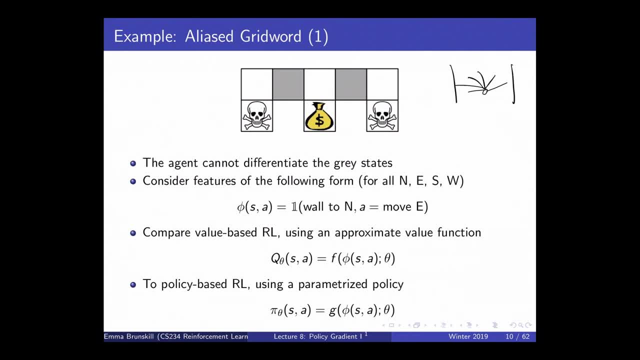 And so that would look the same in lots of different hallways. Um, so this is a simple example of that. So in an alias grid world, um, let's say that the agent, because of their sensors, cannot distinguish the gray states. 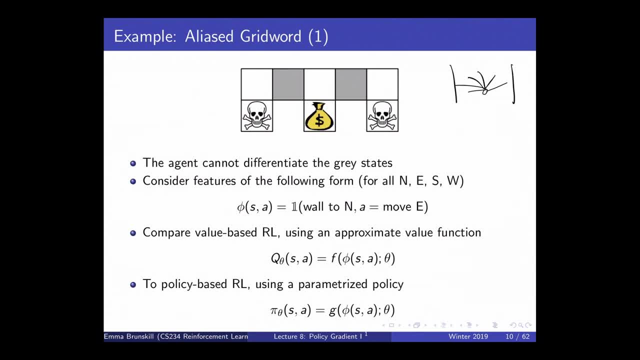 and they have features. they have a particular form, Um, they have a feature for whether or not there's a wall to the north, um, uh, or east, or south or west, So it can basically like if it's here. 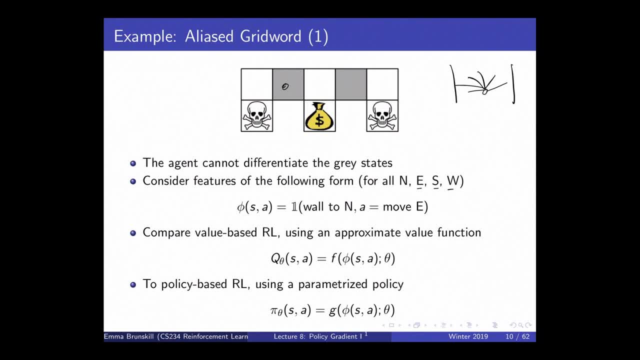 it can tell like: oh, I have walls to either side of me and not in front or behind me, Um, but that could be the same over in that- in- in the other um gray state. So if we did a value-based reinforcement learning approach, 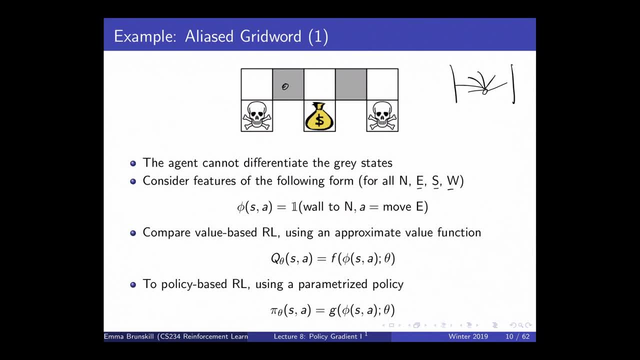 using some sort of approximate value function. um, it would take these features, which are: are a combination of what action am I gonna take and whether there are walls around me or not? Um, or we could have a policy-based approach which also um takes in these features. 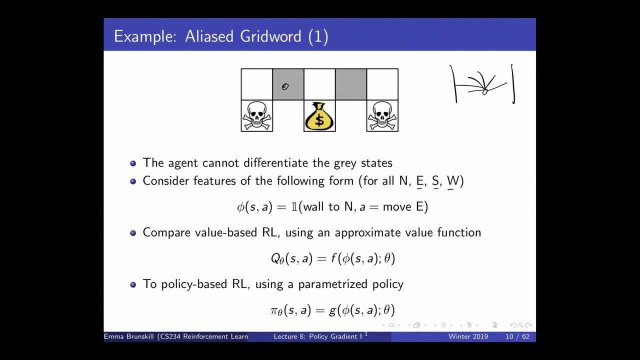 but then just directly tries to make decisions about what action to take, and those actions can be stochastic. So in this case, the agent is trying to figure out how to navigate in this world It really wants to get to here. This is where there's a large reward, so this is good. 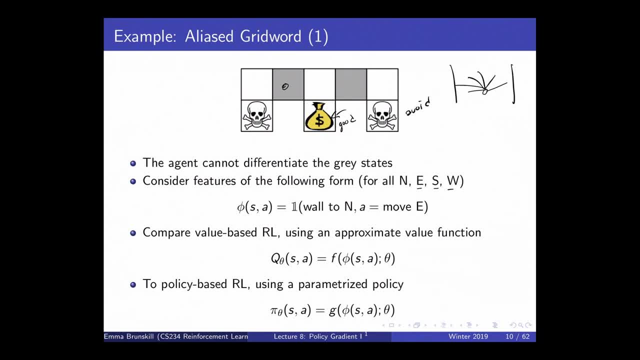 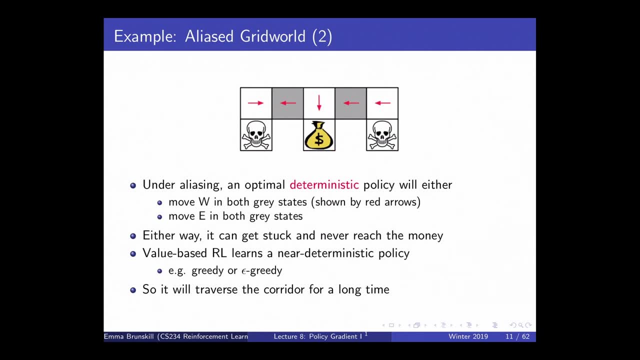 It wants to avoid the skull and crossbones, and those will be negative reward. So because of the aliasing, the agent can't distinguish whether or not it's here or here, Um, and so it has to do the same thing in both states. 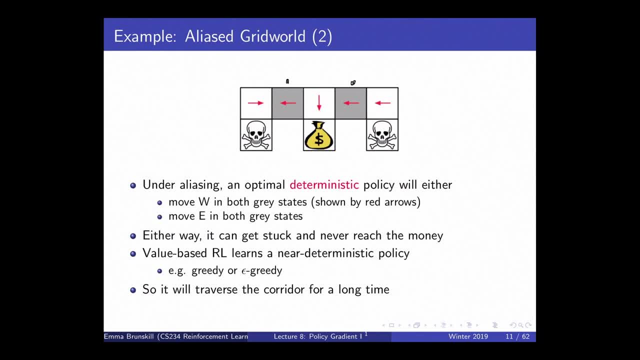 And so either it has to go left or it has to go right. you can call it west or east, Um, and either way that's not optimal, because if it's actually here, it should be going that way, not over here and down. 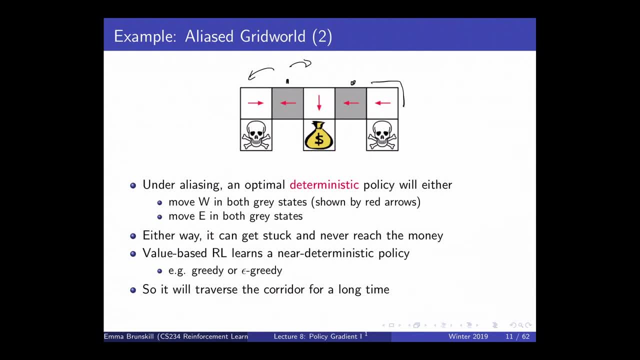 Um, and so it can distinguish whether it's in here or here, but it could just end up moving back and forth or making very bad decisions, And so it can get stuck and never be able to know what it's safe to go down and reach the money. 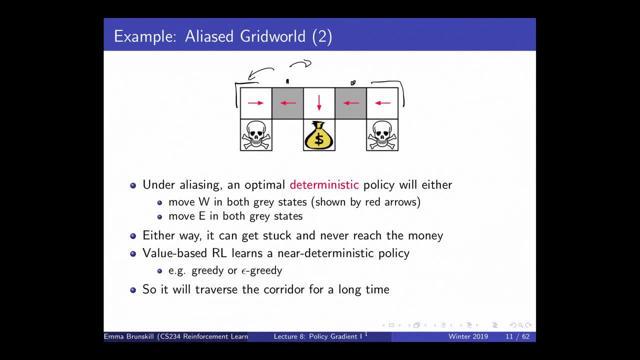 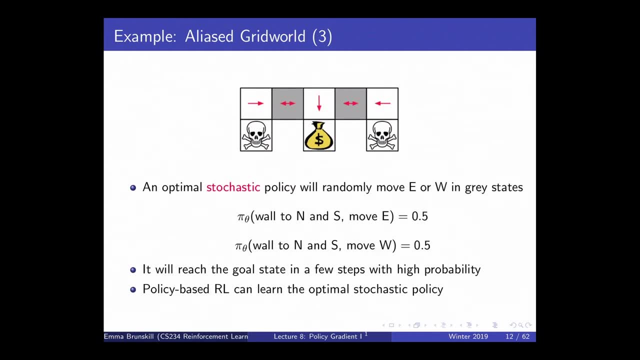 So it learns a near deterministic policy, because that's what we've normally been learning with these Um, and whether it's greedy or e-greedy, in general it will do very poorly. But if you have a stochastic policy when you're in a state where you're aliased, 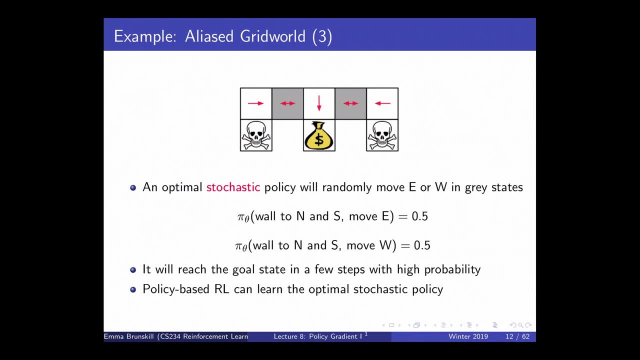 you could just randomize. You could say: I'm not sure whether I'm actually in this state, in this state or this state, um, so I'll just go, uh, either east or west, with 50% probability, and then it'll generally reach the goal state quickly. 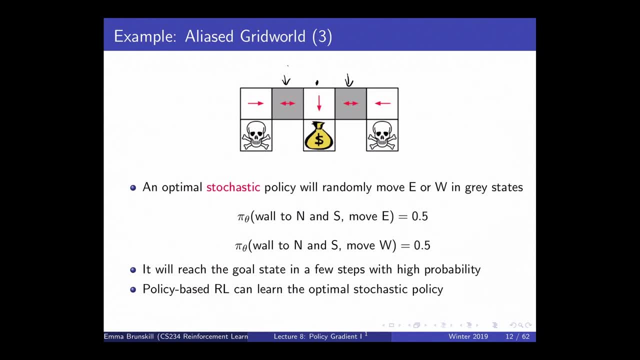 Because- note- it can tell what it should do when it reaches here, because that looks different than these two states. So once it's in the middle, it knows exactly what to do. So that's just again an example where a stochastic policy has a way better value than 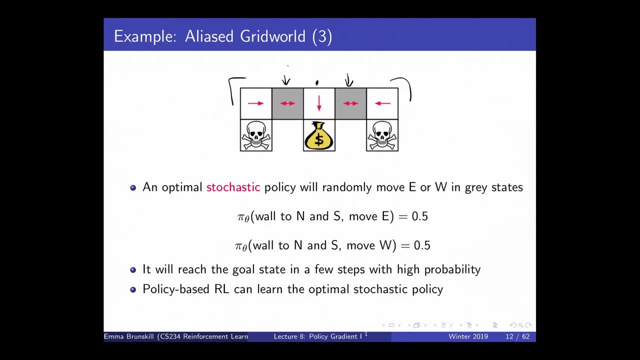 um, a deterministic policy, and that's because the domain here is not Markov. it's partially observable, Okay. So that's sort of one of the reasons why we might want to, some of the reasons why we want- might want to be. 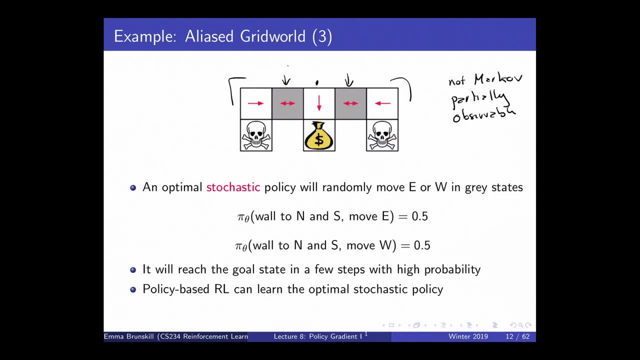 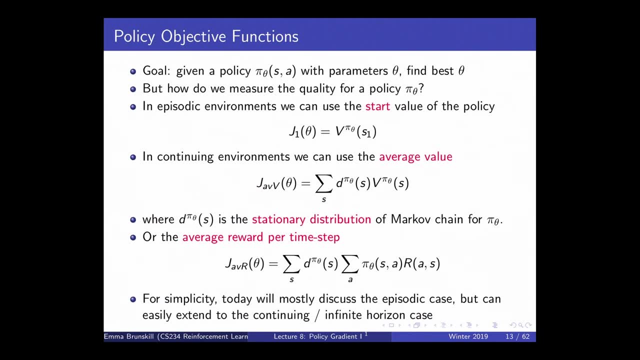 uh, directly policy-based, and there's a lot of other reasons, Um so- so what does this mean? Well, uh, we're gonna have this parameterized policy and the goal is that we want to find- yeah, 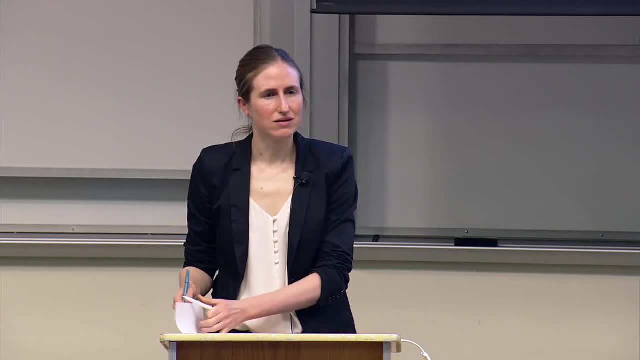 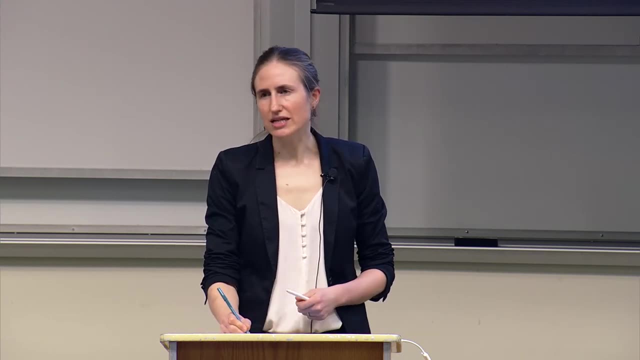 Can we conclude that when the world is not Markov, it's partially observable? Stochastic policies are always better. It's a great question, Sorry. yeah, So what you said is: can we conclude that, um, if the world is partially observable, 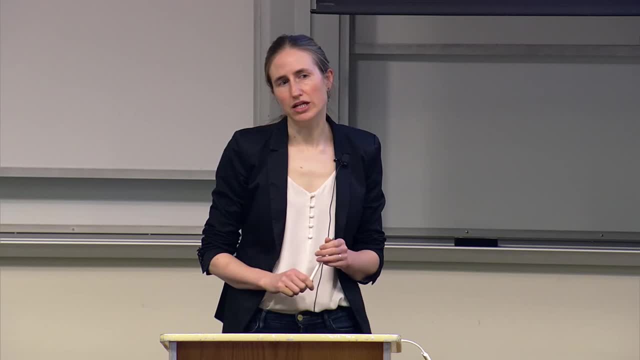 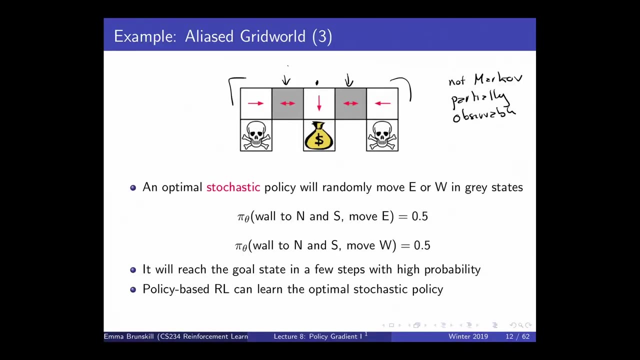 stochastic policies are always better. Um, I think it depends on the modeling you want to do. I think in this case, better than being stochastic- because it's still doing something kind of not very intelligent in the gray states, it's just randomizing- would be to have 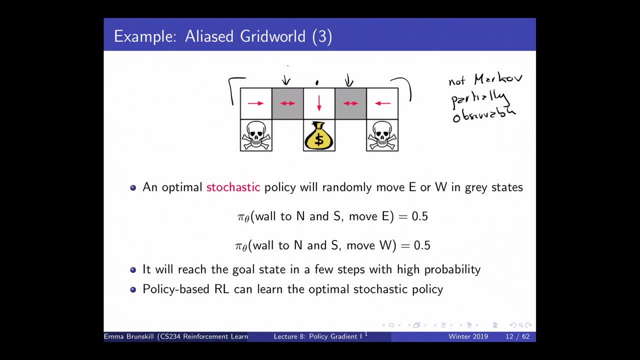 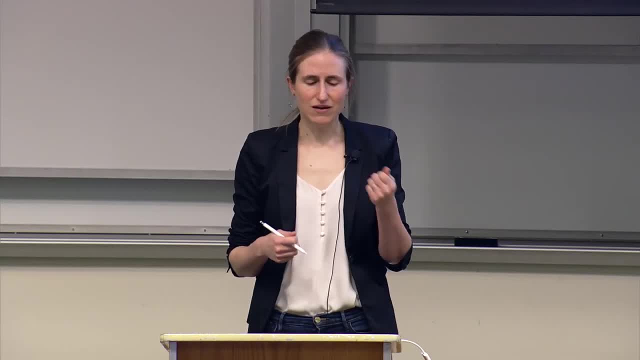 a partially observable Markov decision process policy, um, and then you could track an estimate over where you are in the world. So you could keep track of a belief state over what state you're in, and then you could hopefully uniquely identify that oh. 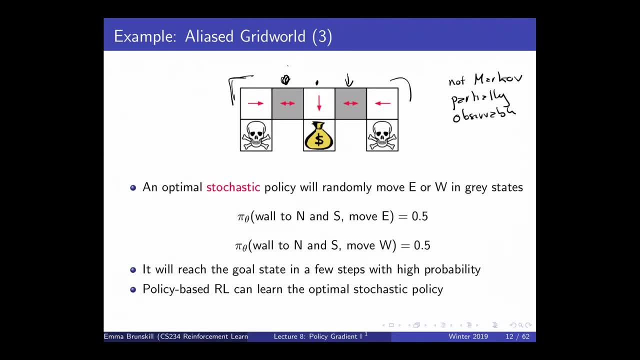 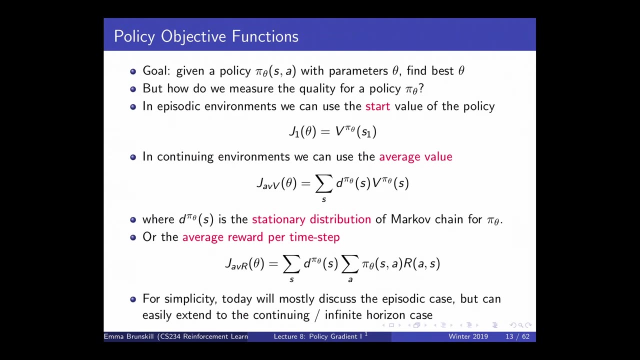 if I was just in this state. I have to be in this state now, And then you could deterministically go to the right or left. So it depends on- on the modeling one's willing to do. Good question, Okay. So when we um start to do the po-, go to parameterize policy search. 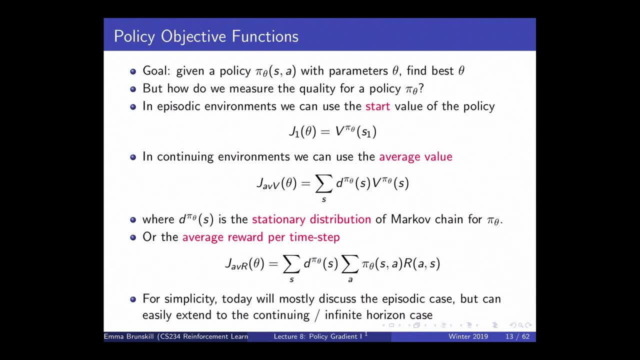 what we're gonna wanna do is find the parameters that yield the best value, the policy in the class with the best value, And so, similar to what we've seen before, we can- we can think about sort of episodic settings and infinite sort of continuing settings. 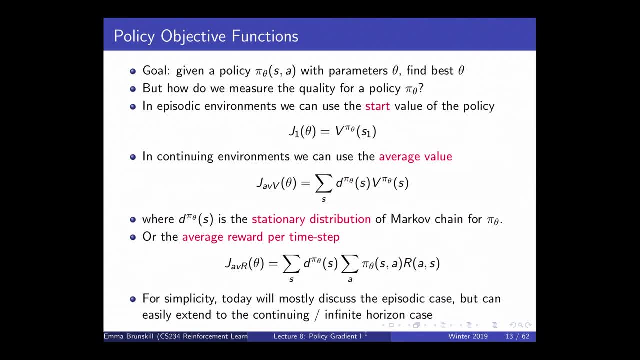 So in an episodic setting, that means that the agent will act for a number of time steps, often, let's say, h steps, But it could be variable, like it might be until you reach, you know, a terminal state. 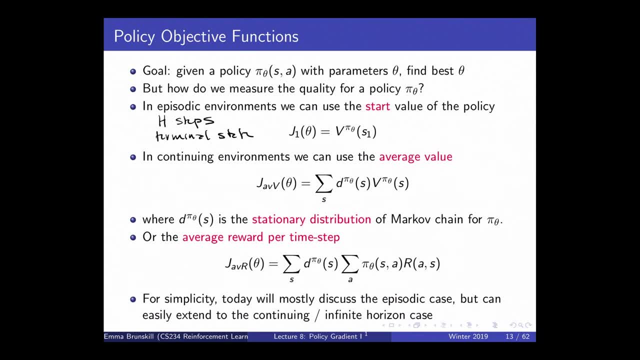 And then we can just consider: what is the expected value, what- or what is the value, what is the expected discounted sum of rewards we get from a start state Or a distribution of start states, And then what we wanna do is find the parameterized policy that has the highest value. 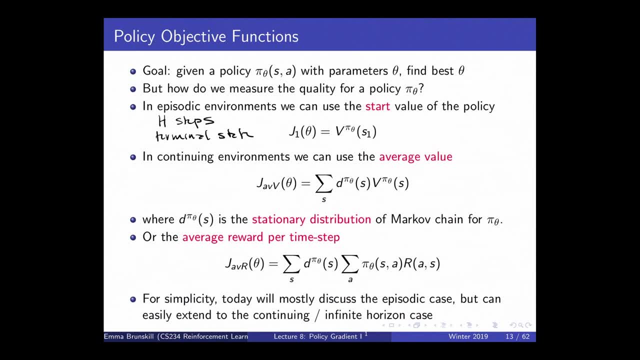 Um. another option is that if we're in a continuing environment, which means we're in the online setting, we don't act for h steps, we just act forever. there's no terminal states And we can either use the um. 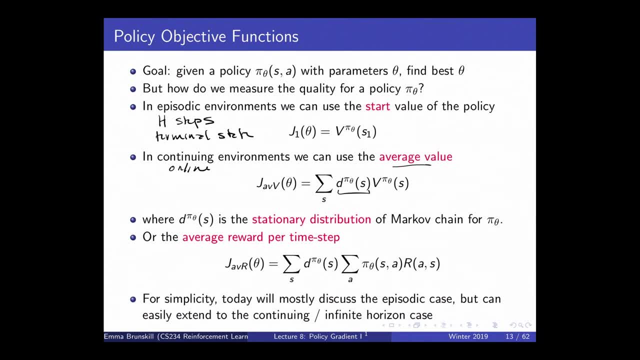 average value where we average over the distribution of states. So this is um like what we saw before thinking about the distribution, the stationary distribution over the Markov chain, That is induced by a particular policy, Because we talked about before about the fact that if you fix the policy, 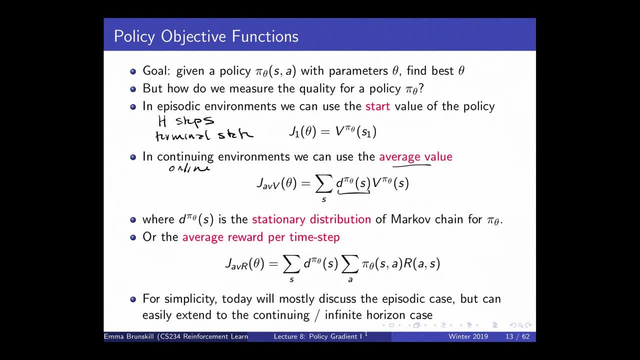 um then basically, uh, you get in a Markov reward process. You can also just think of the distribution of states you get as a Markov chain. So, um, if we're acting forever, we're gonna say sort of on average. 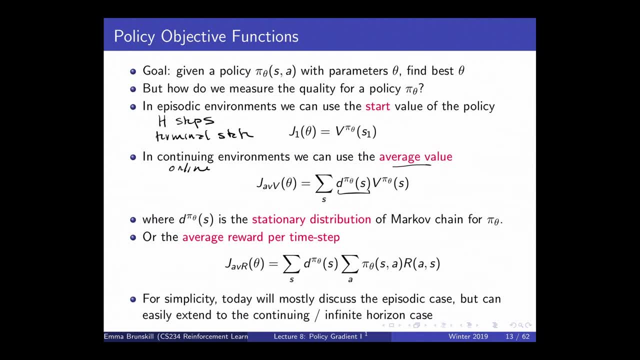 what is the value of the states that we reach under that stationary distribution? Um, and another way to do it is also to say we just look at sort of the average reward per time. step Now for simplicity. there we're gonna focus almost. 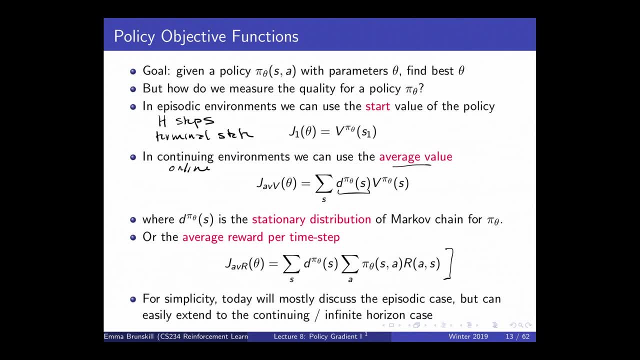 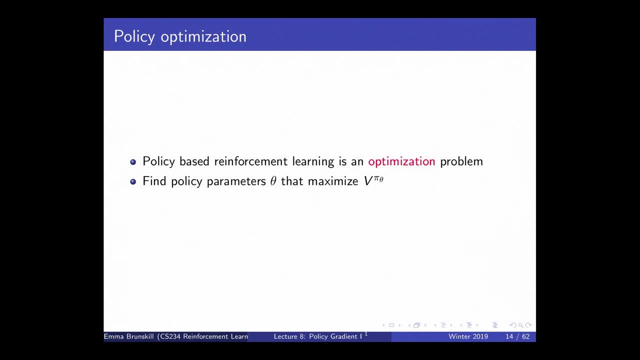 exclusively on the episodic setting, but we can think about similar techniques for these other forms of settings. So, as before um, this is an optimization problem, similar to what we saw in the value function approximation case, uh for linear value functions and using deep neural networks. 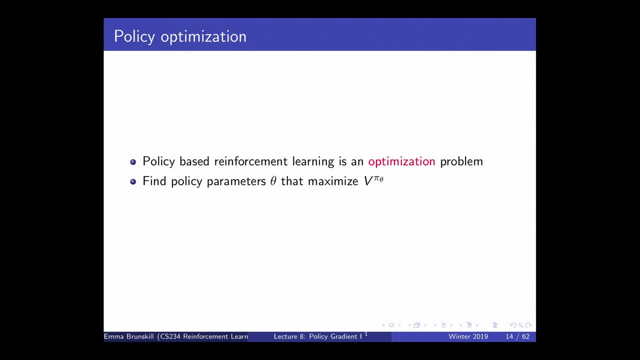 Um, we're gonna wanna be doing optimization, uh, which means that we need to do some sort of optimization tool to try to search for the best data. So one option is to do gradient-free optimization. We don't tend to do this very much in policy search methods. 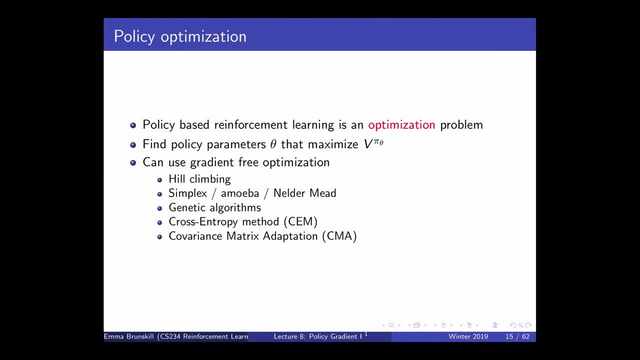 um. but there are lots of different methods that are gradient-free optimization, just for us to find whatever parameters maximize this- v, pi, theta, Um- and just to connect this, just like what we saw for Q functions. now we have theta, which is specifying a policy. 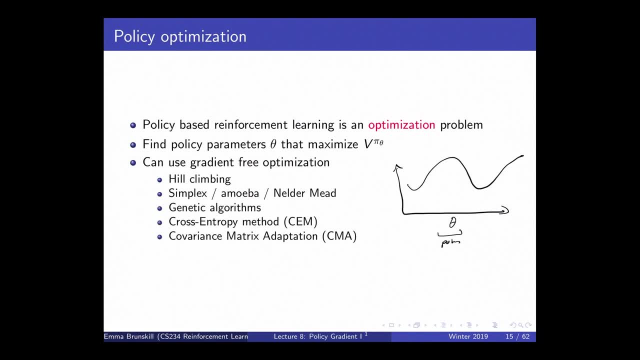 and it maybe have some interesting landscape, and then we wanna be able to find where's the max. So we're really trying to find the max of a function as we go along, Okay, As efficiently as we can, And there are lots of methods for doing that that don't rely on the function being differentiable. 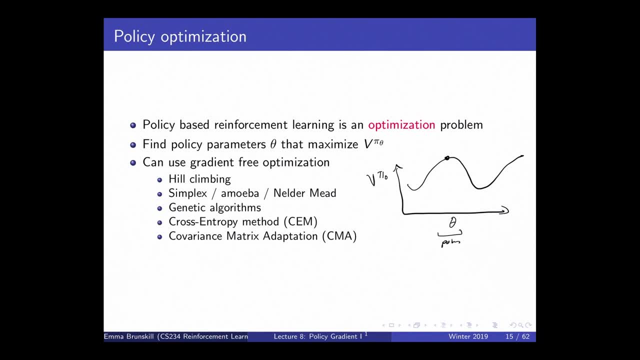 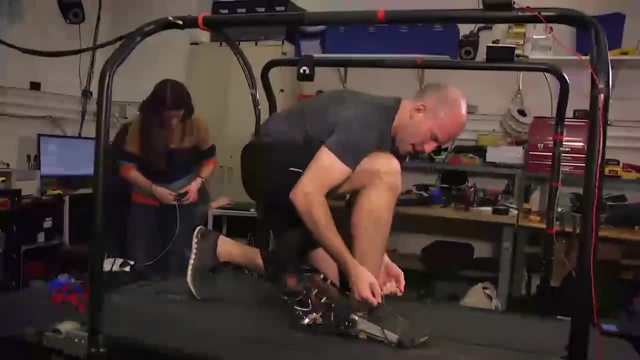 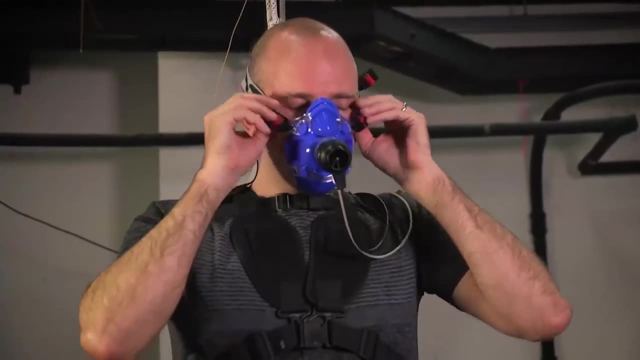 Um, and these actually can be very good in some cases. Um, so this is some nice work done by a colleague of mine in. We have developed a method for automatically identifying the exoskeleton assistance patterns that minimize metabolic energy cost for individual humans during walking. 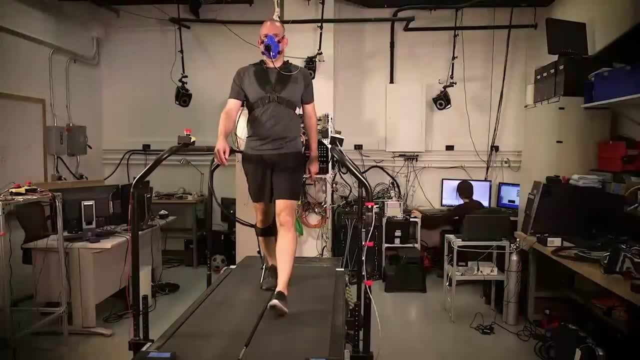 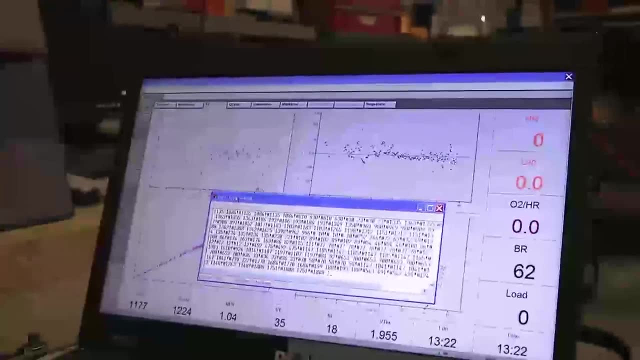 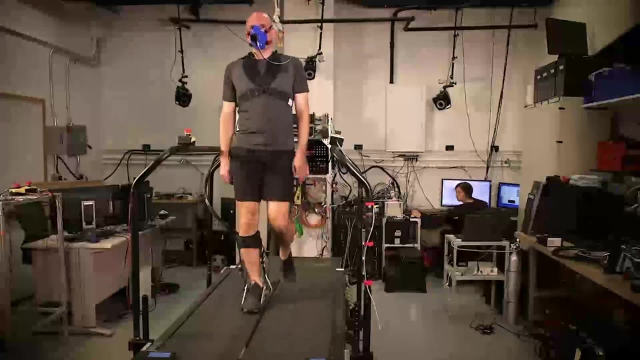 During optimization, the user first experiences one control law. while respiratory measurements are taken, Steady state energy cost is estimated by fitting a first-order dynamical model to two minutes of transient data. The control law is then changed and metabolic rate is estimated again. 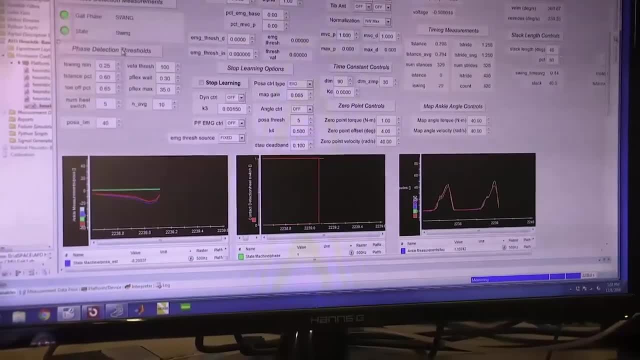 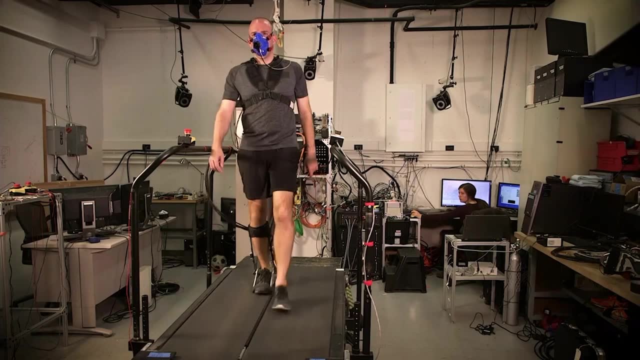 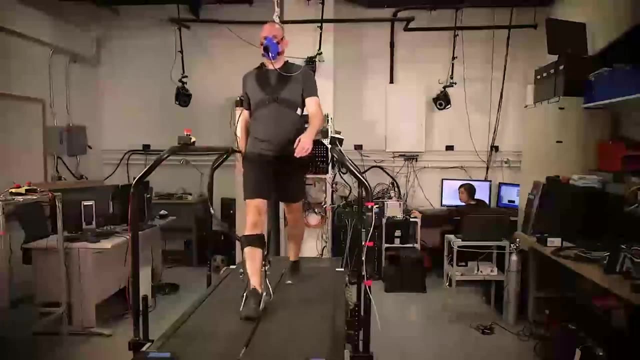 This process is repeated for a prescribed number of control laws, forming one generation. Alright, We can use a co-variance matrix. adaptation evolution strategy is then used to create the next generation. The mean of each generation represents the best estimate of the optimal control parameter values. 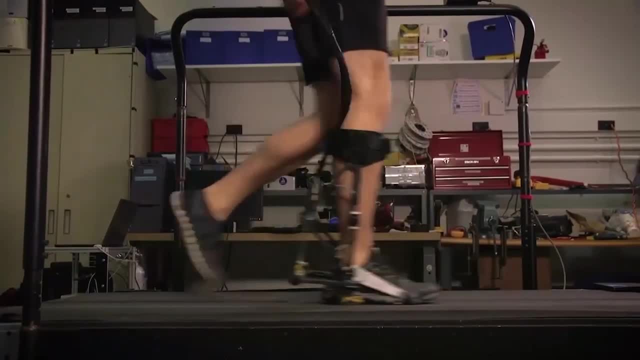 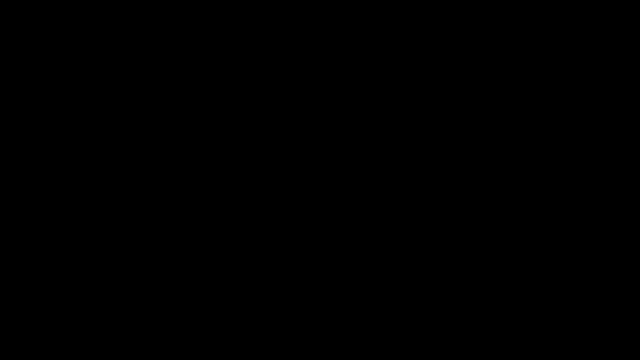 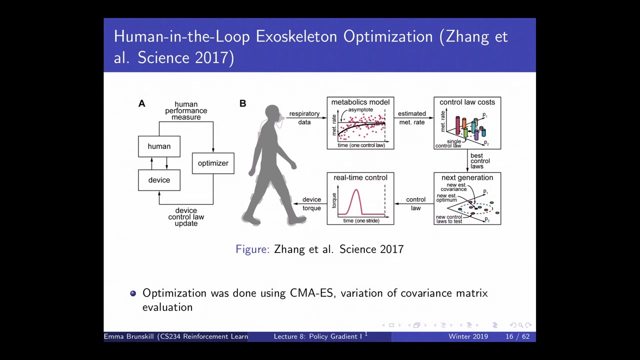 After about an hour of optimization, energy cost was reduced by an average of 24%, compared to no assistance. So this is work that's done by my colleague, uh, Steve Collins, um, who's over in mechanical engineering, and we've been collaborating. 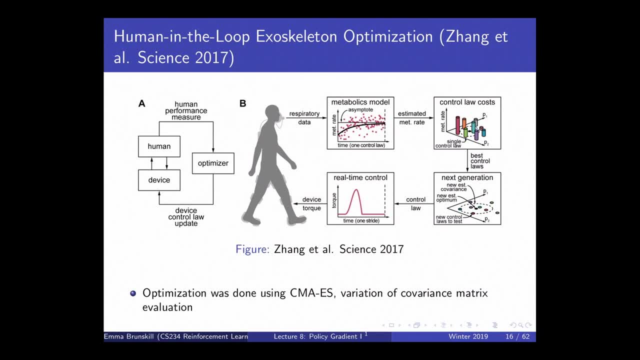 some on whether you can train people to do this better. So the idea in this case is that there's lots of instances for which you'd like to use exoskeletons. A lot of people have strokes, a lot of people have mobility problems and, of course, there's a lot of veterans that lose a limb. 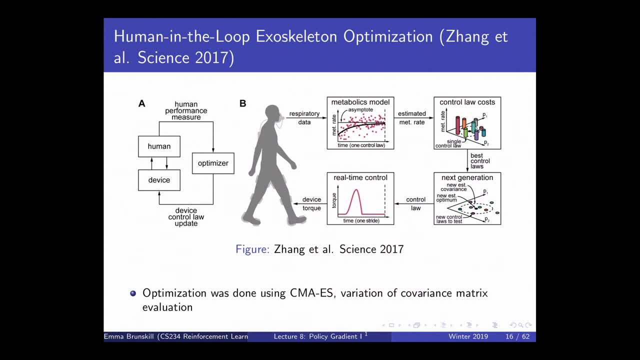 And in these cases one of the challenges has been is: how do you sort of figure out what are the parameters of these exoskeletons in order to provide support for people walking- And generally it varies on physiology and for many different people they're going to need different types. 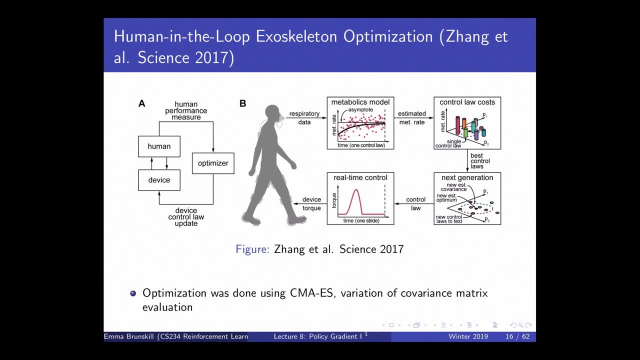 of parameters, But you want to do this really quickly, So you want to be able to figure out very fast for each individual what is the right control parameters in order to help them get the most assistance as they walk, And so Steve's labs treated this as sort of a policy search problem. 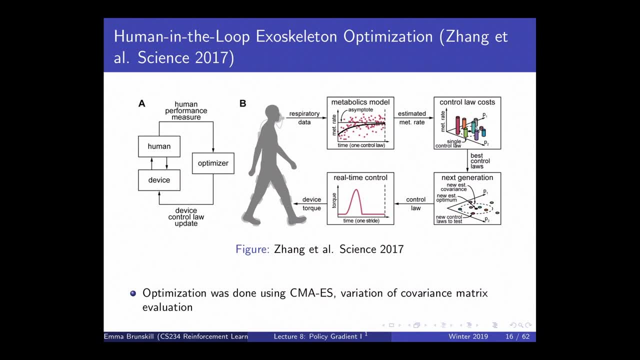 where what you're doing is you're having somebody wear their device, you're trying some control laws that are providing a particular form of support in terms of their exoskeleton. you're measuring their sort of metabolic efficiency, Which is: how do you, you know, how hard are they breathing, how hard are they having to work? compared? 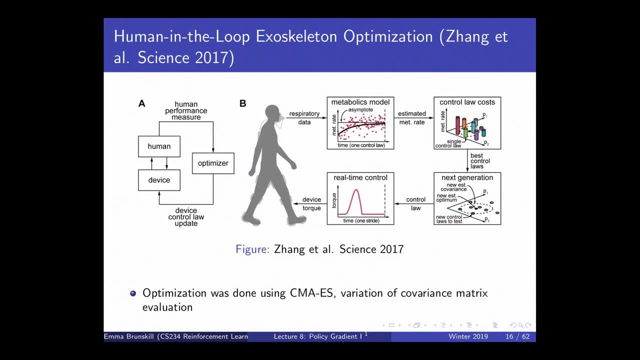 to if they weren't wearing this or under different control laws, And then you can use this information to figure out what's the next set of control laws you use, and do this all in a closed loop fashion as quickly as possible. Now, one of the reasons I bring this up is both because it was incredibly. 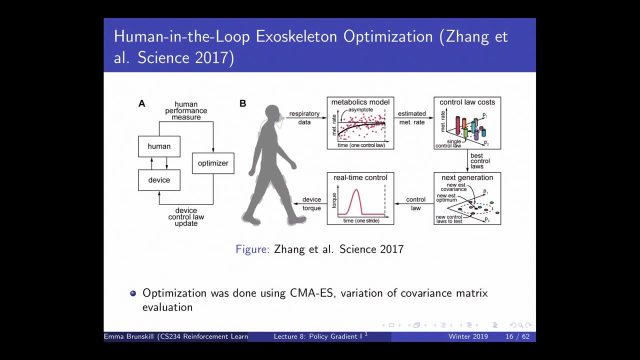 effective. it's a really nice science paper that illustrates how this could be much more effective than previous techniques. And second, because it was using CMAES, which is a gradient pre-approach, Even though most of what we're going to discuss today in class is all with gradient-based methods. 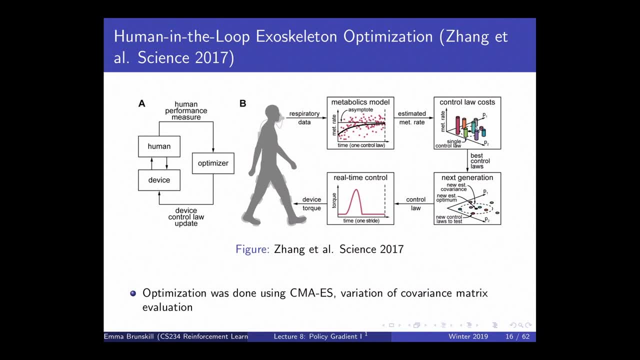 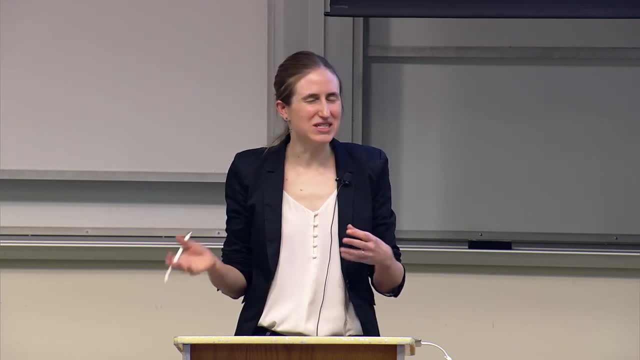 there's some really nice examples of not using gradient-based methods also to do policy search for lots of other types of applications. So I think it's useful to sort of know in your toolbox that one doesn't have to be constrained to gradient-based methods. And one of the really nice things: 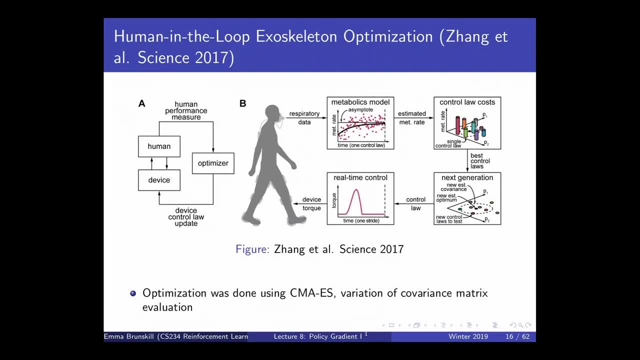 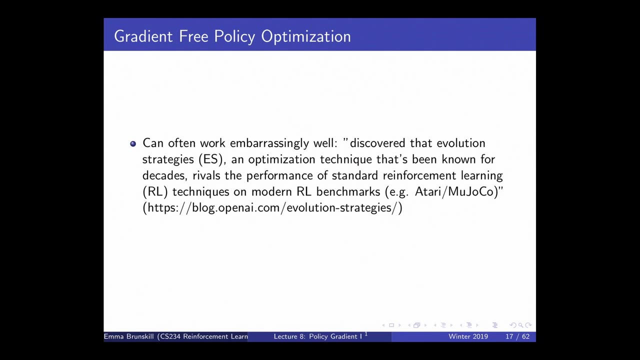 about things like CMAES is that they're guaranteed to get towards a to a global optima. So in some cases you might really want to be guaranteed that you're doing that, because it's a high-stakes situation And in general it sort of is has been noticed repeatedly recently that sometimes these sort of approaches 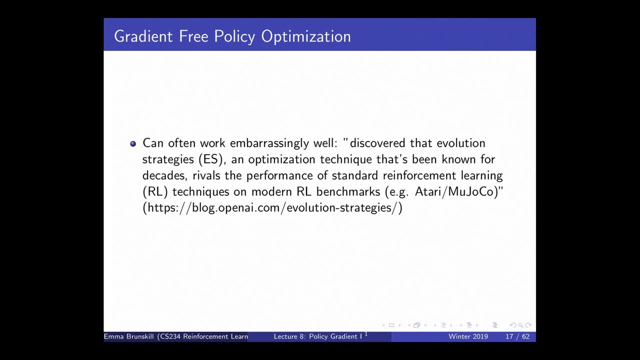 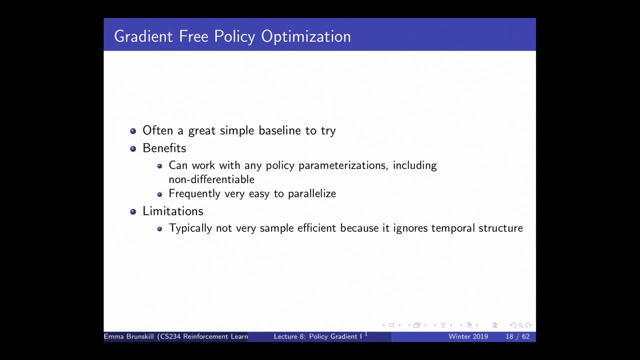 do work kind of embarrassingly well. They tend to be in some ways sort of a brute force, a smart brute force way that often can be very effective. So they're good to consider in terms of the applications you look at. But you know, despite this, even though they can be really good, and sometimes they're very, very helpful, 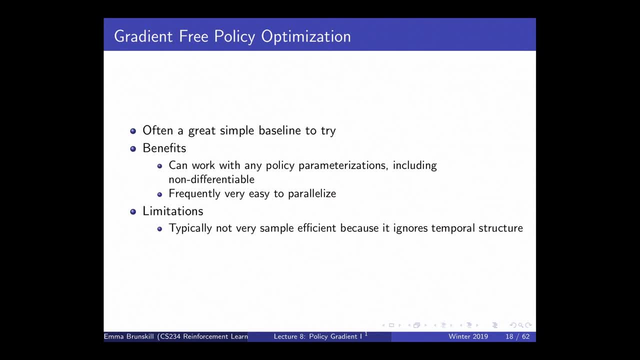 for parallelization. they're generally not very successful, And so you know, I think it's important to keep in mind that you're looking at a domain that's very sample efficient, And so, depending on the domain that you're looking at and what sort of structure you have, often it's useful to go to a gradient-based method. 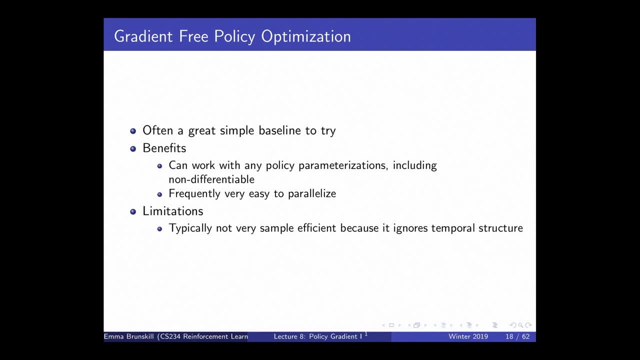 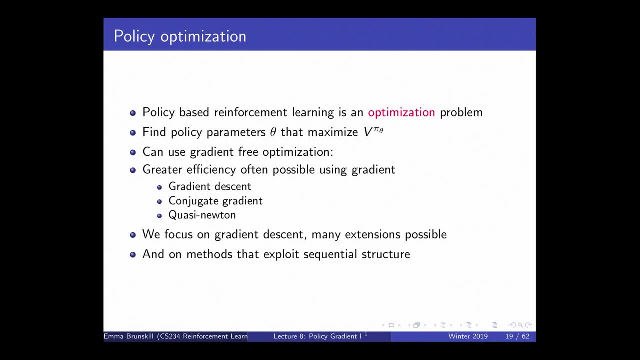 particularly if you might be satisfied with the local solution at the end, Sort of locally optimal. So what we're going to talk about mostly today, just like what we did for value, like value-based methods, is gradient descent and gradient-based methods And other methods that try to exploit the sequential structure. 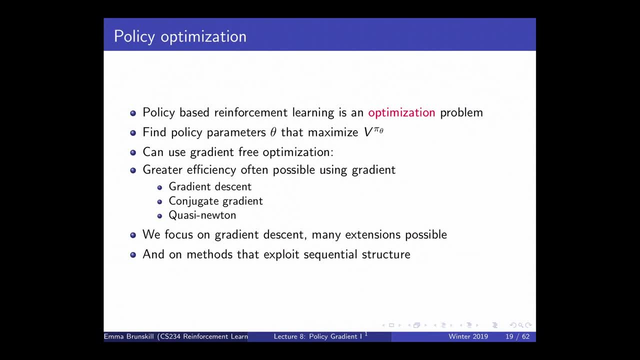 of decision-making problems. So CMAES doesn't know anything about gradient descent, It doesn't know anything about the fact that this- the world might be an MDP or any sort of sequential stochastic process, And we're going to focus on ones that sort of leverage, the structure of 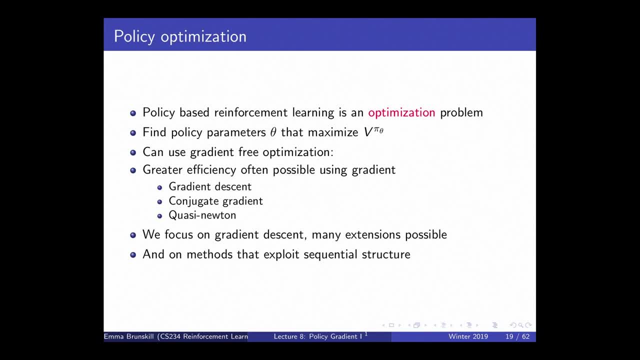 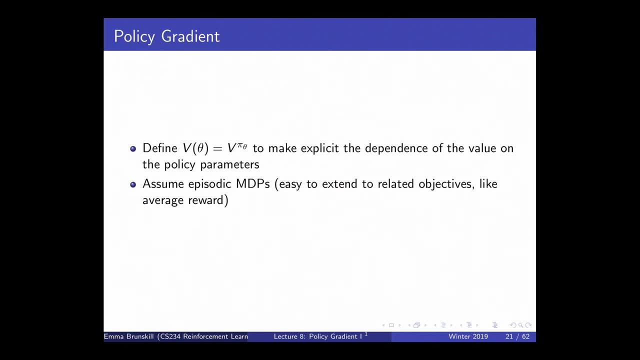 the Markov decision process and the decision process itself. So let's talk about policy gradient methods. We're again just sort of define things in terms of theta, so that we're explicit about the parameter, And we're going to focus on episodic MDPs. 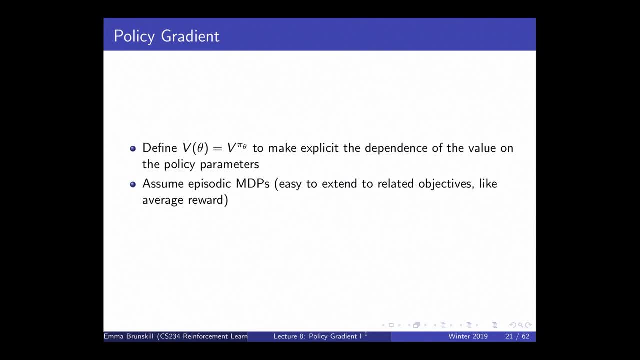 which means that we're going to run our policy for a certain number of time steps until we reach a terminal state or for certain you know, maybe eight steps. We're going to get some reward during that time period and then we're going to reset. 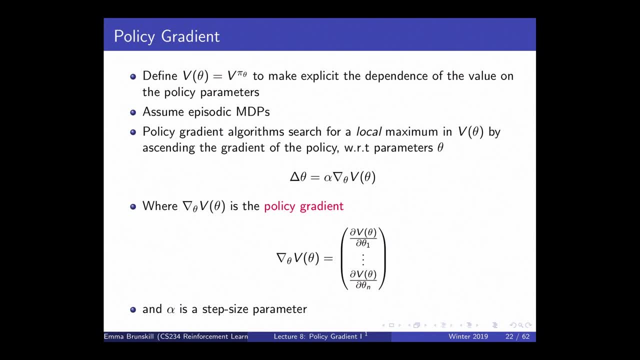 So we're going to be looking for a local maximum and we're going to be taking the gradient with respect to the parameters that define the policy And then use some small learning rate. So just this is- this should look very similar, Very similar to the- similar to Q and V based. 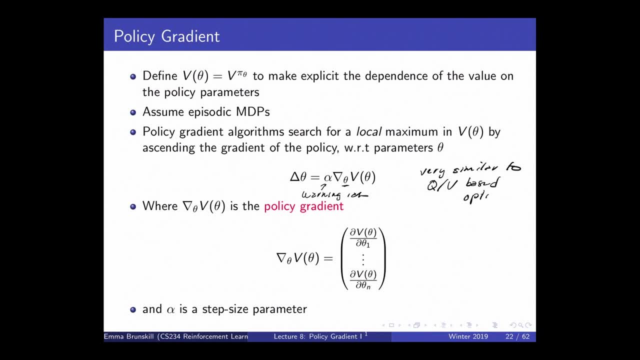 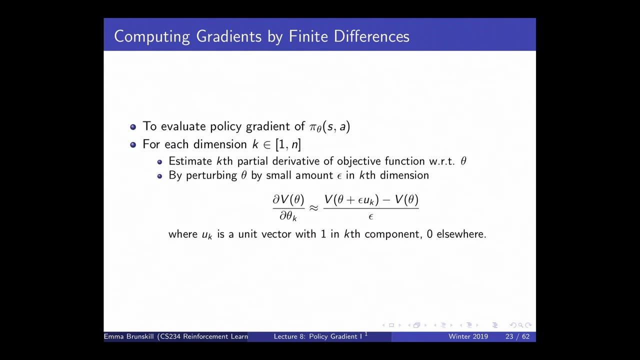 And the main difference here is that, instead of taking the derivative with respect to parameters that define our Q function, we're taking them with respect to the parameters that define our policy. So the simplest thing to do here is to do finite differences. So, for each of your policy parameters. 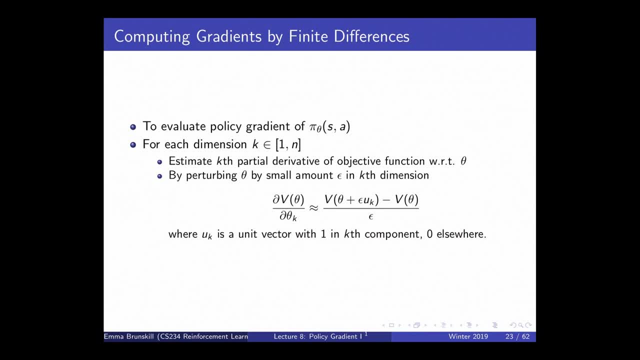 you just perturb it a little bit, And if you do that for every single one of the dimensions that define your policy parameters, then you're going to get an estimate of the gradient. You're just doing sort of a finite differences estimate of the gradient. 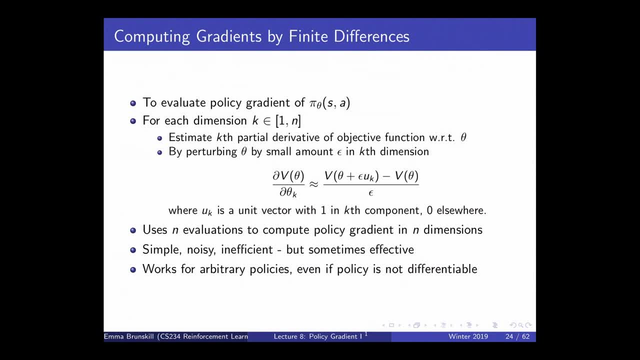 And you can use a certain number of evaluations for doing this in each of the cases. So you can- let's say you have this k-dimensional set of parameters that define your policy. You try changing one of them a little bit, you repeat it, you get a bunch of samples for that new policy. 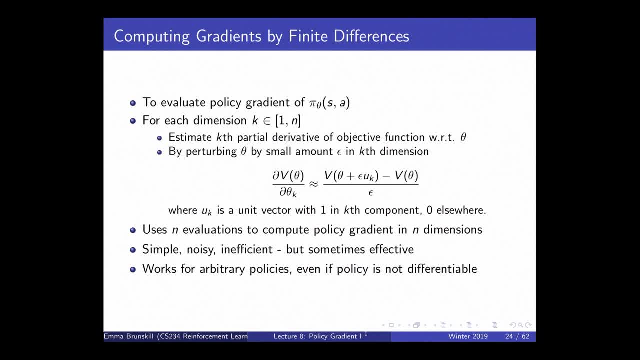 Um, you do that for every single one of the dimensions that define your policy. You do that for all of the different dimensions and now you have an approximation of the gradient. It's very simple. It's quite noisy, Um, it's not particularly efficient. 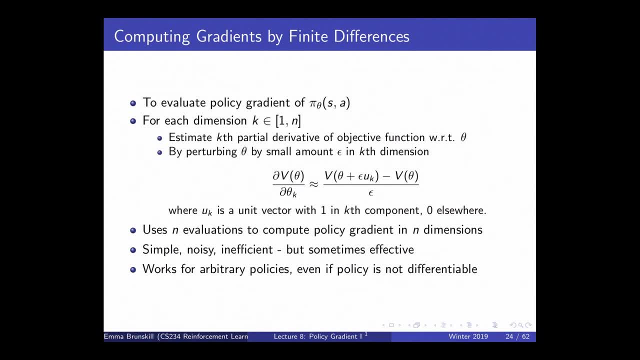 but can sometimes be effective. Um, and it was one of the earlier demonstrations of how policy gradient methods could be very useful in an RL context. Um, and the nice thing is that the policy itself doesn't have to be differentiable, because we're just doing sort of a finite difference: approximation of the gradient. 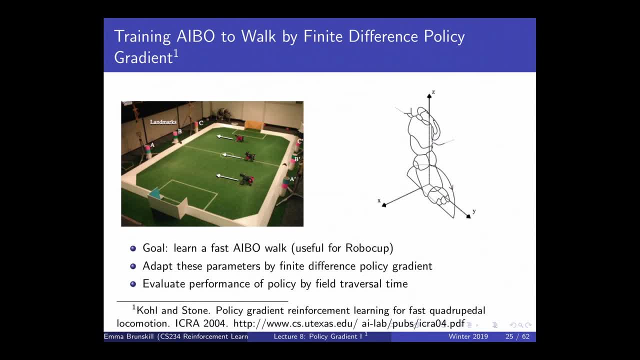 So, um, what are the first examples that I say- um I think of when I think of sort of how policy, uh granite methods or how policy search methods can be really effective, is Peter Stone's work, um on doing uh RoboCup. 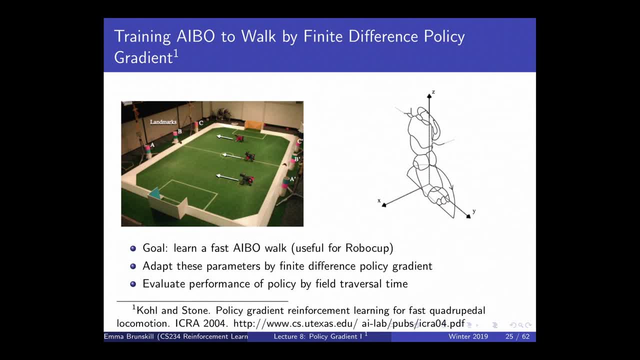 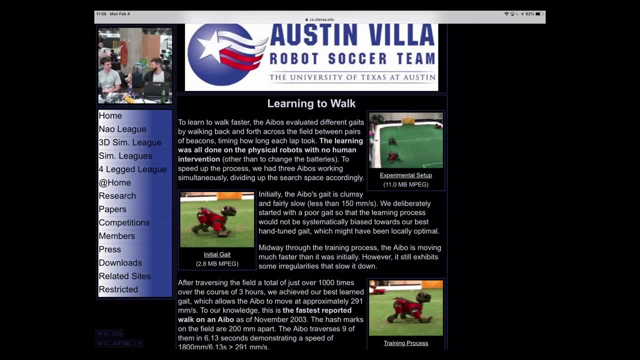 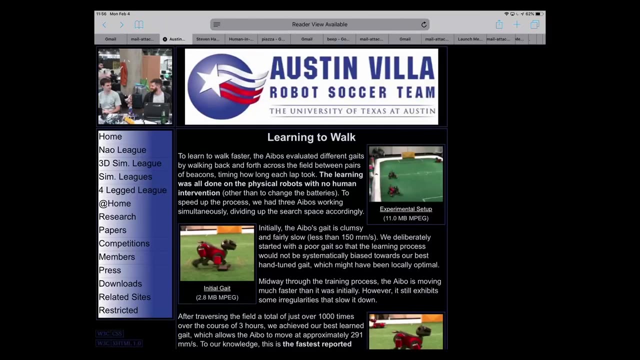 And who here has ever seen like RoboCup? Okay, a few people, but not everybody. So let's see if we can get up like a short demonstration of like what these robots look like. So let's, ah, okay. 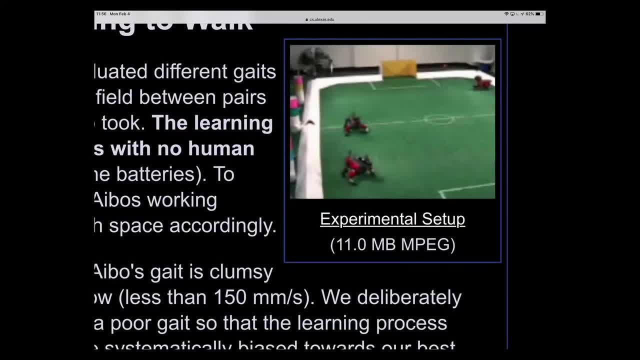 So you probably can't see it. We won't do that right now, Um, but essentially what you have is there's a bunch of different leagues of RoboCup. One of the goals has been that, um, I think by 2050, the goal is that we're going to have 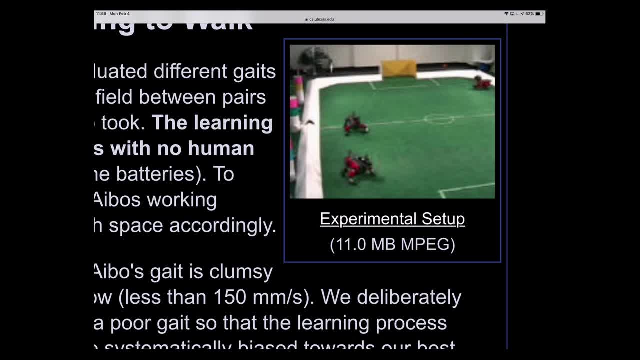 uh, a robotic soccer, um team that is going to be able to defeat, like able to, you know, um win the the World Cup? Um. so that's been one of the driving goals of the sort of the RoboCup initiative. 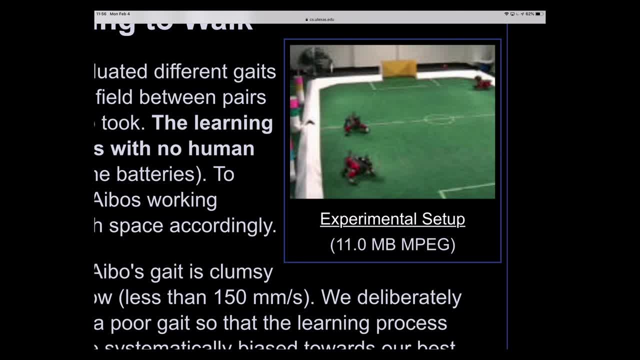 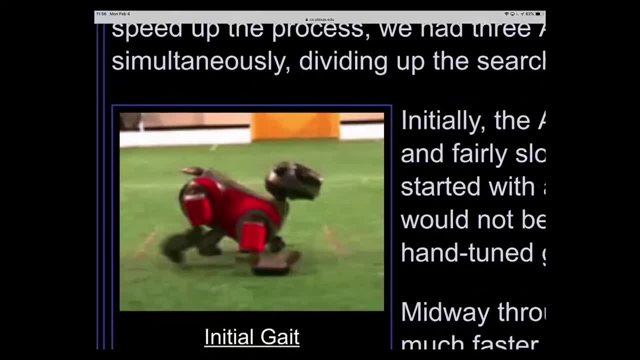 Um, and there's a lot of different uh leagues within this, and one of them is these sort of quadruped robots, um, which try to score goals against each other, And one of the key challenges for this is that they look kind of like that. 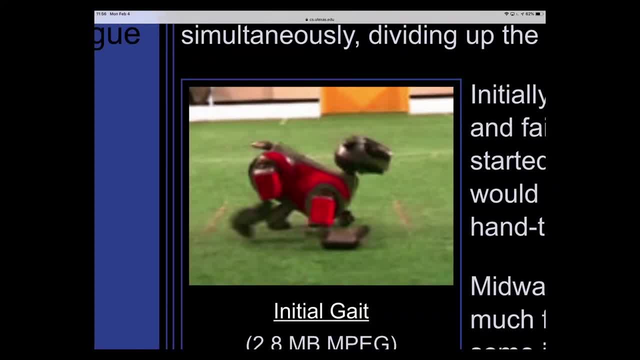 Um and you have to figure out the gait for walking Um and you want them to be able to walk quickly, but you don't want them to fall over Um, and so just simply that question of like, how do you optimize the gait? is an important question in order to win. 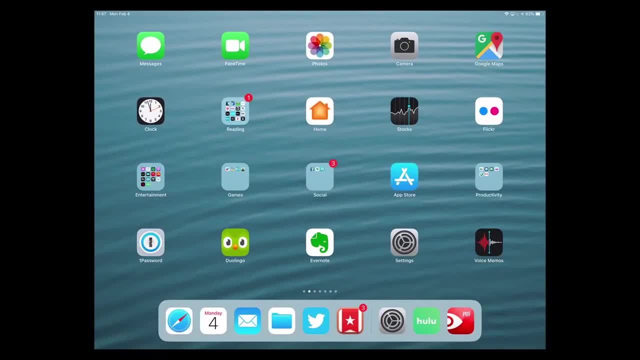 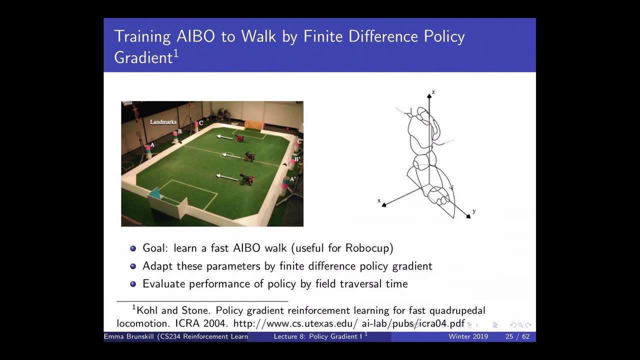 because you need your robots to move fast on the field. So Peter Stone has been a leading person in in RoboCup for a long time. Um, and their goal was simply to learn a fast way for these eyeballs to walk um. 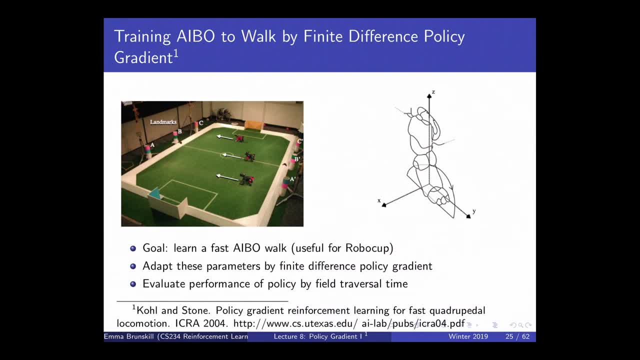 and to do it by, uh, real experience. um, and data is really important here, because it's expensive. Um, like you have these robots walking back and forth and you want them to very quickly optimize their gait, um, and you don't want to have to keep changing batteries and things like that. 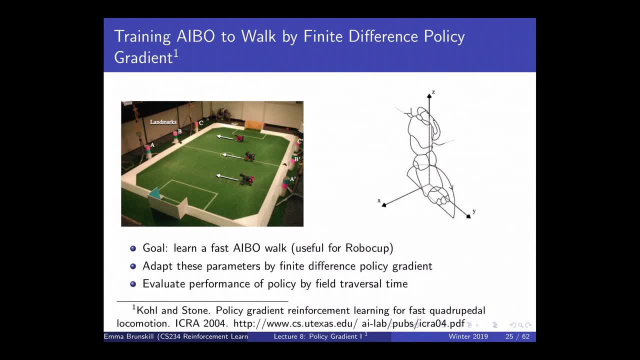 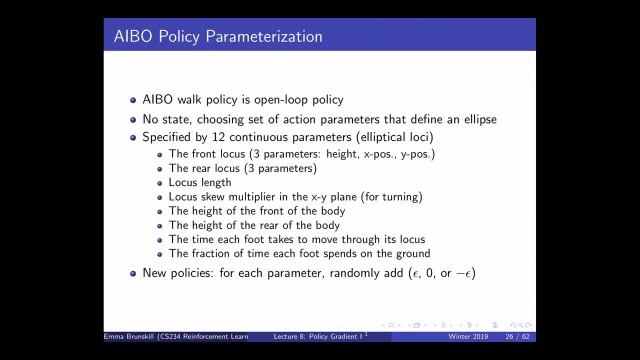 So you really want to do this with very little amounts of data. So what they thought of doing in this case is sort of to do a parameterized policy and try to optimize those pro-. policies. So this is where significant domain knowledge came in. 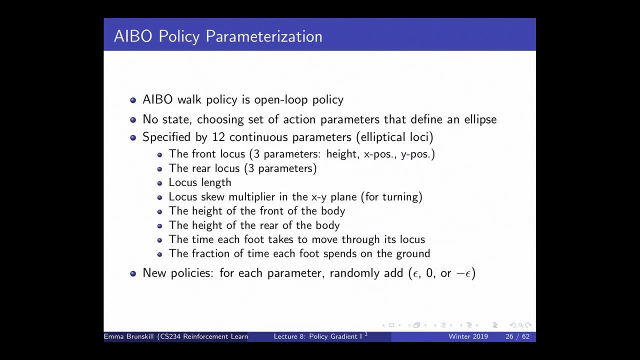 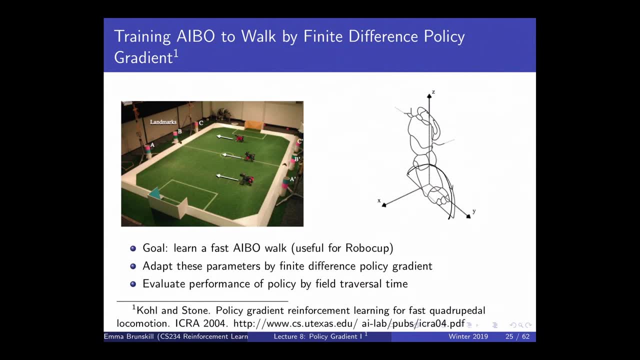 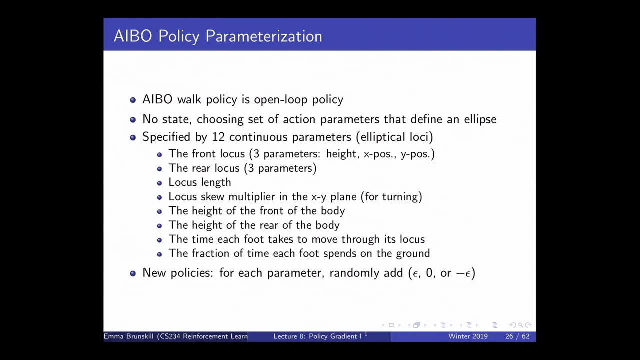 and this is a way to inject domain knowledge. So they um specified it by this sort of continuous ellipse of how gait works for um, this small robot, And so they parameterize it by these 12 continuous parameters, And this completely defines the space of possible policies. you could learn. 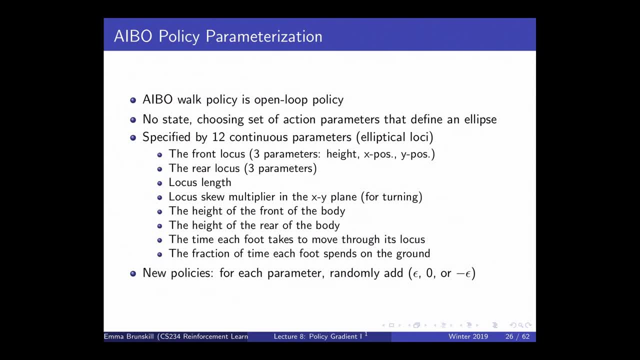 This might not be optimal. Peter Stone and his group have a huge amount of experience on doing RoboCup um at the time they were doing this paper, And so they really had a lot of knowledge they could inject in here And in some ways it's a way to provide sort of this hierarchical structure. 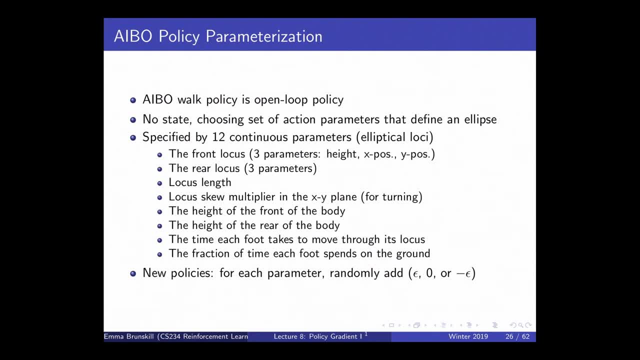 about what sort of policies might be good, And then what they did is they just did this method of finite differencing in order to try to optimize for all of these parameters. So one of the important things here, um, is that all of their policy evaluations were gonna be done on actual, real robots. 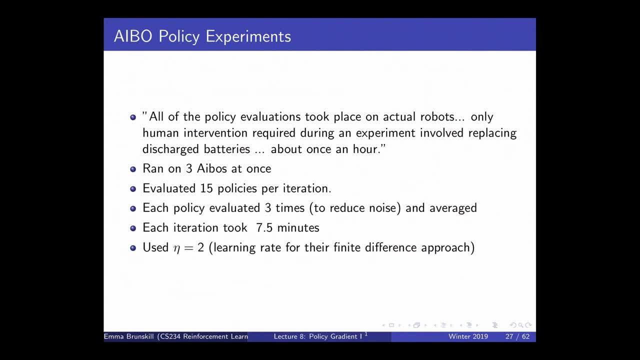 Um, and they just wanted to have people inter- interfering every once in a while in order to replace batteries, which took- happened about once an hour, Um, and so they did it on three IBOs, very small amount of hardware, Um, they did about 15 policies per iteration and they evaluated each policy. 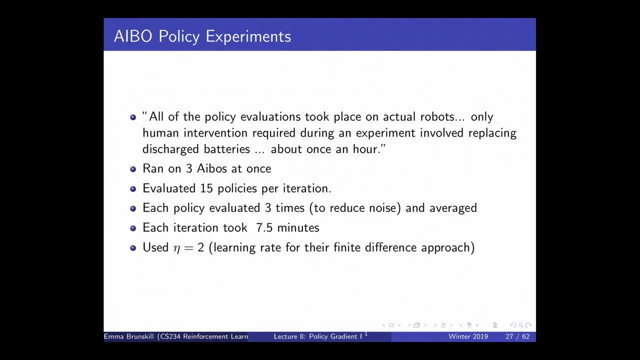 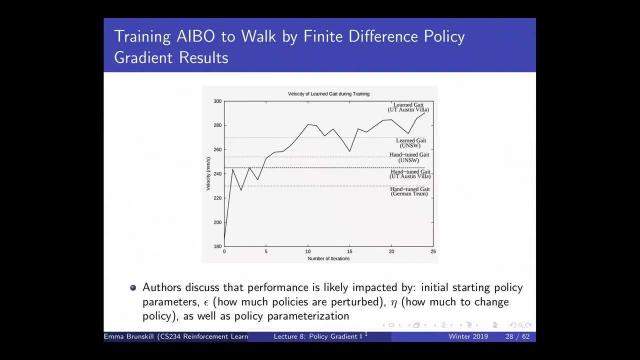 Three times, So that's not very many. That can be a very noisy signal, Um, and each iteration took about 7.5 minutes, So, and then they had to pick some learning rate. And so what do we see in this case? 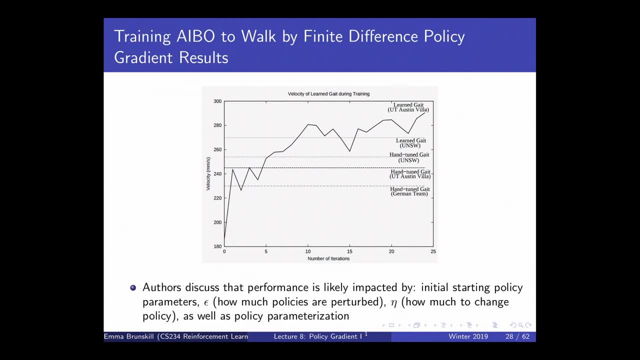 Well, we see that in terms of the number of iterations that they have versus how quickly they're. of course, you have to define your optimization criteria. In this case, they're looking at speed of stable walking, Um, and a lot of people had been trying to figure out how to do these using hand-tuning before. 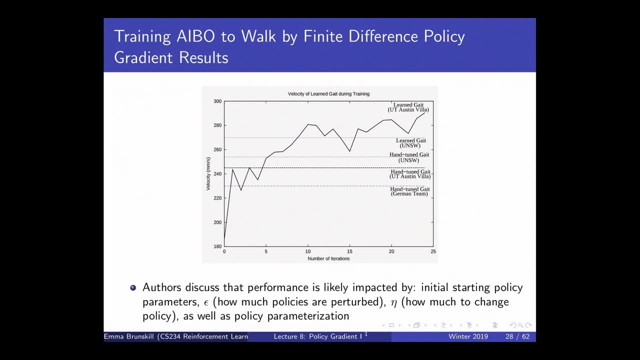 Um, uh, including- so they're- the UT Austin Villa team. um, including them. in the past, people have found different ways to sort of hand-tune. Um, I don't know if some of you are using supervised learning, et cetera. 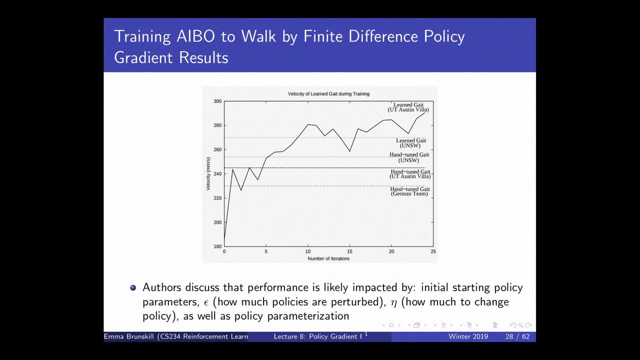 And you can see, as they do, multiple iterations of trying to search for a better policy using this finite difference method that they get to faster than everything else, And this is not that many iterations. Um, so this is something that was happening over. 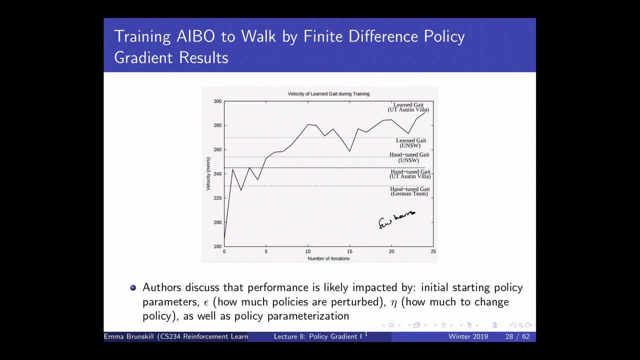 you know a few hours, So I think this is a really compelling example of how policy gradient methods could really do much better than what had happened before, and they didn't have to require enormous amount of data. That's very different than probably what you're experiencing in assignment two. 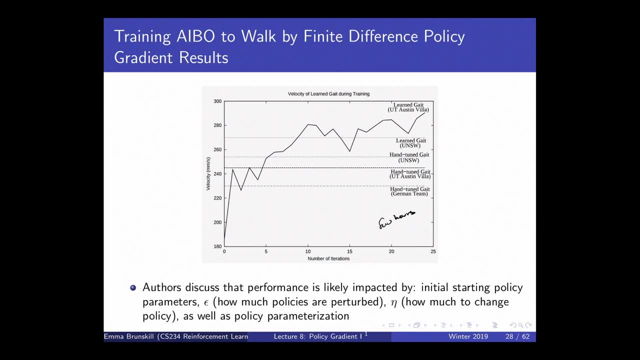 So this is no total number of iterations. Um, I think this was on the order of. let's see, like I don't know, this is on the order of, you know, tens to hundreds of policies, not millions and millions of steps. 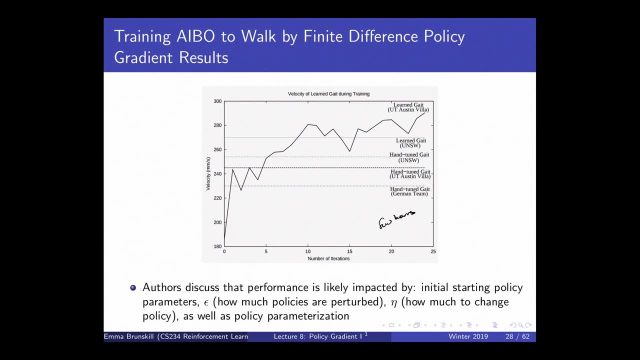 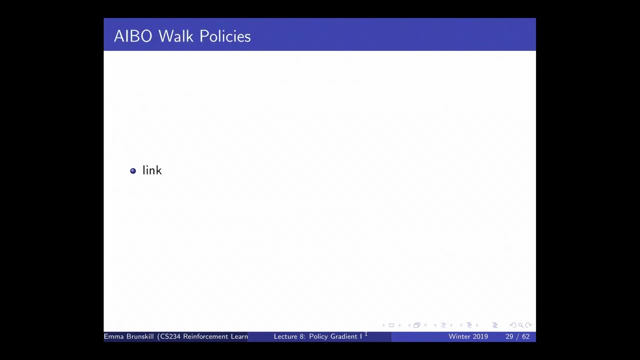 So these things can be very data efficient, but there was also a lot of information that was given. So, um, if you think about sort of like, uh, let me have a little bit on here. So in their paper they discussed sort of what was actually impacting performance in this case. 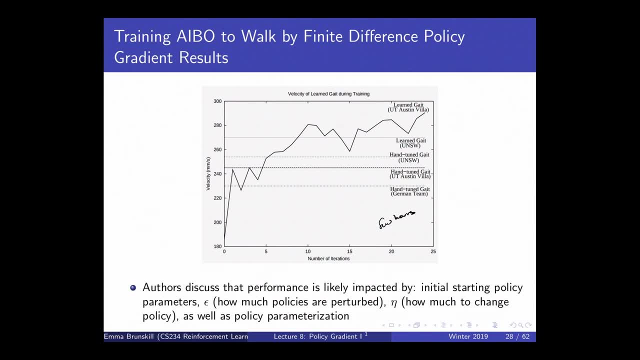 and there's a lot of things that impact performance. So, um, you know how do we start. Um, so it may have a sense what you know. why does the initial policy parameters used matter for this type of method? Yeah, 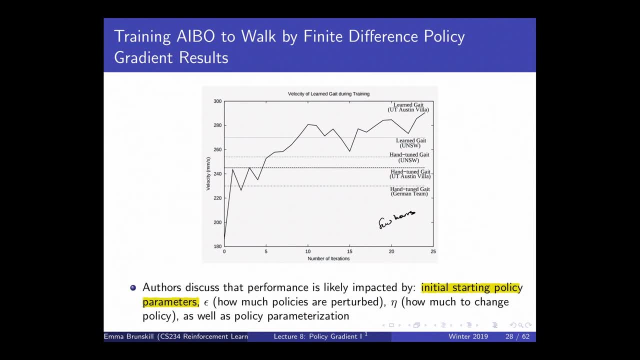 Well, because we're not guaranteed to have a global optimum, only a local optimum. So your starting point is going to affect which local optimum you are able to find Exactly. So what-? What I just said is that, um, because these methods are only guaranteed. 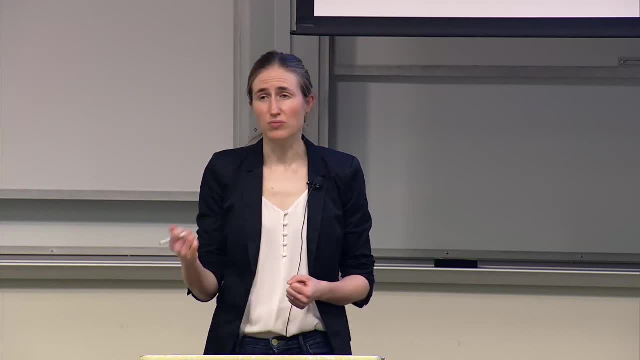 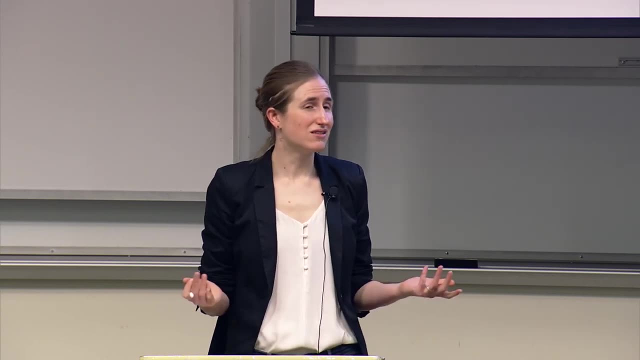 particularly, this method is only guaranteed to find a local optima, and all of the sort of policy gradient style methods are um then, wherever you start, you're going to get to the closest local optima and you have no guarantee that that's the best global optima. 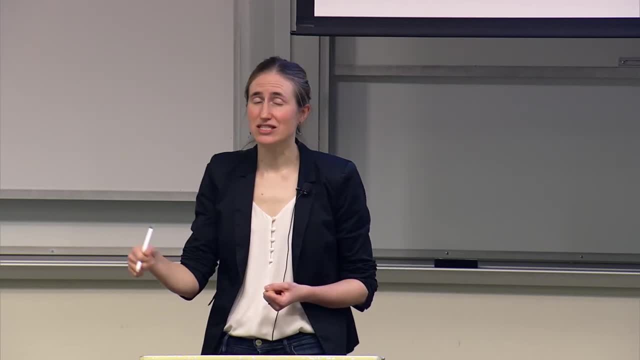 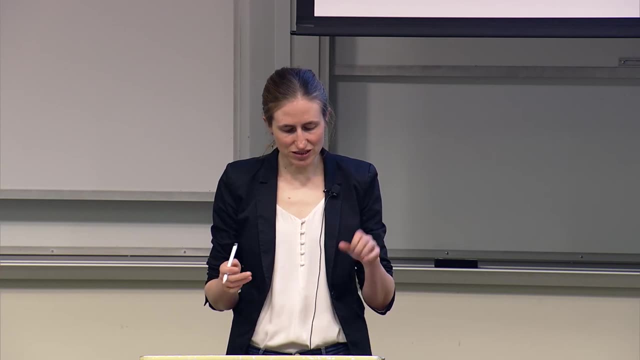 Um. so it's important to either try lots of random restarts here in this case, or to have domain knowledge, Um. another important question here is: how much are you perturbing sort of the size of your finite differences? And then I think really most critical is this policy parameterization. 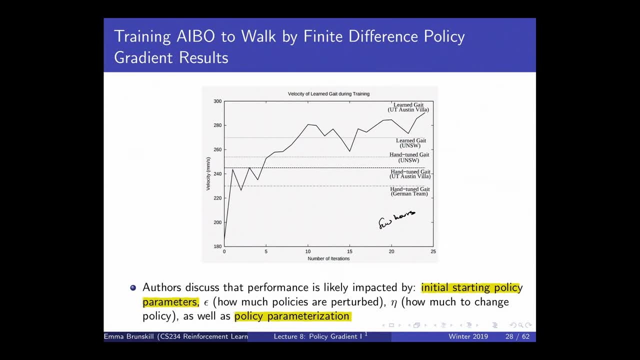 Like, just how are you writing down the space of possible policies that you can learn within? Because if that's not a good policy space, then you're just not going to learn anything. Um, yeah, On slide 26, you had uh. 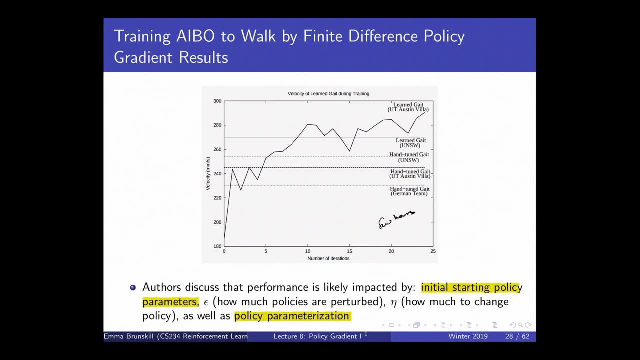 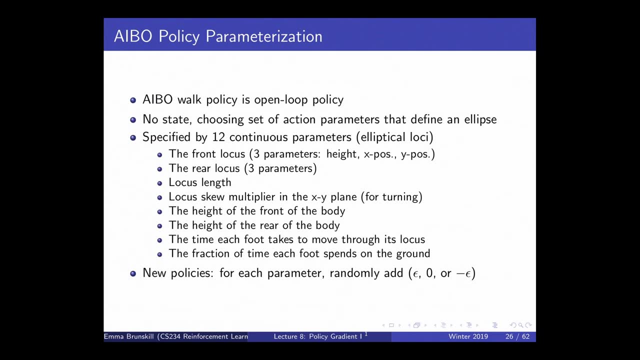 AIVO is an open loop policy. Can you expand a bit more on that? Yeah, Um, uh. so the question was about the open loop policy part. So these policies that we're learning don't have to be adaptive. An open loop policy is essentially a plan. 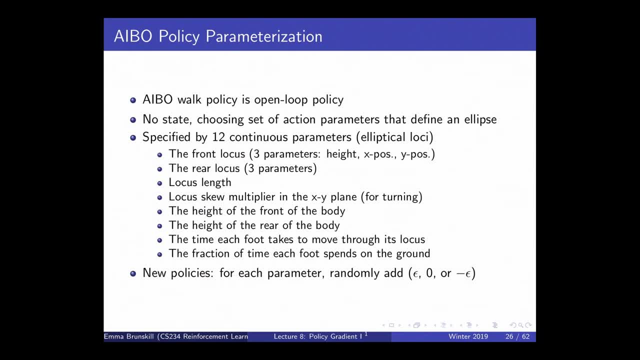 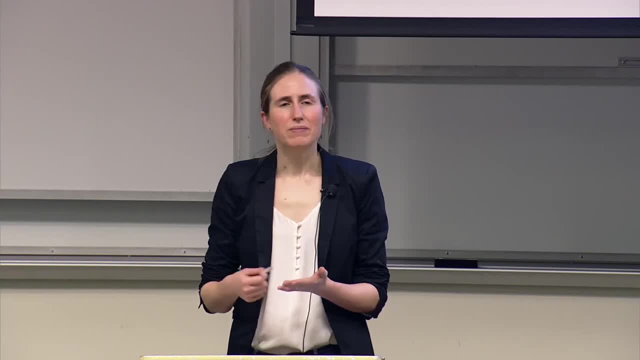 It's a sequence of actions to take, Um, regardless of any additional input that you might have. So, um, we typically have been thinking about policies as mappings from states to actions, but they can also just be a series of actions, And so, when we talk about an open loop policy, 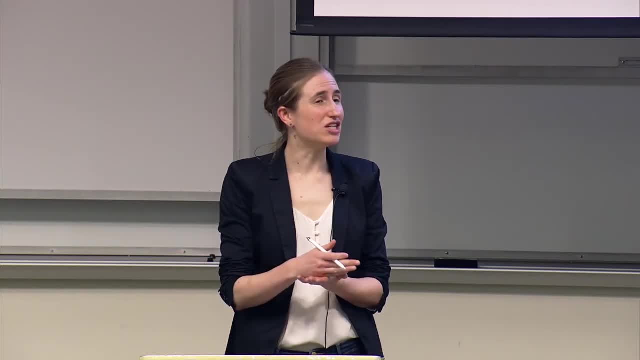 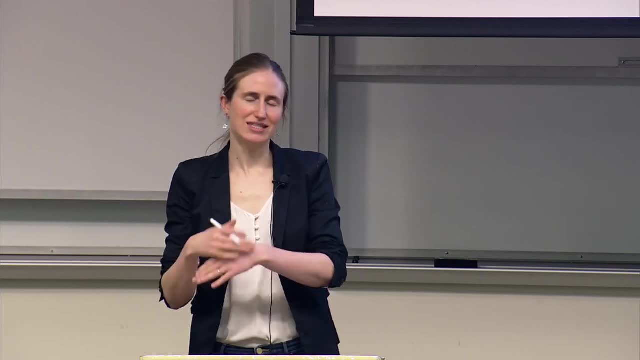 that's a non-reactive policy, because it's just a sequence of actions that, regardless of the state of the robot, you just keep going. So maybe there's a really large wind in the middle and the robot's next action is the same whether there's a lot of wind or not. 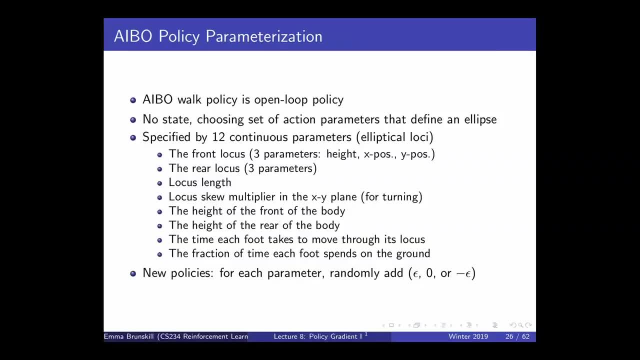 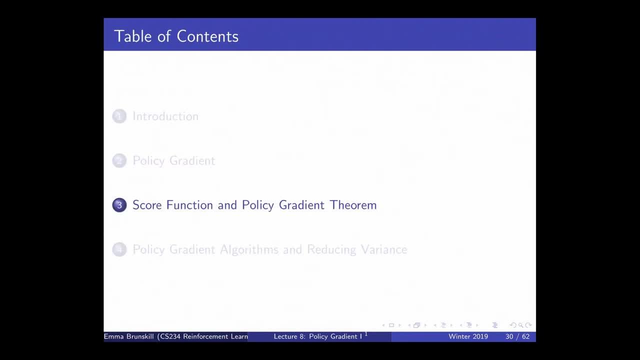 It doesn't have to be reactive. Okay So, but in general, um, you know, finite differences is a reasonable thing to try. Um, often we're gonna want to use gradient information and leverage the fact that our policy function is actually differentiable. 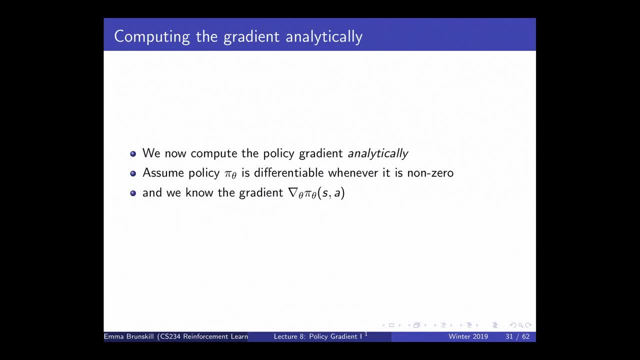 So what we're gonna do now is um compute the policy gradient analytically. Excuse me, this is most common um in most of the techniques that are used right now. Um, we're gonna assume it's differentiable wherever it's non-zero. um. 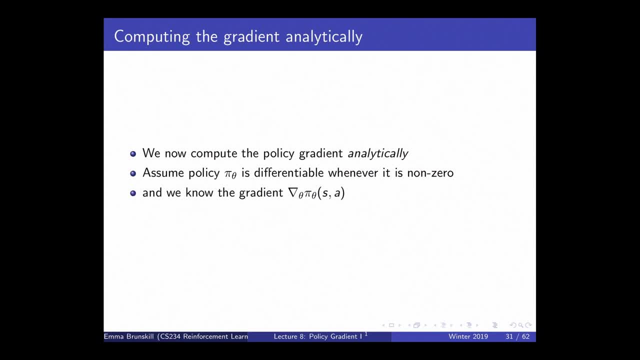 and that we can explicitly compute this. So when we say what we- when we say we know, that means that this is computable, We can compute this explicitly. And so now we're gonna be um thinking only about gradient-based methods. 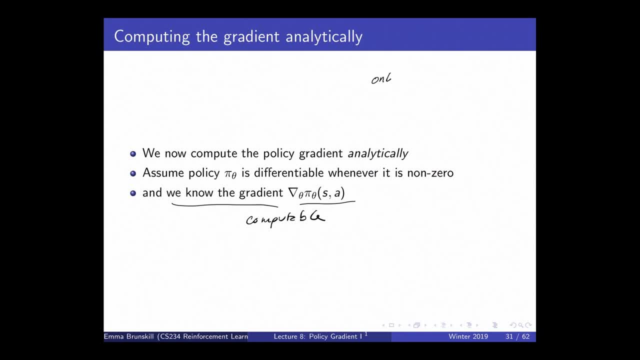 And so we're only- we're gonna only- converge to a local optima. Hopefully, hopefully we'll get to a local optima. That's the best we can hope for in this case. Okay, So we're gonna talk- people often talk about likelihood ratio policies. 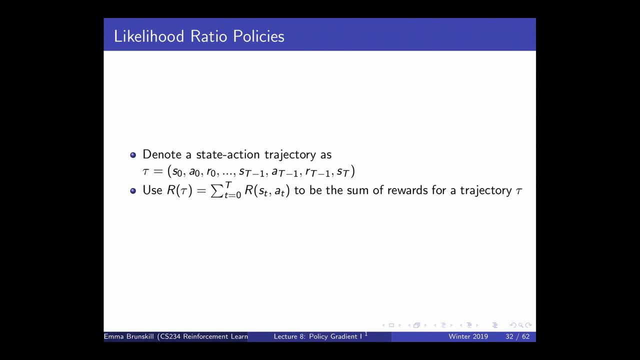 Um, and they're gonna sort of proceed as follows: So let- we're thinking about the episodic case, So we're gonna think about it as having um trajectories, So state action, reward, next state, et cetera, all the way out to some terminal state. 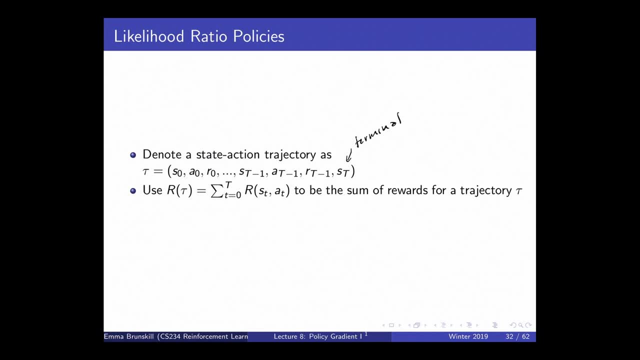 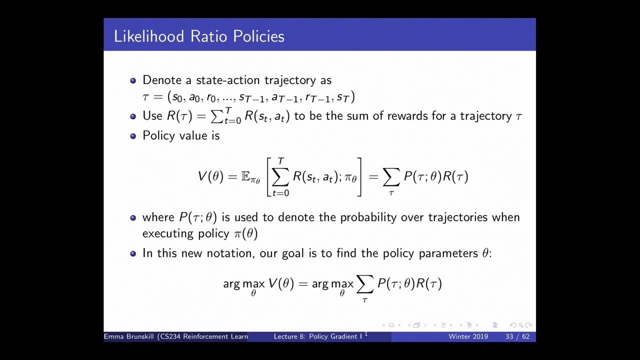 So this is where we terminate And we're gonna use R of tau to denote the sum of rewards for a trajectory. Okay, So the policy value in this case is just gonna be the expected discounted sum of rewards we get by following this policy. 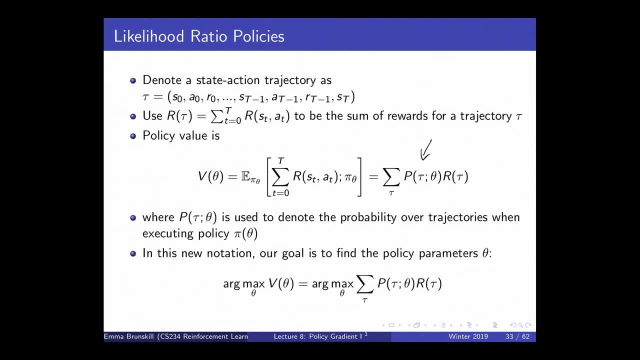 And we can represent that as the probability that we observed a particular trajectory times the reward of that trajectory. So it just says, given under this policy, what are the you know what's the probability of seeing any trajectory, And then what would be the reward of that trajectory? 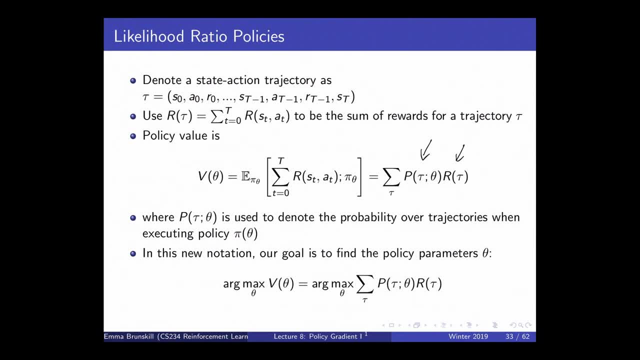 Because the reward is just a deterministic function of the trajectory. Once you know the state, action, rewards, et cetera, then your reward is, um, just the sum of all of those. And so now, in this particular notation, what our goal will be is to find policy parameters, theta. 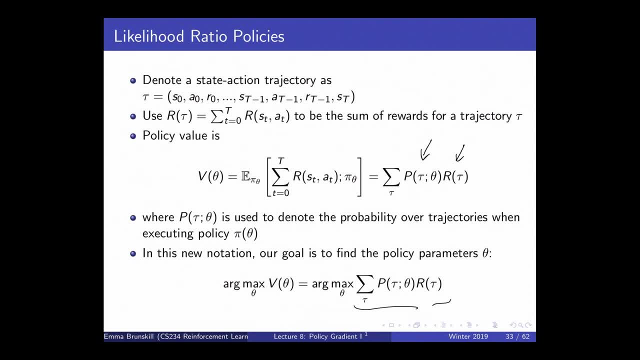 which um are the argmax of this And- and the reason we've sort of- what- what have we changed here? Um, the change now been- has been the fact that we're gonna focus on here. So notice now that the policy parameters only appear in terms of. 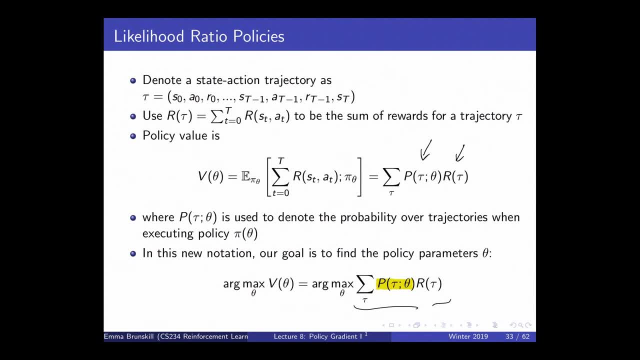 the distribution of trajectories that we might encounter under this policy. And this is again a little bit similar to what we talked about for imitation learning before, Where in imitation learning we talked a lot about distributions of states and distributions of states and actions and trying to find a policy that 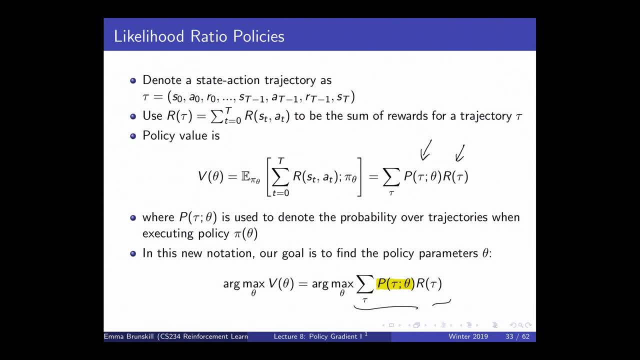 would match the same state action distribution as what was demonstrated by an expert Um. today we're not gonna talk as much about sort of state action distributions, but we are talking about sort of distributions of trajectories that we could encounter under our particular policy. 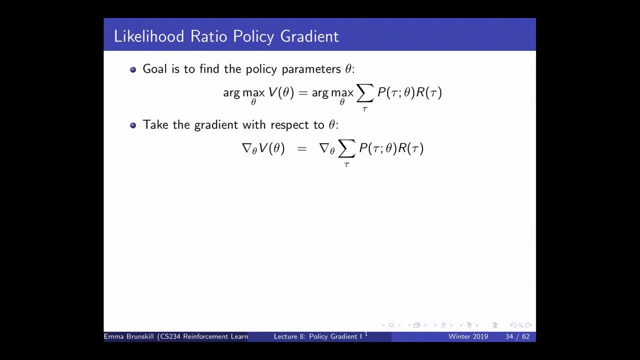 So. So what's the gradient of this? Um, so we wanna take the gradient of this function with respect to Theta, So we're gonna go for this as follows: We're gonna rewrite what is the probability of a trajectory under Theta. 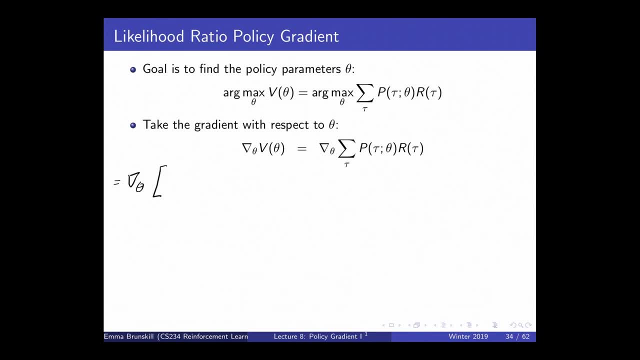 So I'm over Tau And we're gonna do probability of Tau Theta times, uh, or at first actually, I'll move it in here And then what we're gonna do is- I'm just gonna make sure I get the notation the same. 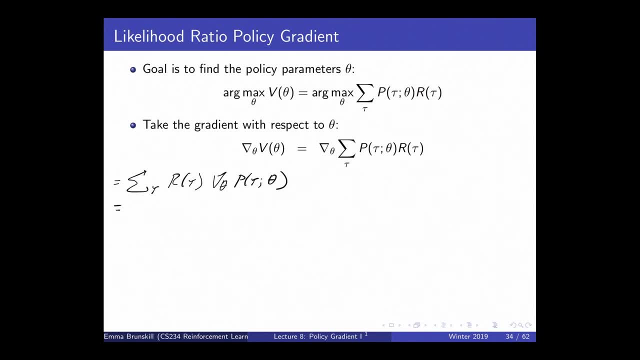 Okay, Okay, Okay, Okay, Okay. So then what we're gonna do is we're gonna do something simple where we just multiply and divide by the same thing. So we're gonna put in probability of Tau given Theta divided by probability of Tau given Theta. 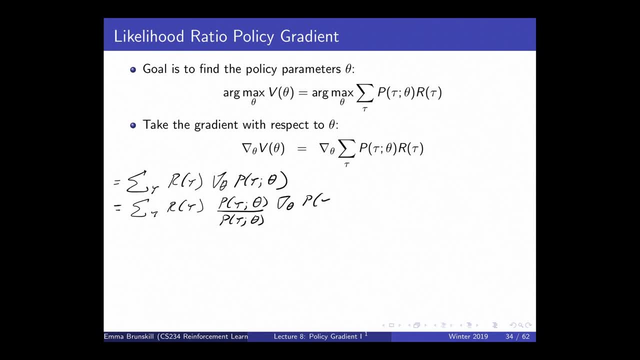 times the derivative of the probability of Tau given Theta And the probability of Tau given Theta and the vergib React, because measure is already wanna be that size. So how many times we can indeed fill in that? how many times is that gonna solve the problem? 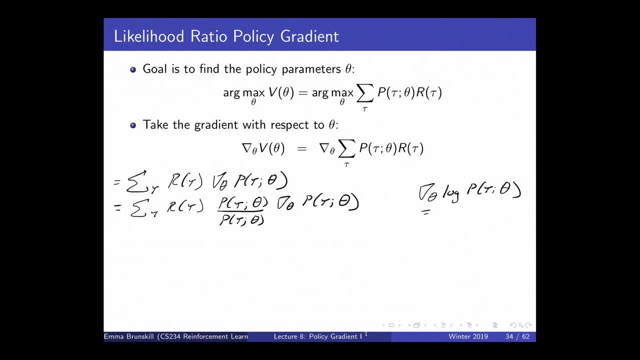 So there we go, Our scale of the probability If we instead had a log. so we're taking the derivative of Log of probability of Tau given Theta. that is exactly equal to the one over the probability of Tau given Theta times the derivative of p of Tau given Theta. 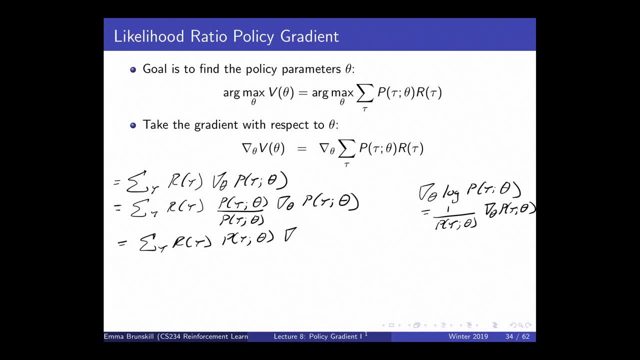 So we can re-express this as follows: times derivative with respect to log of P of Tau. given Theta Now, so far, that doesn't necessarily seem like that's gonna be very useful. Um, so we've done that. that's a reasonable transformation. 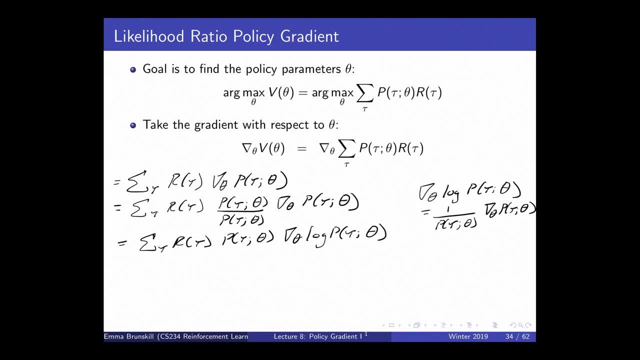 but we'll see shortly why that transformation is helpful And, in particular, the reason this transformation is helpful is it's gonna be very useful when we think about wanting to do all of this without knowing the dynamics or reward models. Um, so we're gonna need to be able to, you know. 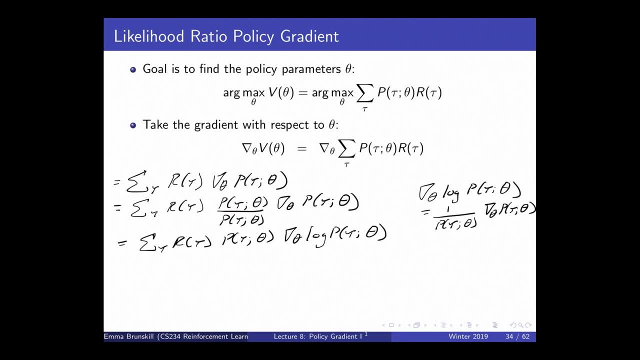 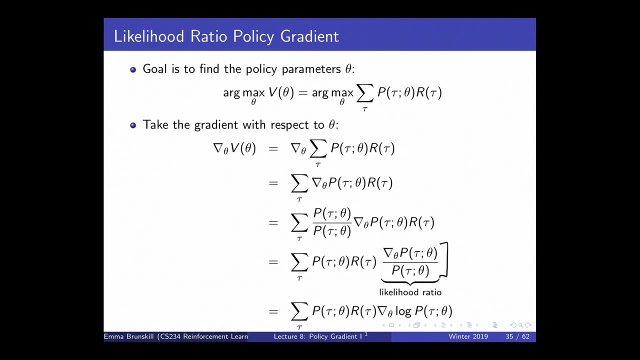 get reward in terms of, uh, a trajectory, But we wanna be able to evaluate, um, the gradient of a policy without knowing the dynamics model, and this trick is gonna help us get there. So when- when we do this, this is often- this is often- referred to as the likelihood ratio. 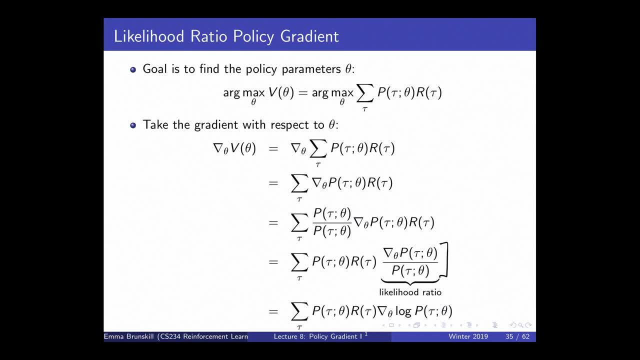 And then we can convert it and just say: well, we noticed that by doing this, this is actually exactly the same as the log. Now why else does this start to look like something that might be useful? Well, what do we have here? 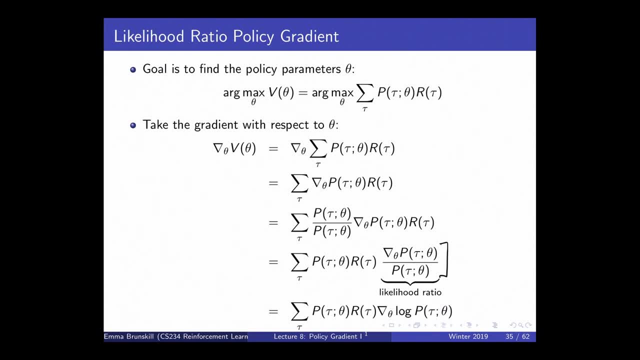 We have if we- this is the sum over all trajectories. of course, we don't necessarily have access to all possible trajectories, but we can sample them, So you could imagine starting to be able to approximate this by running your policy a number of times. 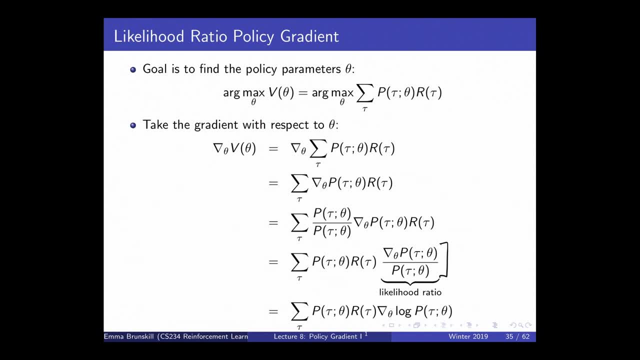 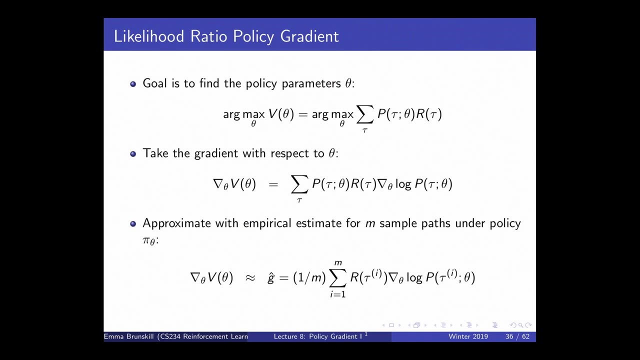 sampling a number of trajectories, looking at the reward of those um and then taking the derivative with respect to this probability of trajectory, given Theta. So typically we're going to do this by just running the policy m times um and then that p of theta. 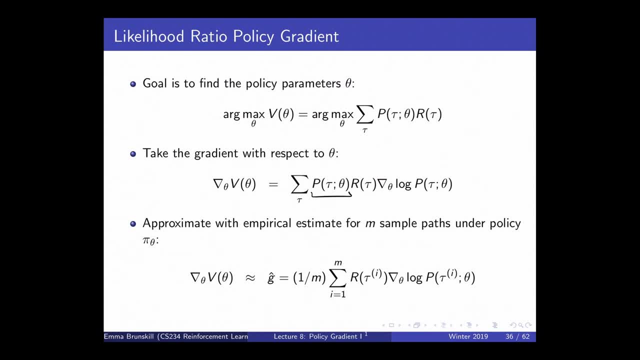 of the tau given theta. we're gonna just approximate that by the following, So that part drops out. We're just going to weigh all of the trajectories that we got during our sampling uniformly and then we look at the reward of that trajectory and the log of p of tau given theta. So what is happening in this case? 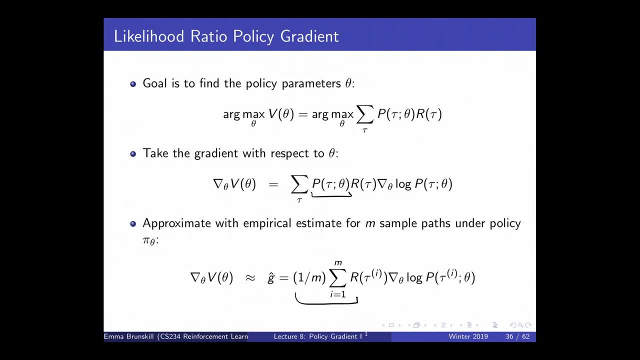 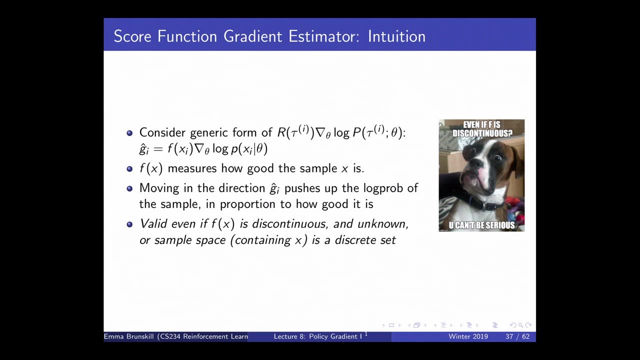 Okay, so this is saying that the gradient is this sort of: the reward we get times, the log of the probability of that trajectory for the reward- associated reward times, theta. So what's happening in that case? So in this case we have a. 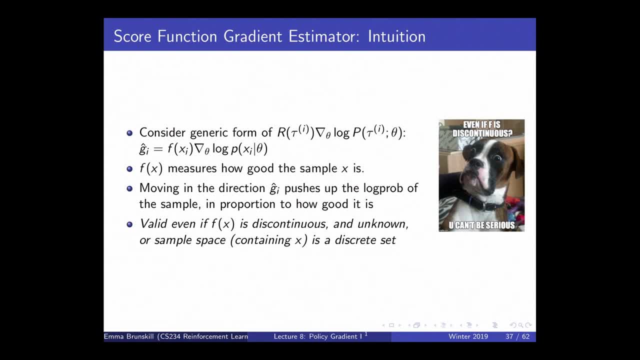 function which, for our case, is the reward, which is sort of measuring how good um that particular, um you know, trajectory is, or how good that sample is, And so what this is doing is we're just moving up in the trajectory of the log. 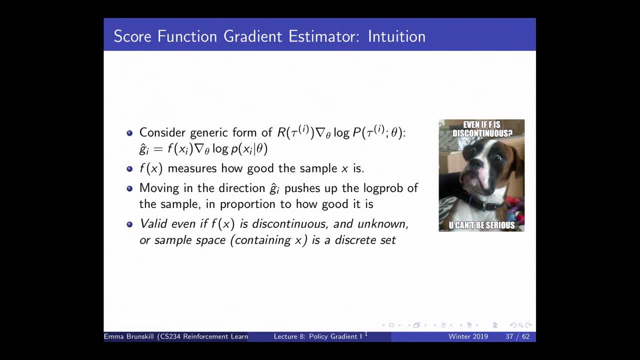 probability of that sample based on how good it is. So we want to sort of push up our parameters that um are responsible for us getting samples which are good. So, um, we want to have parameters in our policy that are going to. 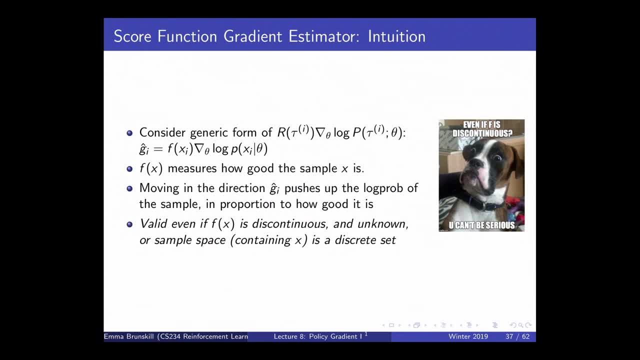 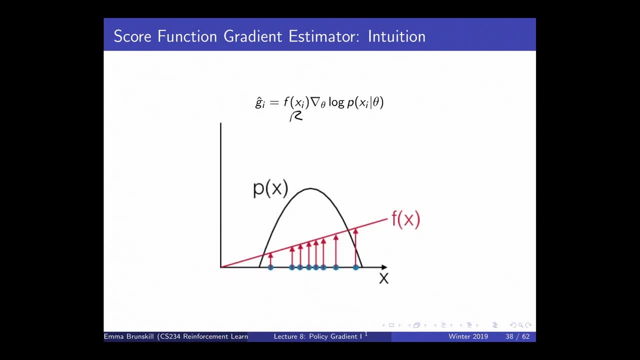 cause us to execute trajectories that give us high reward. So if we think of just sort of here f of x again as the reward we-, this is going to be our policy, our parameterized policy. we want to increase the weight, uh, of things in our space that lead to high reward. 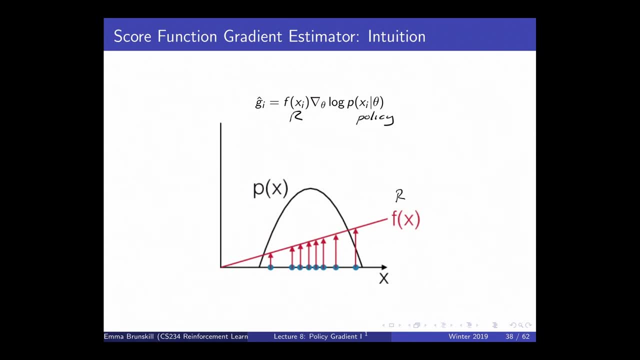 So if this is our f of x, which is our reward function, and this is the probability of our trajectories, then we want to reweight our policy to try to increase the probability of trajectories that yield high reward. So you would end up having larger gradients towards things that have high value, high reward. 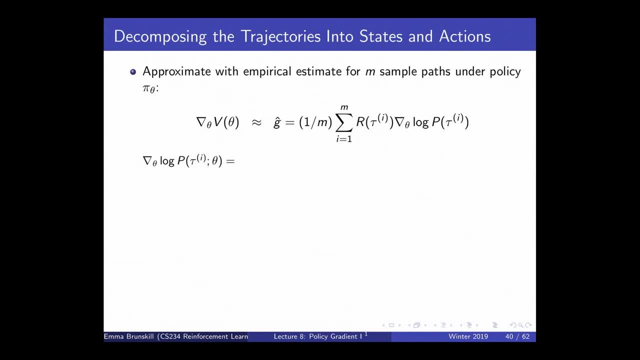 Okay. So then the next question is: if I'm going to do this, then I have to be able to approximately um. Okay, So then the next question is: if I'm going to do this, then I have to be able to approximately um. 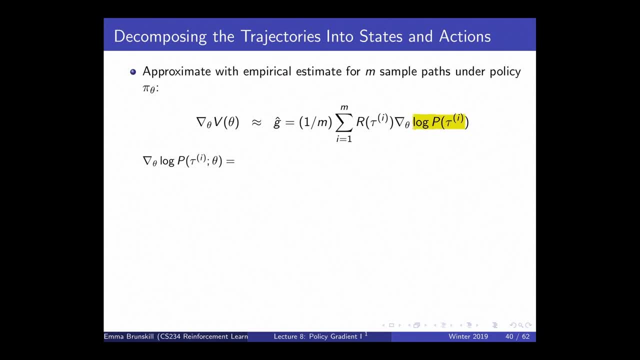 make the second term, which is this log. you know the derivative with respect to the probability of a trajectory um under some parameters. So I have to be able to figure out what is the probability of a trajectory under a set of parameters. 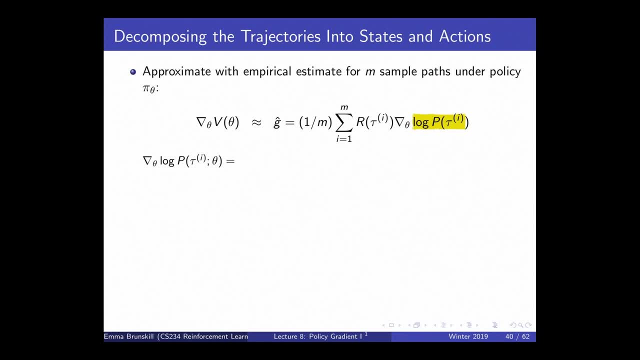 and we can do that as follows. So this is gonna be delta Theta of log of the prod- of mu of S zero. So this is our initial starting state, the probability of our initial starting state. So this is our initial starting state. 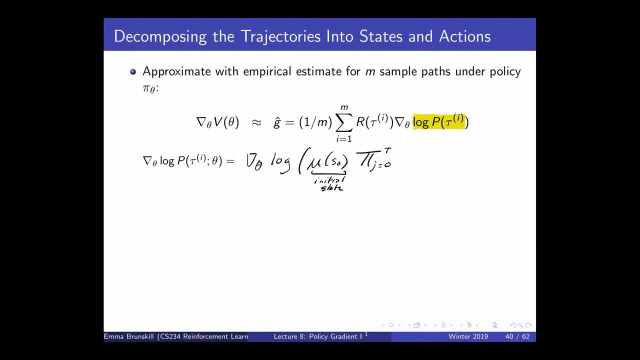 times the product over J equals zero to T minus one of the probability of observing the next state, given the action that was taken times the probability of taking that action under our current policy. So there's like another bracket at the end. Um and so, since this is log, 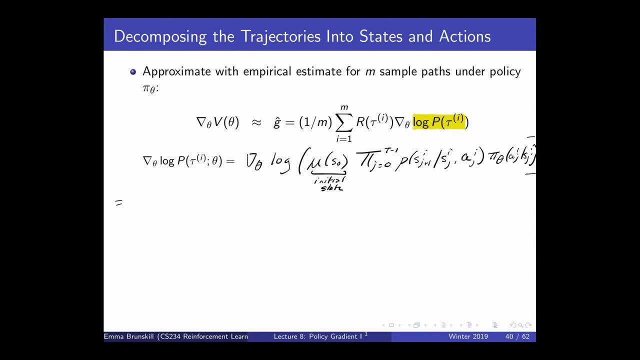 we can just decompose this, So this is gonna be equal to delta Theta of log of mu of S naught plus delta Theta, sum over delta Theta, because it's a log term of J equals zero to T minus one of log of the transition model. 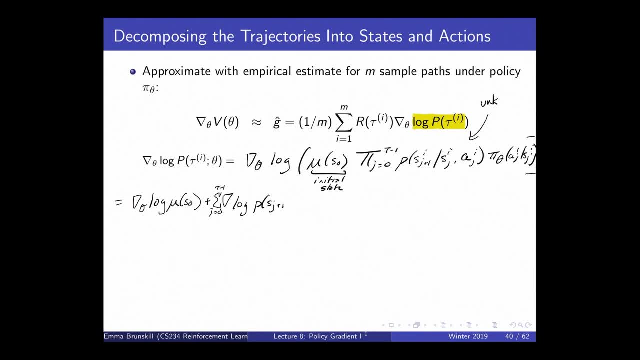 Remember, we don't know this in general, This is unknown. We're just gonna hopefully end up with an expression which means we don't need to have it. Okay, And what I is indexing here is which trajectory we're on. Uh, sum over J equals zero to T minus one. 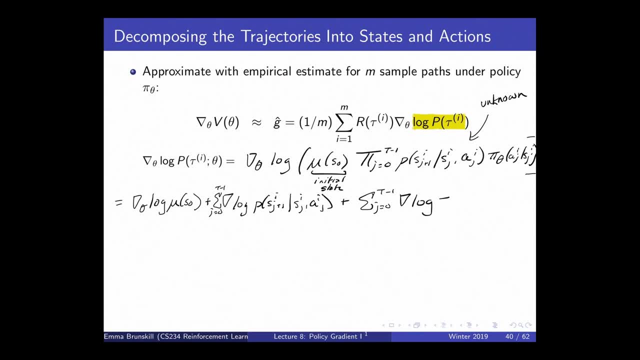 And this is gonna be our actual policy parameters. All right, Can anybody tell me why this is a useful decomposition And whether or not it looks like we're gonna need to? so let me just parametrize all of these things. Um, does this look hopeful in terms of us not needing to know what the dynamics model is? 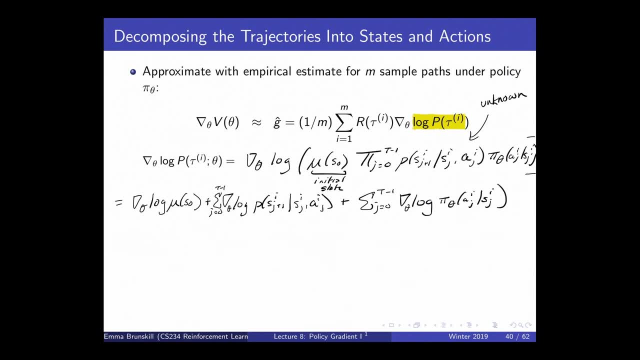 That definitely is right. How about everybody just take a second talk to your neighbor and, um, then tell me which of these terms are going to be zero? So we're taking the derivative with respect to Theta, and which of these terms depend on Theta? 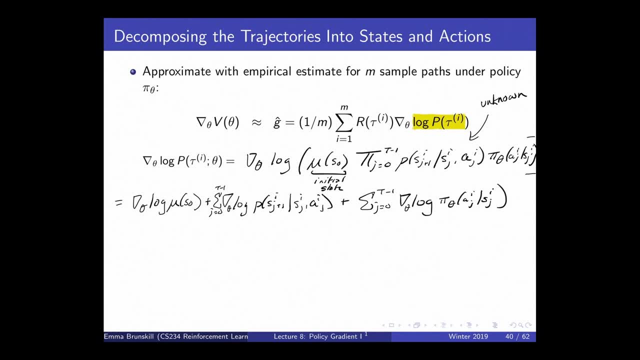 and which of these terms depend on Theta? P, P, P P. 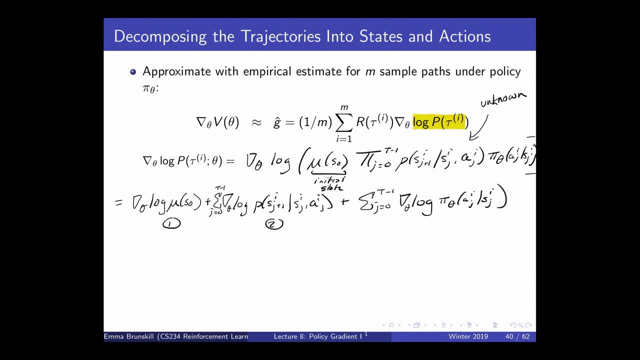 PAR extending ez3 with a p, P, P, Great. So this goes to 0.. So the only thing we have left is this, which is great. So, um, the nice thing. 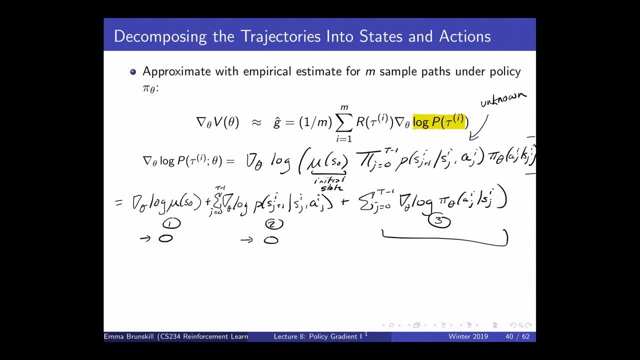 and so now it sort of becomes more clear why we did this weird log um transformation. because when we did this weird log transformation, it allowed us to take this product of the probability of the action that we took and the state transitions. then instead we can decompose it into sums. 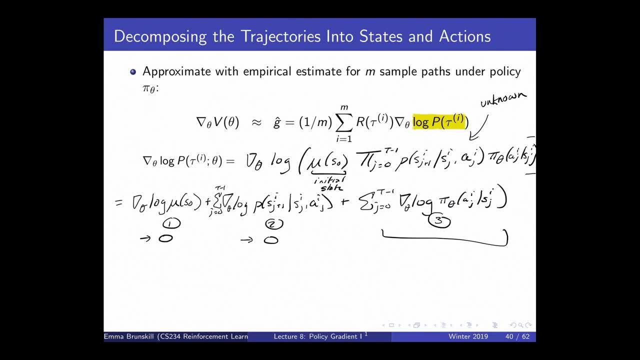 And now, once we see that we decompose it into sums, we can apply the derivative separately, and that means some of these terms just directly disappear, Which is really cool. So it means that we don't actually need to know what the transition model is. 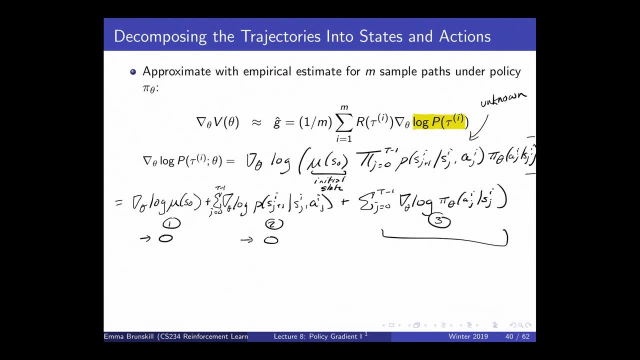 Um, we don't need to have explicit representation. Yeah, question and name first, please. And the question is, I was wondering: doesn't the dynamics of the system depend on the policy though? um, in general, Great question. So the question is: 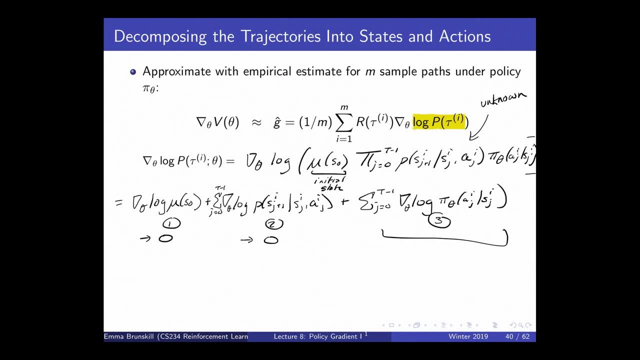 doesn't the dynamics of the system depend on the policy? Absolutely, but only through this part. So it's like, um, the agent gets to pick what action they take, but once they pick that, the dynamics is independent of the agent. 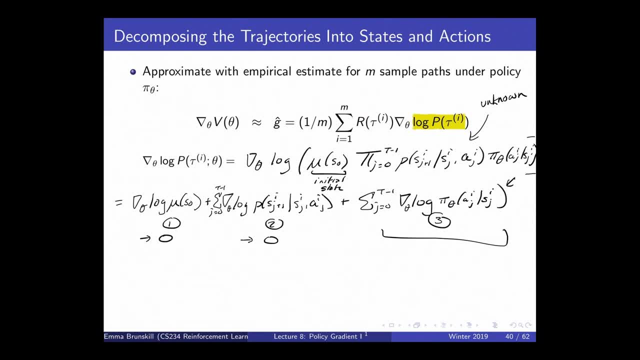 And so it's this decoupling. So if you have a different policy, you will absolutely get different trajectories, but the way in which you'll get different trajectories um is only affected by the policy in terms of the actions that are selected. 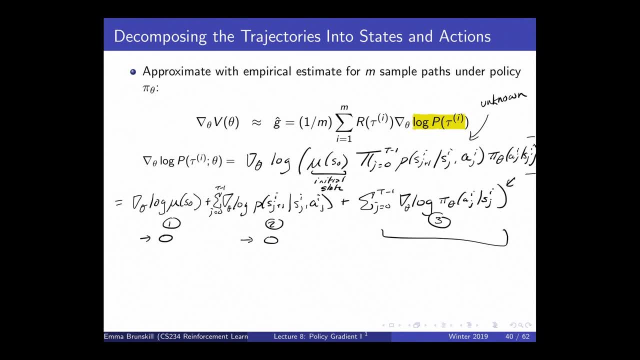 and then the environment will determine sort of the next states that you get, And so we don't need to know that, in terms of um estimating the impact of the actions on the environment, It'll also come through in terms of the rewards you get. 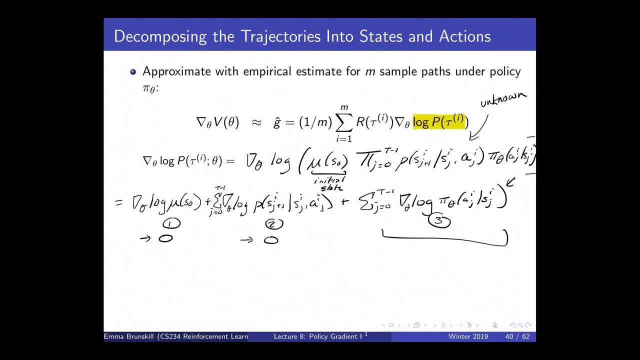 because the rewards you get are also a function of the state, So you'll absolutely visit different parts of the state depending on the actions you take. Any other question? Yeah, I just want to make sure I understand how I get the estimate for the probability of how you can do the data. 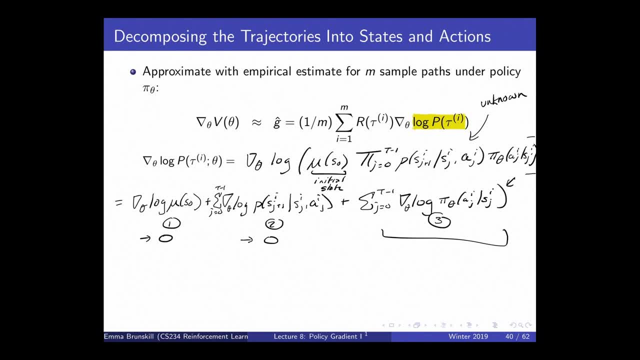 Um, it looks like we're just saying, if it could M episodes and this one showed up. you know I times and it can be I over M Is. is that what we are doing here? Is that correct Great question. So Andrew is asking. 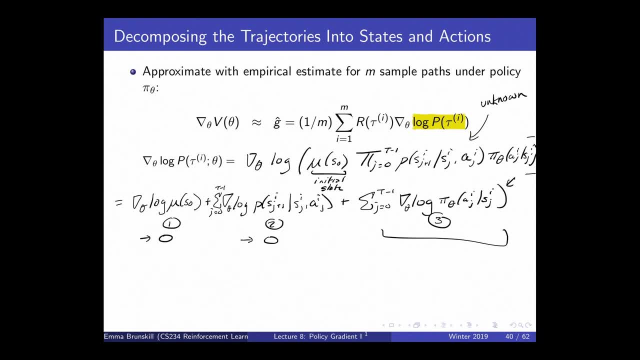 um, you know, this is- what I put here is just one of those internal terms that would cope for one to I yes. So what we're doing here is we're saying: we're gonna take this policy, we're gonna run it m times. 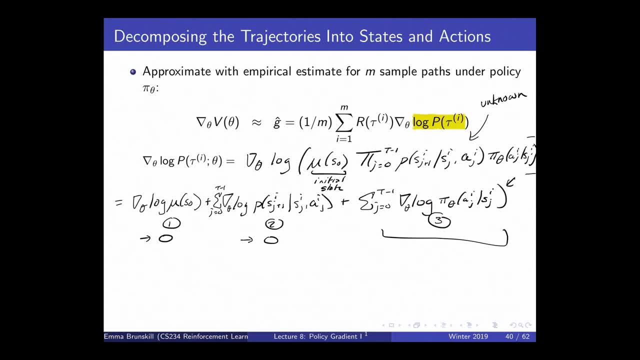 We're probably not gonna get any trajectories that are identical, Um, and what we're gonna do is compute this log of the probability of trajectory for each of those separately, um and then sum them up. You might end up with it, I mean, you know. 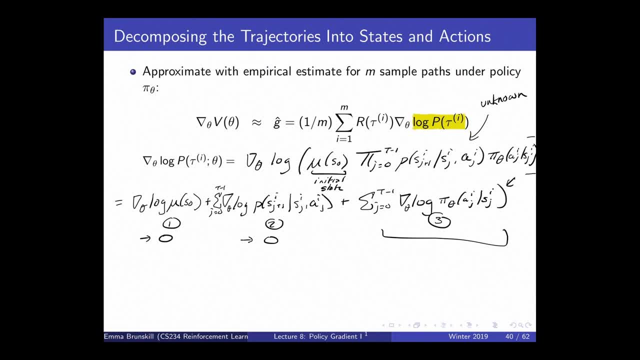 in deterministic cases you might um uh. or if your domain doesn't have a lot of stochasticity and neither does your policy, you might end up with multiple trajectories that are identical In general. all your trajectories will be completely different, And so will your estimate of their local gradients. 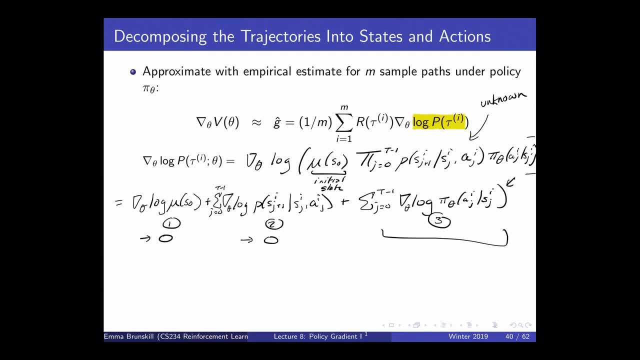 So this is really nice. We're gonna end up with this situation where we only have to be able to have an analytic form for the derivative of our policy with respect to our parameters. So we still need- and we'll talk about this a little bit more later- 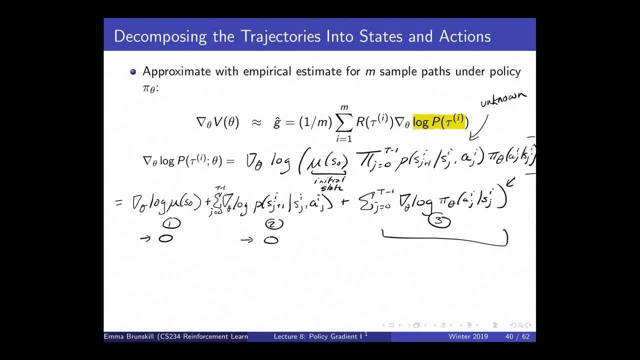 we still need this. we have to evaluate this. This is about how we've parameterized our policy, And if we want this to be analytic, we need to have parameterized our policy in a way that we can compute this exactly for any state in action. 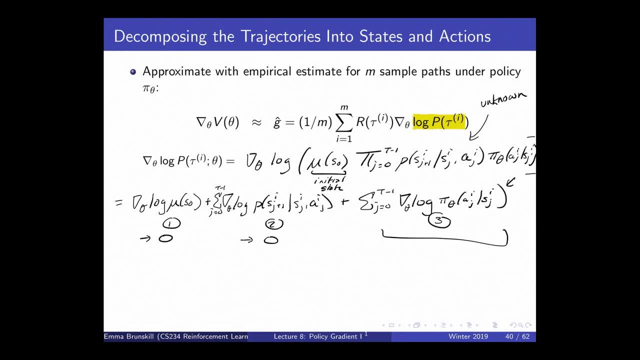 So we'll talk more about some ways, you know, some policy parameterizations which make this computation analytic and nice. In other cases you might have to estimate this thing itself by you know brute force or computation or finite differences or something. 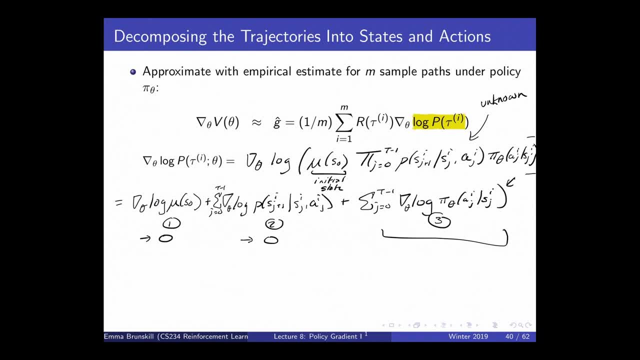 But if we choose a particular form of parameterized policy, then this part is gonna be analytic. So another thing is: I don't find this, but um, uh, I don't find this additional terminology particularly helpful, but it's used all over the place, so I want to in turn. 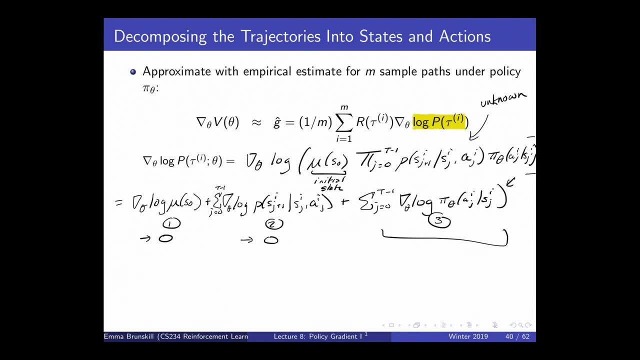 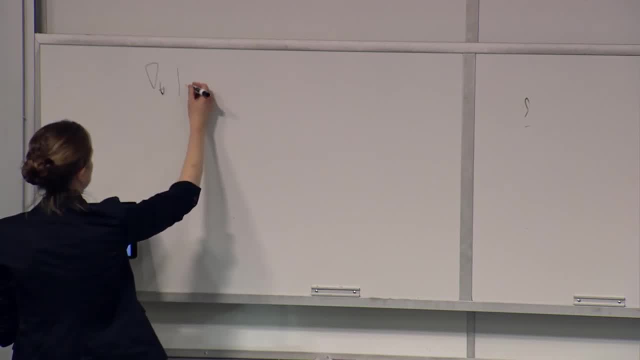 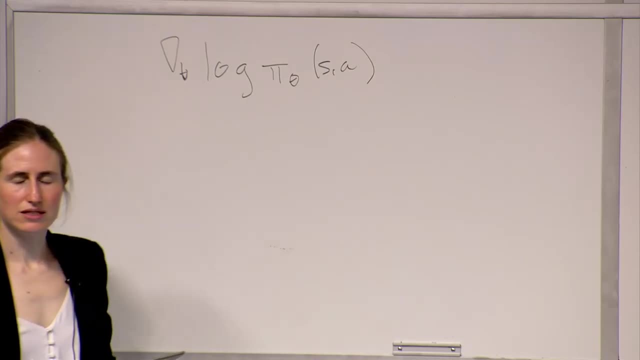 introduce it, which is people often call um this part a score function, Just a score function, which is not particularly helpful, I think, but nevertheless is often used, is called this. So that's the quantity that we were just talking about needing to be able to evaluate. 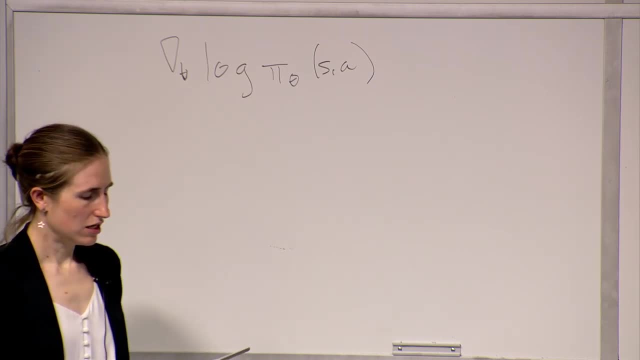 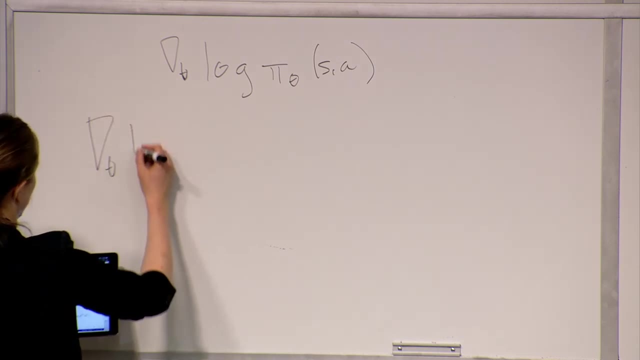 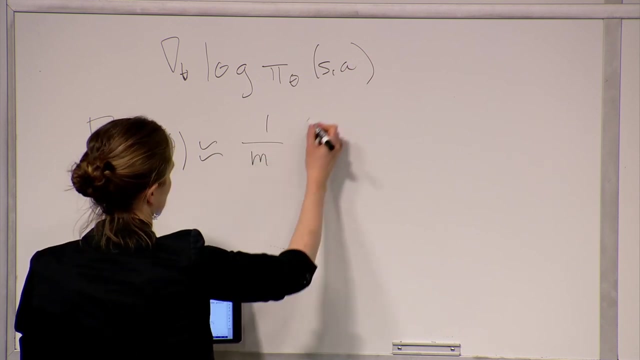 So this really gets into um a-. well, we'll- we'll write it out again. So, um, when we take the derivative of the value function, we approximate that by getting m samples and we sum over, i equals 1 to m. 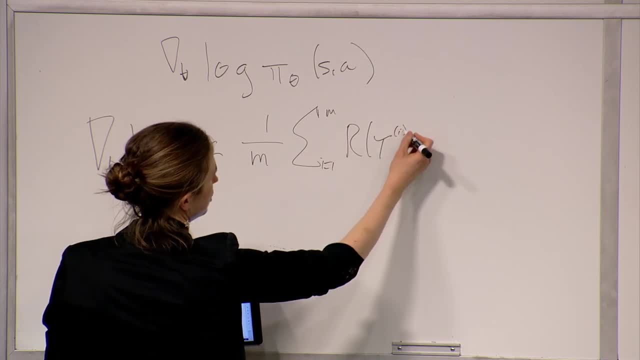 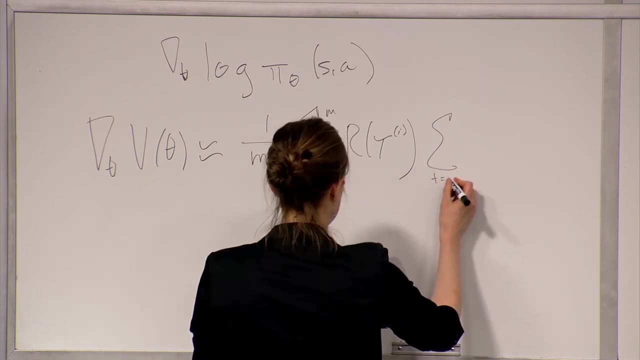 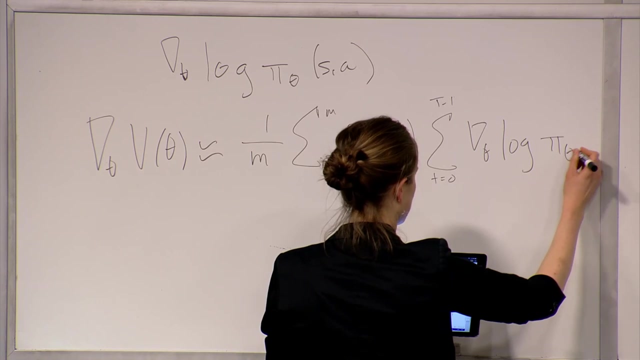 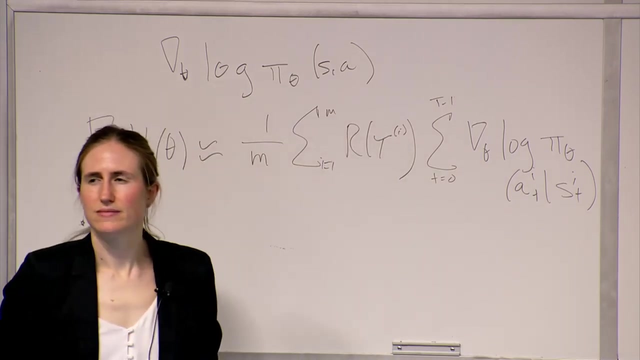 and we look at the reward for that tra- the i- um trajectory, and then we sum over these per-step score functions. Can anybody read that in the back? Yeah, Okay, great Yeah. So these are sort of our score functions. 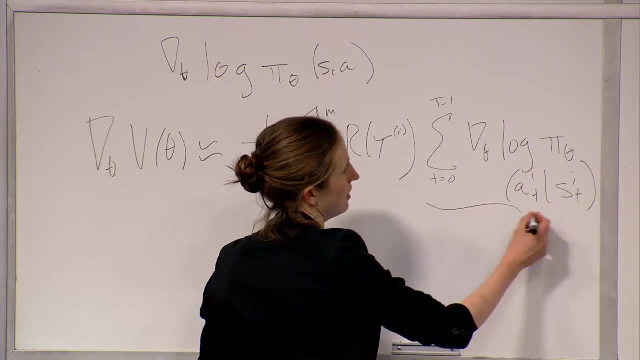 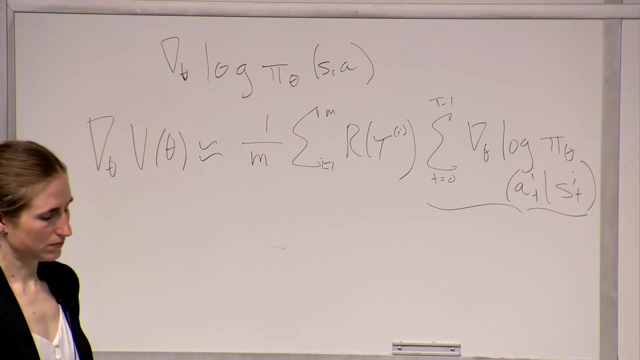 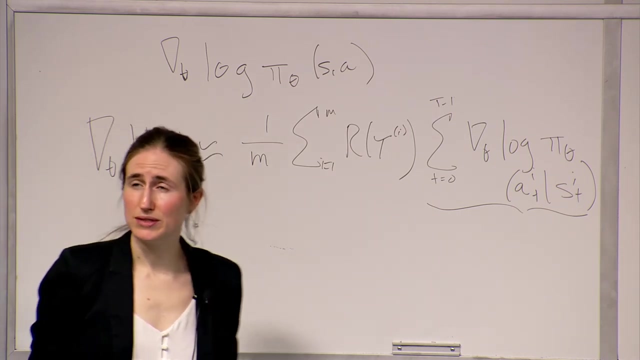 and these are our score functions. um can be evaluated over every single state action pair. that we saw, and we do not need to note the dynamics model. So the policy gradient theorem slightly generalizes this. How is it gonna generalize this Note in this case? what we're doing here is we're 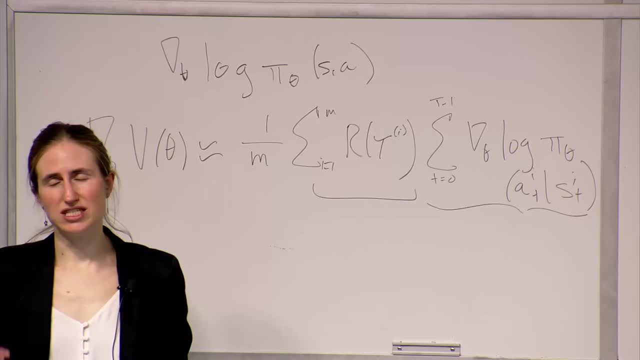 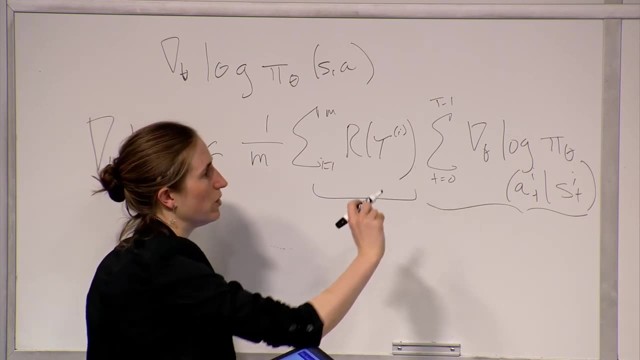 this is for the episodic setting and this is for when we just take our raw- our raw reward functions. So we look at the sum of rewards for that trajectory and then, um, we weigh it by this sort of derivative with respect to our policy parameters. 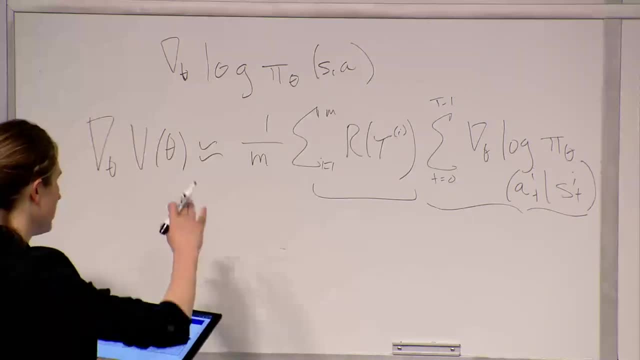 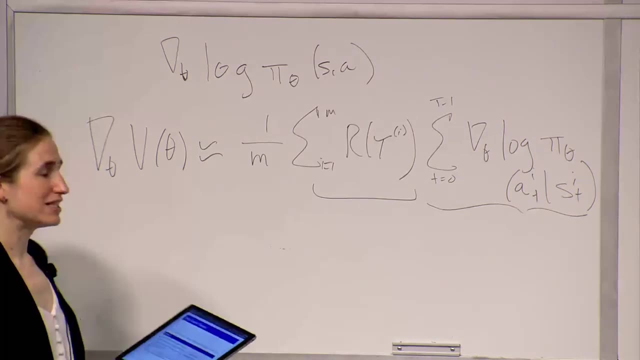 Um, it turns out that we can also slightly generalize this. And let's say: I'm gonna call- so this is a value function. Um, let's say that we had slightly different objective functions. We talked before about how we could have episodic reward. 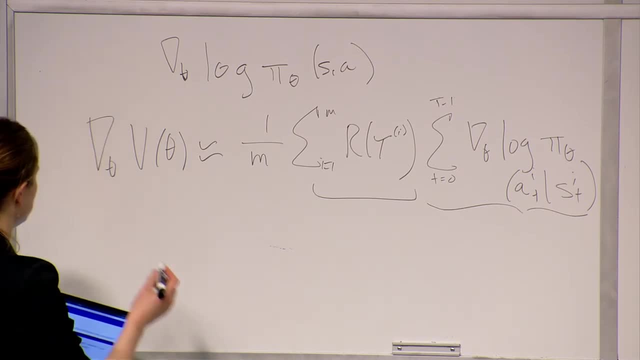 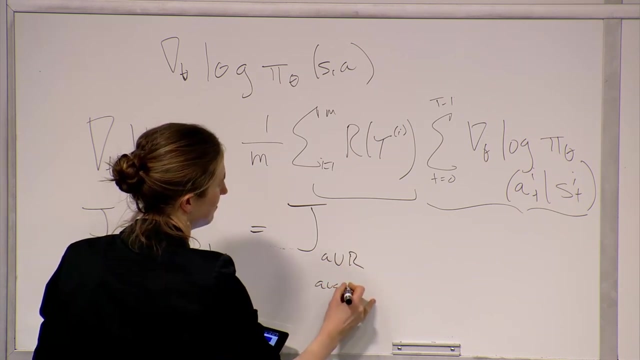 or average reward per time step or average value. So we could either have our objective function be equal to our normal value for episodic, or we could have it equal to what I'm gonna call J, A, V, R, which is average reward per time step. 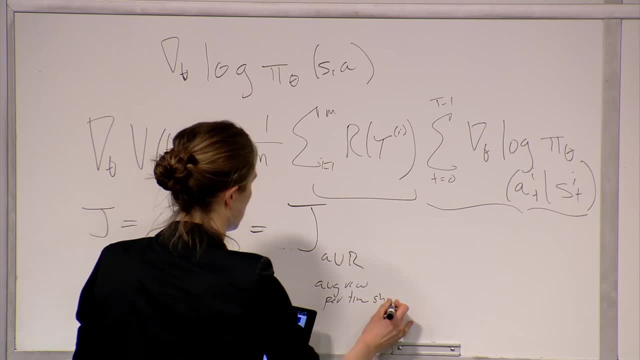 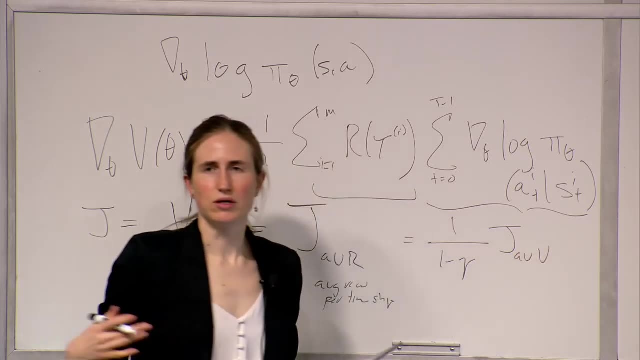 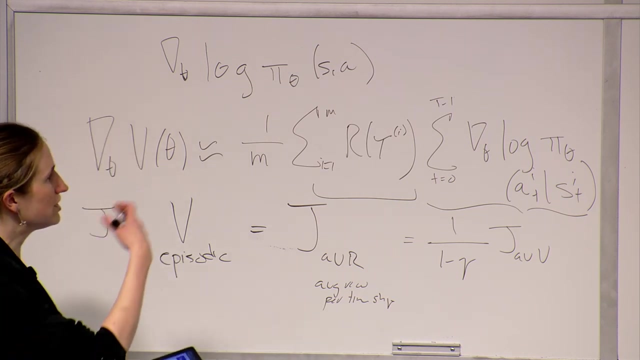 or we could have it as average value. Let's say we're always continuing and we want to average over the distribution of states that we encounter. So we could think about that scenario too. Turns out in all of those cases is you can do. 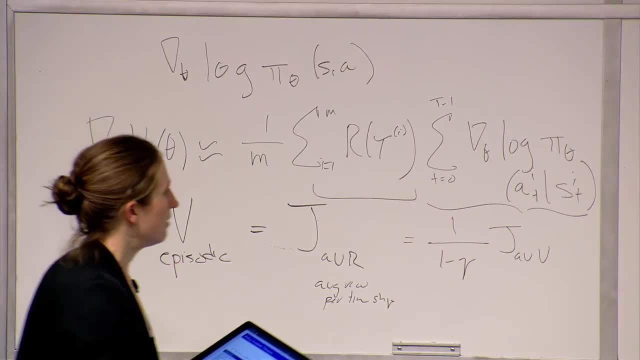 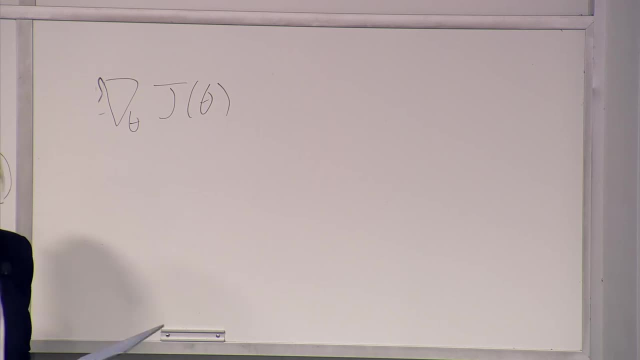 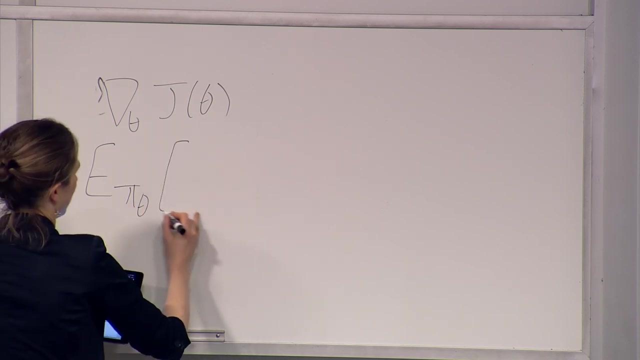 a similar derivation to what we did here for the episodic case, And what we find is that we have the derivative of our objective function, which now can be kind of. any one of these different objective functions is equal to the expected value. under that- the current policy of 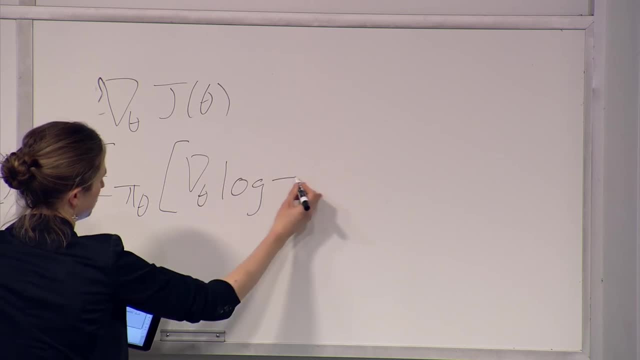 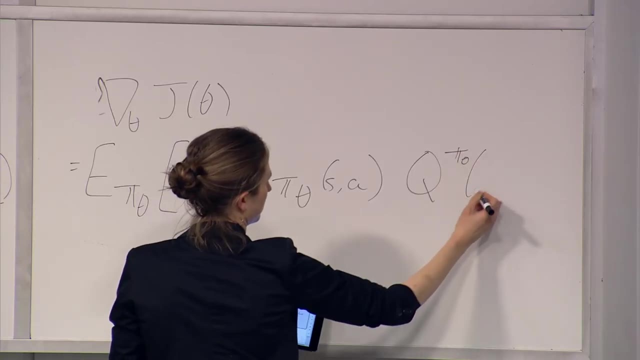 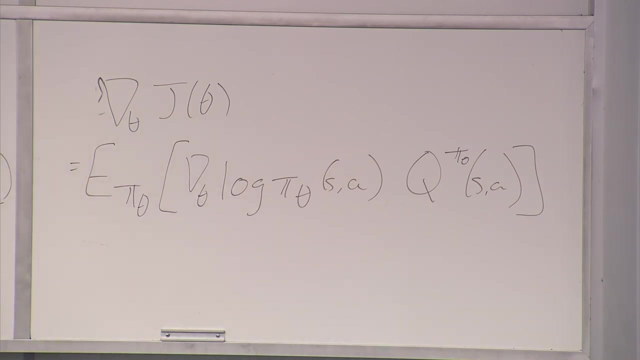 the derivative with respect to just those policy parameters, times Q And Sutton-Rombarto in Chapter 13,, which we also reference on the on the schedule. um have a nice discussion about a number of these different issues. Um and so again. 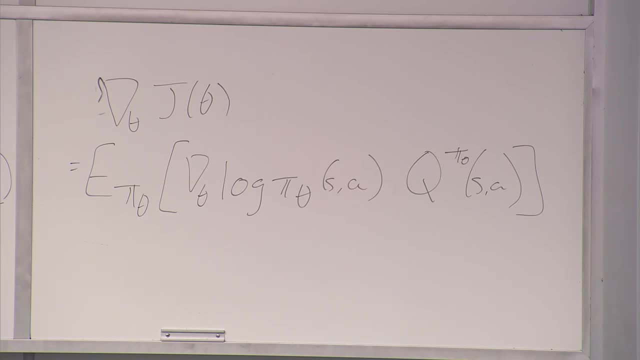 we're not gonna talk too much about these slightly other different objective functions, but just know that this all can be extended to the continuing case. Okay, So what we've said here so far is that we have this approximation where what we do is we just take our policy. 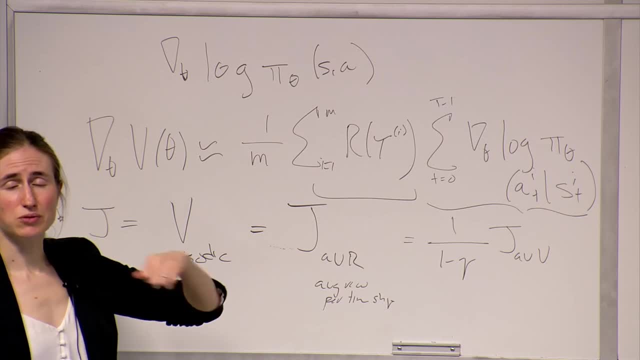 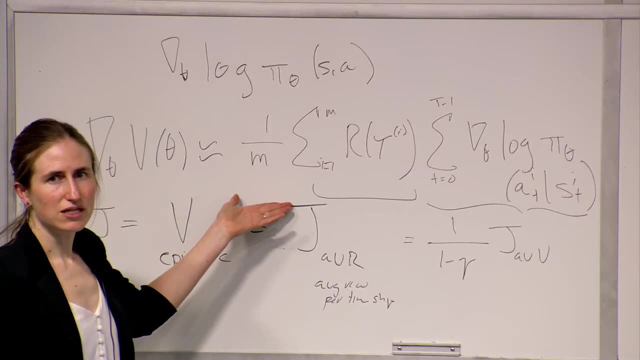 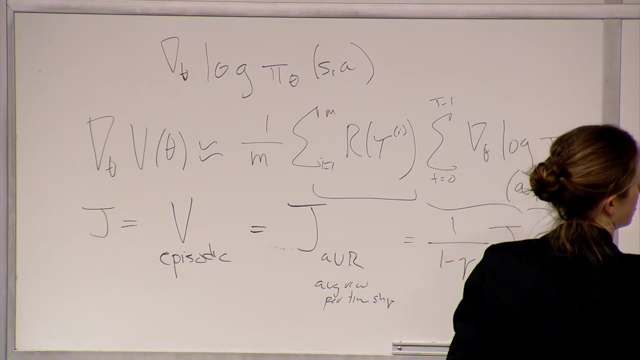 we run it out five- m times. For each of those m times we get a whole sequence of states and actions and rewards and then we average And this is an unbiased estimate of the policy gradient, but it's very noisy, So this is gonna be unbiased and noisy. 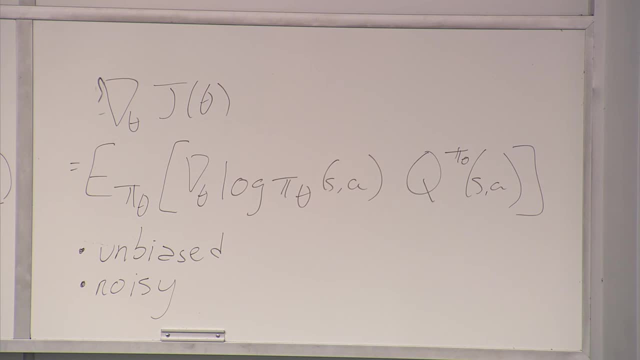 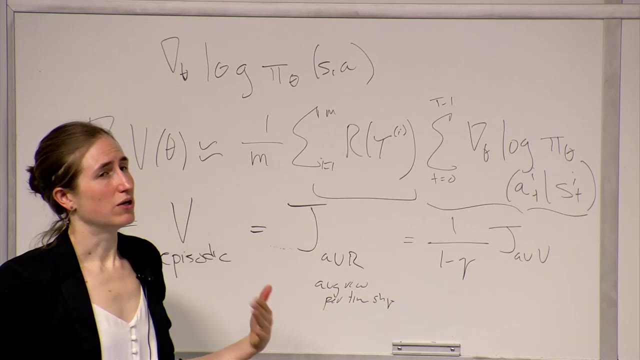 If you think about what we saw before for things like Monte Carlo methods, it should look vaguely familiar. same sort of spirit, right, We have. um, we're just running out our policy, we're gonna get some- sum of rewards. 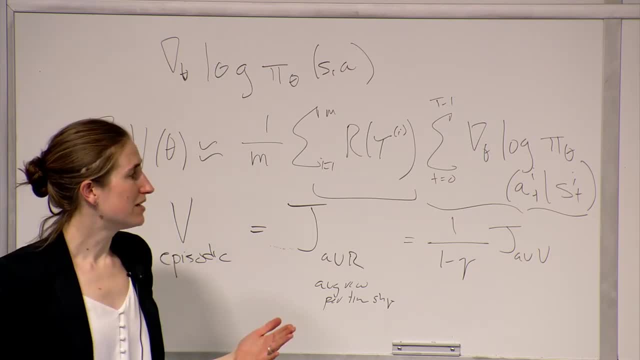 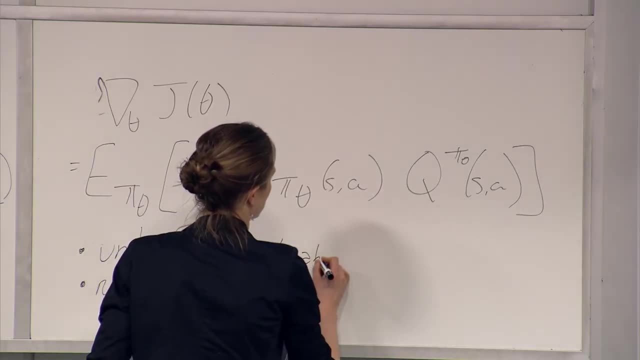 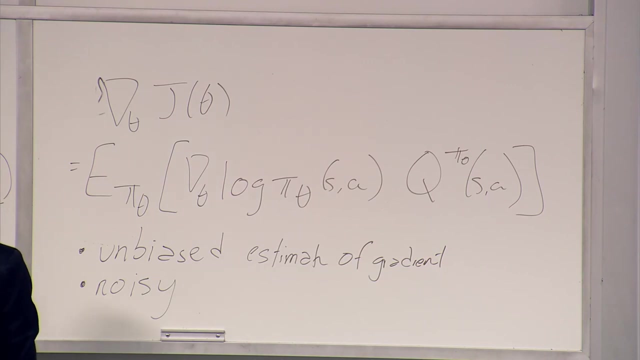 just like what we got in Monte Carlo um estimates But- so it'll be unbiased estimate of the gradient. so it's unbiased estimate of the gradient. estimate of gradient, but noisy. So what can make if it's actually practical? 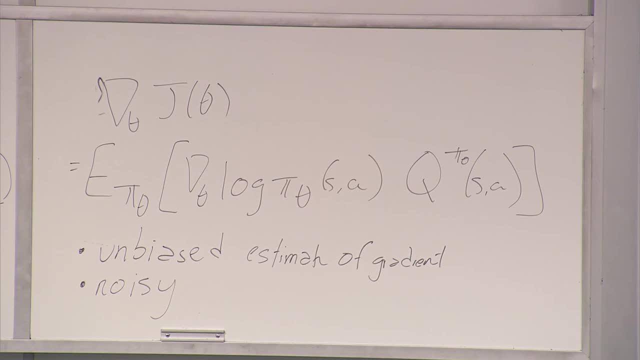 Um, there's a number of different techniques for doing that. Um, but some of the things we'll start to talk about today are temporal structure and baselines. Okay, So how do we fix this? We're gonna start to look at, you know. 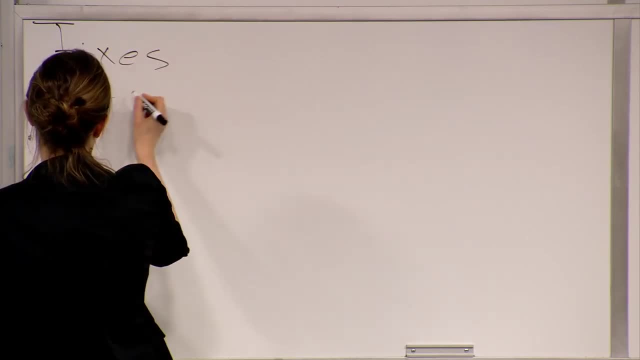 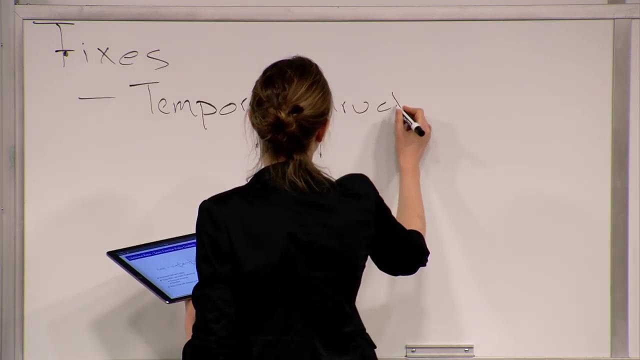 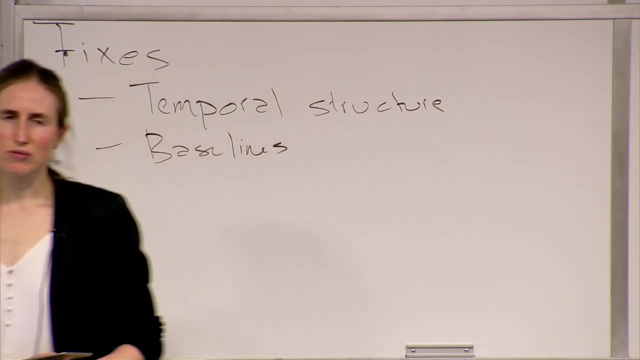 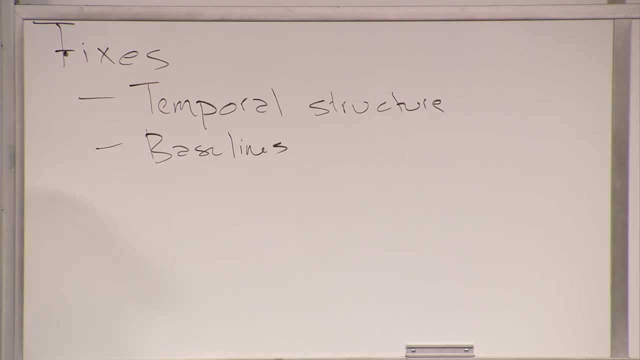 fixes are temporal structure and baselines. And before we keep going on this, um, based on what I just said in terms of Monte Carlo estimates, um what are some of you guys' ideas for how we could maybe reduce the variance of this estimate? 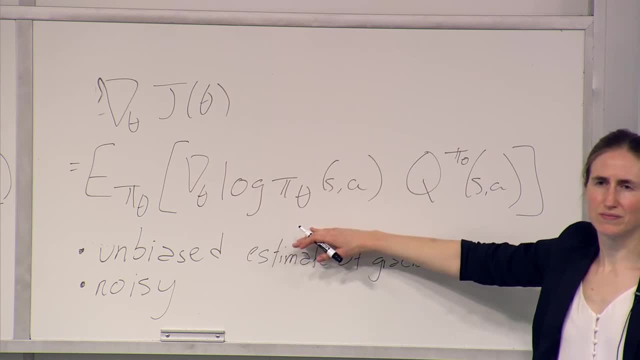 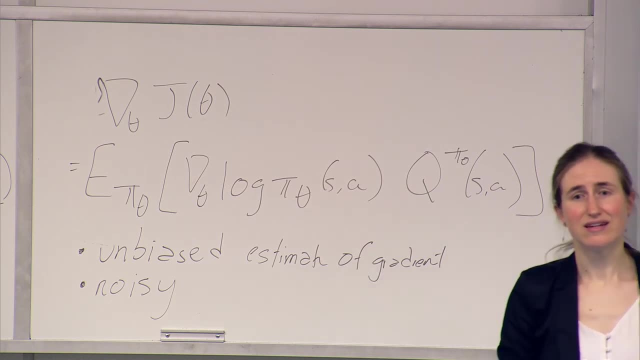 based on stuff we've seen so far in class, Like what are the alternative to kind of Monte Carlo methods? Yeah, Could you use bootstrapping, Um, I mean first do you know? Yeah, What you said is exactly right. 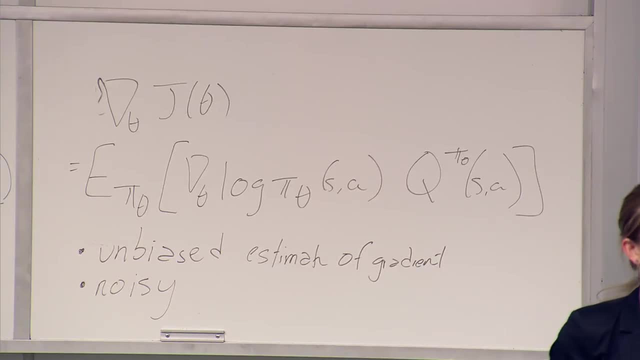 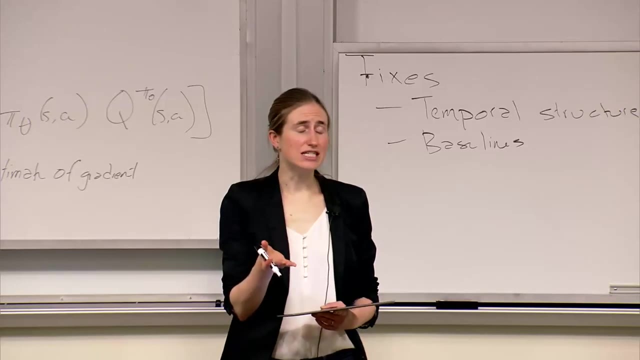 So Deanne said: could you use bootstrapping? Yeah, So we've repeatedly seen that um we have this trade-off between bias and variance and that bootstrapping- um like temporal difference methods that we saw in Q-learning that you're doing in DQN, can be. 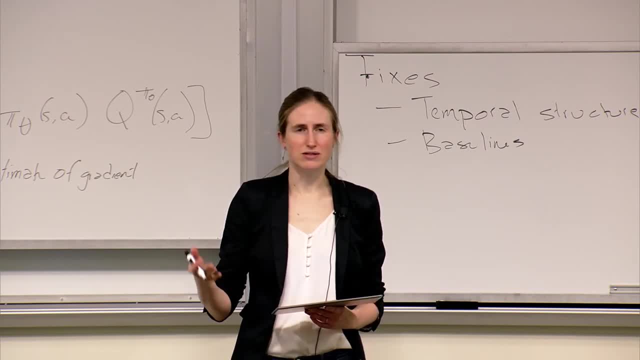 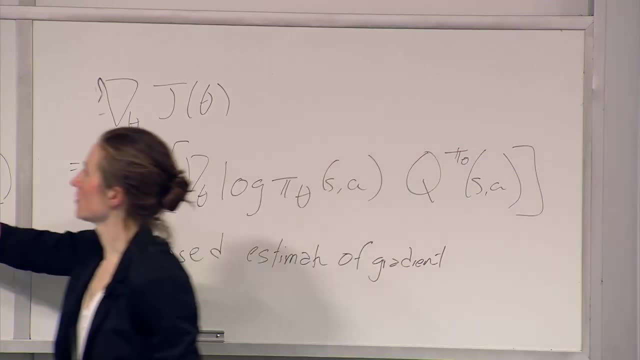 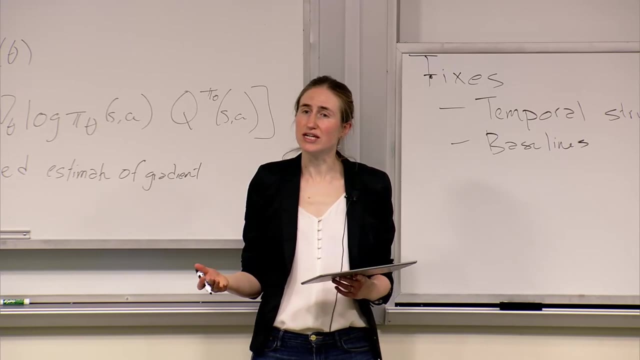 helpful in um reducing variance and- and speeding the spread of information. So yeah, So we could absolutely do things like bootstrapping um to kind of replace R with something else, or use um, a covariate in addition to R, to try to reduce the variance of R. 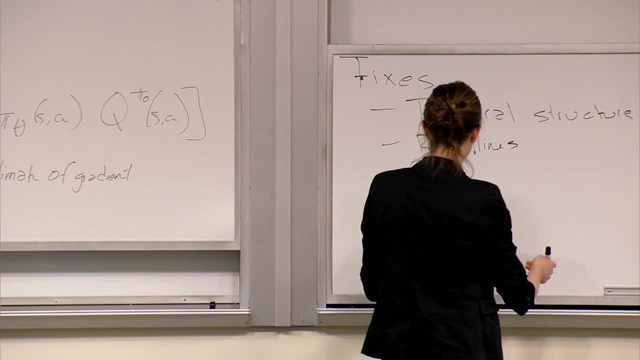 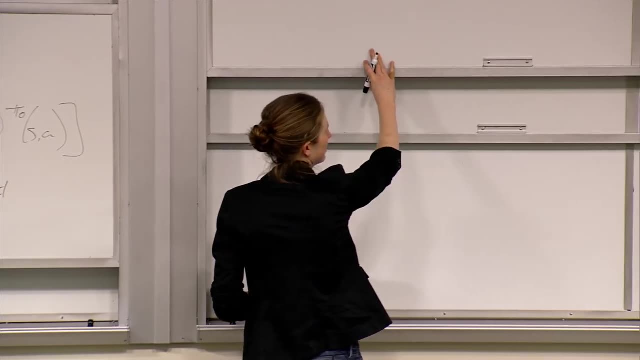 Okay, All right. So what we're gonna do now is we're first gonna do something that doesn't go all the way to there, but tries to at least leverage the fact that we're in a temporal- temporal um process. 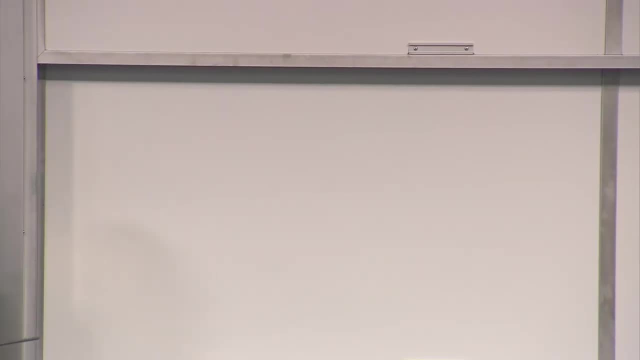 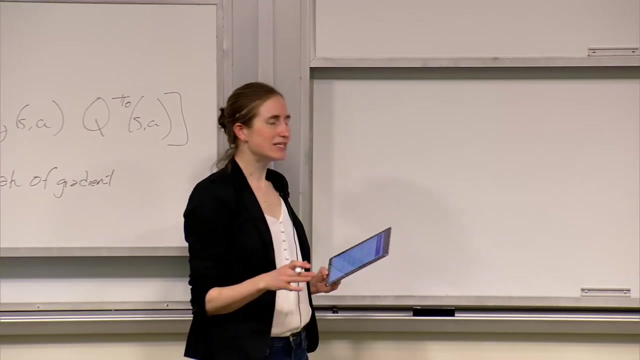 Okay, Um, and for any of you who have played around with important sampling before, this is closely related to um, per-decision, important sampling and basically the um thing that we're going to exploit is the fact that 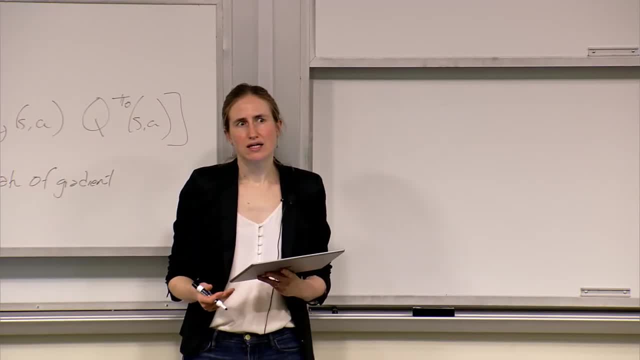 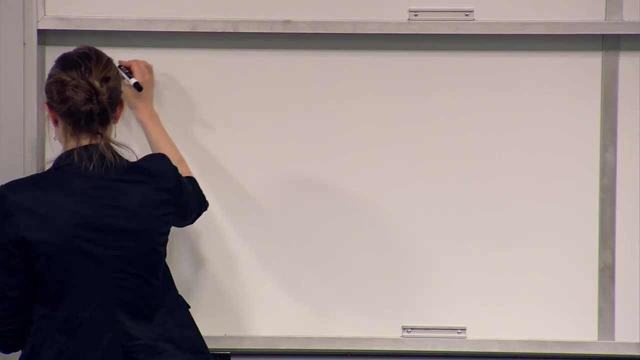 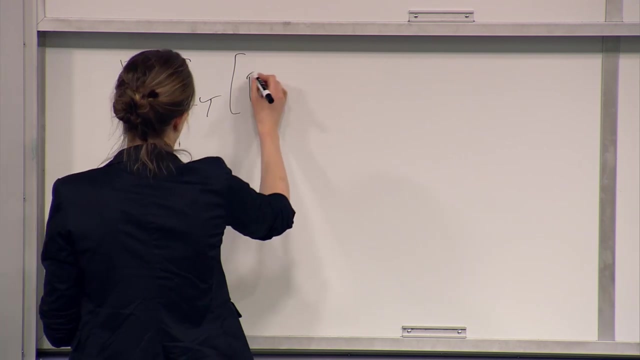 um, the reward. I can only the temporal structure of the domain. I'll write it out first. Okay, So what we had before is we said that the derivative with respect to theta of the expected value of tau of the return is equal to the expected value under the. 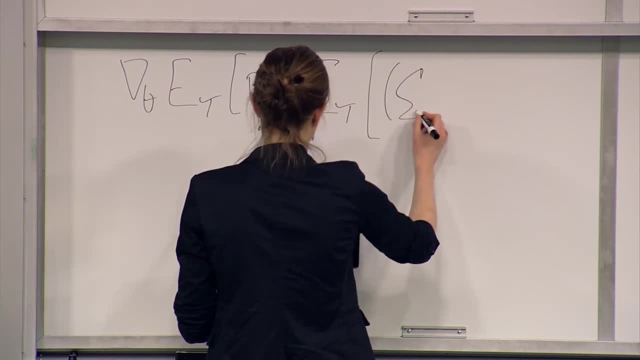 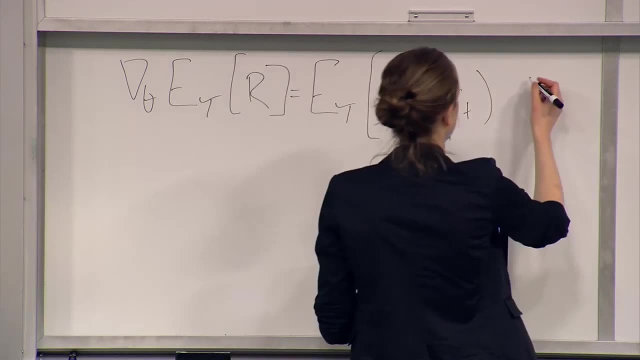 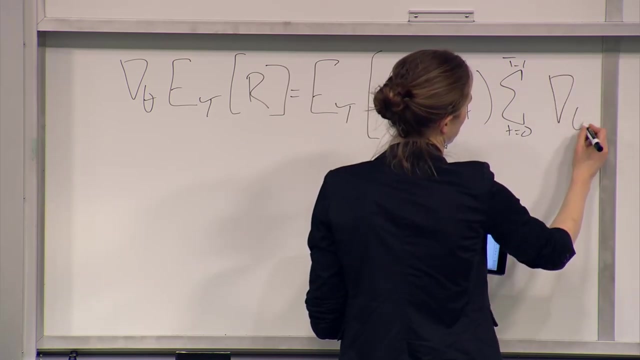 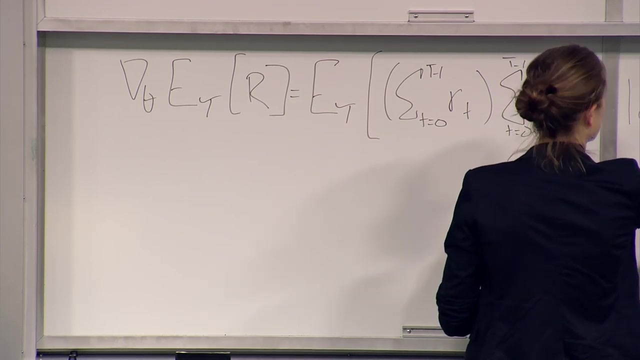 trajectories you could get of the sum over t equals 0 to t minus 1 of RT, So just the sum of rewards you get. times this sum over t equals 0 to t minus 1 of your derivative with respect to your policy parameters. That's what we had. 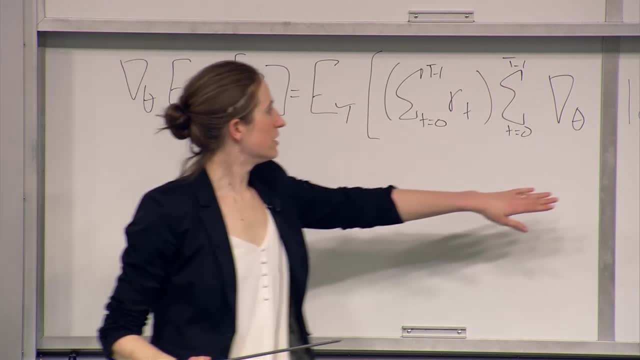 before. So we just sum up all of our rewards and then we'd multiply that by the sum over all of the gradients of our policy at every single action state pair we can get. So the sum over t equals 2, over t equals 0 to t minus 1 of RT. So 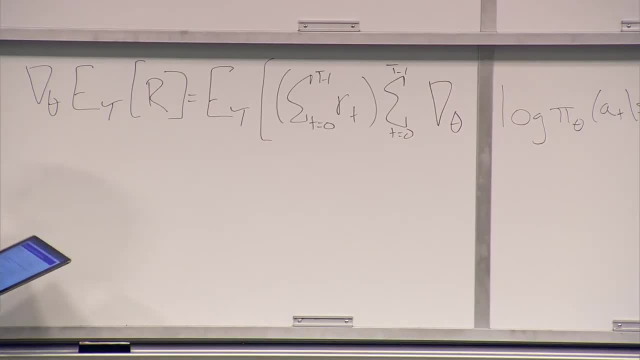 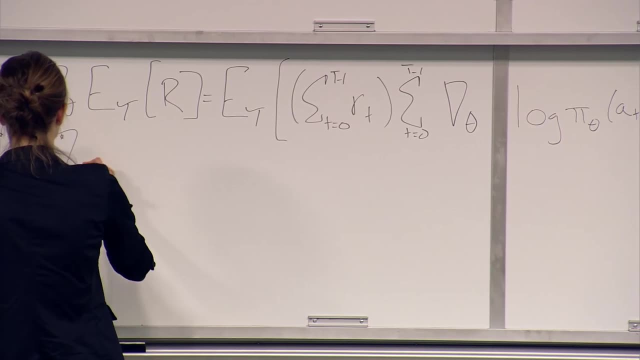 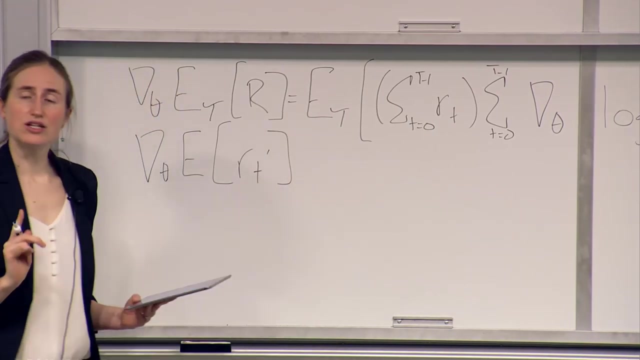 got in that trajectory. So let's think about doing this for a single reward instead of looking at the whole sum of rewards. So let's just look at- we take the derivative with respect to theta of expected value of r t prime. So this is just a single time step reward that we might encounter. 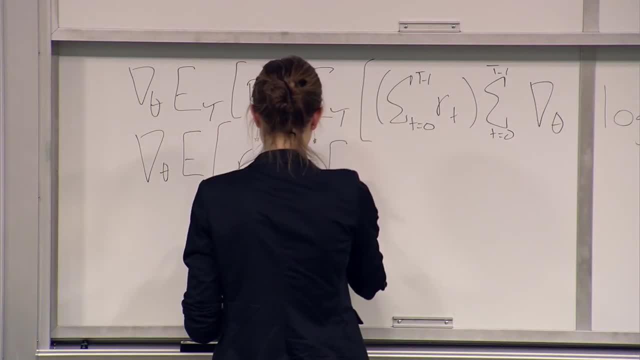 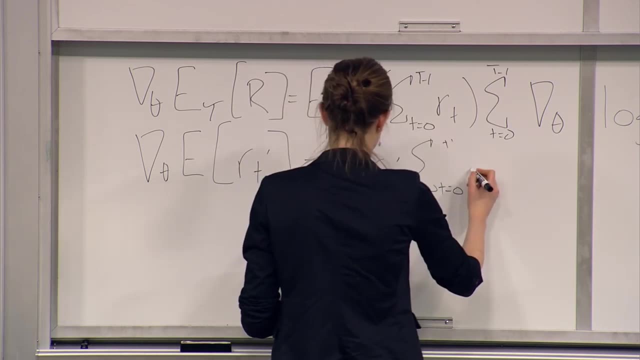 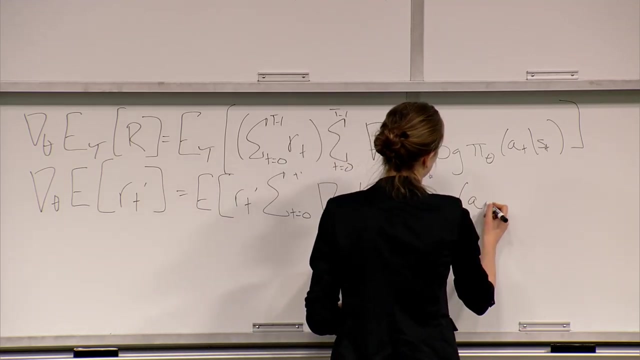 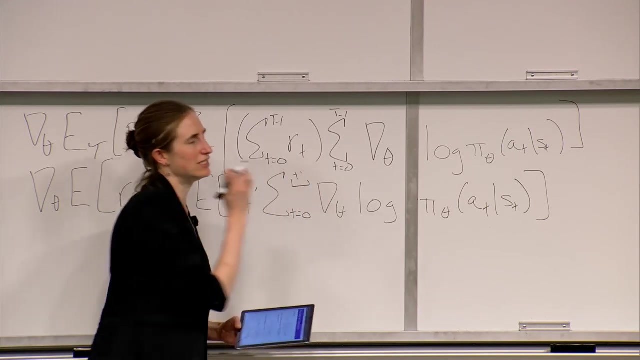 you know along our trajectory, And that's going to be equal to the expected value of r t prime times sum over t equals zero to t prime of this derivative. So this is going to look almost exactly the same as before, Except the only key difference here is that I'm only summing up to t prime. 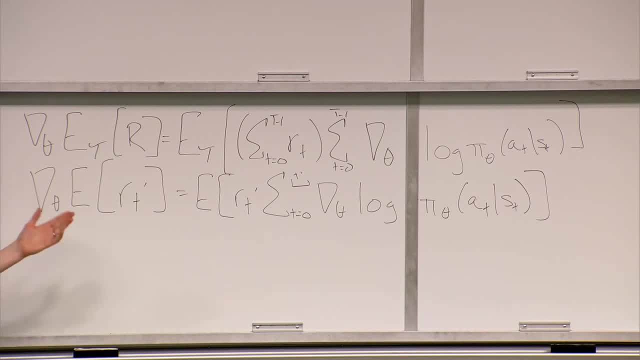 Okay, So we're only summing up. you can think of this as just like a shortened trajectory. I'm looking at the product of, you know, the sum of r t prime times sum over t equals zero to t prime- The states and the actions and the rewards that I reached all the way up to when I got to r t prime. 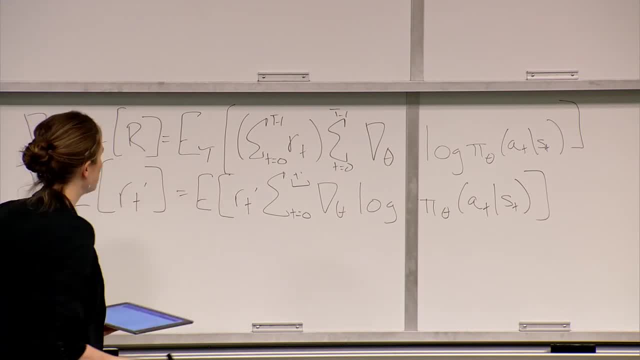 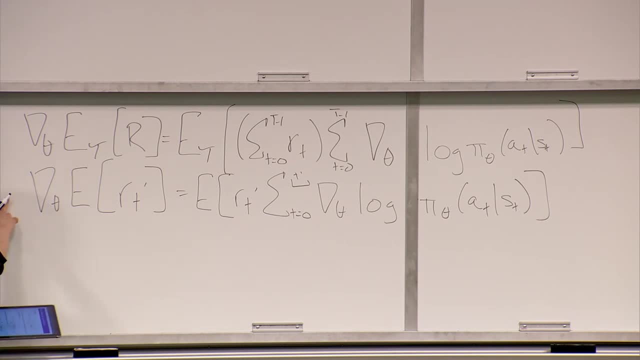 Okay, So I don't have to sum all the way over the future ones. So we can take this expression: and now we can sum over all time steps. So this says what's the expected reward, the derivative with respect to the reward for time, step t: prime. 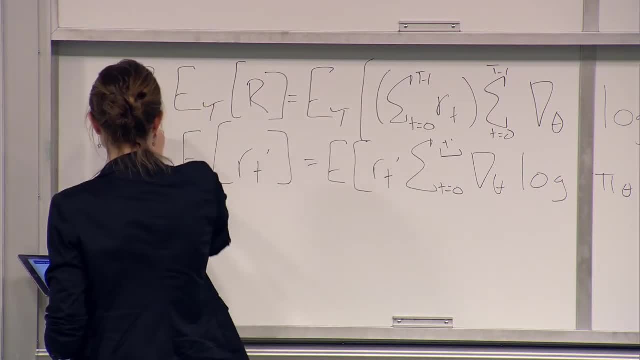 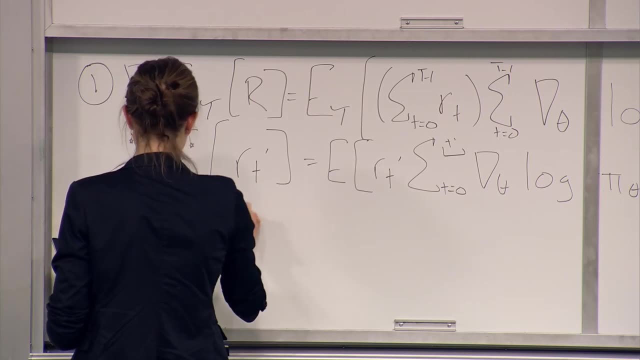 Now I'm going to just sum that, And that's going to be the same as my first expression. So what I'm going to do is I'm going to say: v of theta times. t prime Is equal to the derivative with respect to theta of e r. 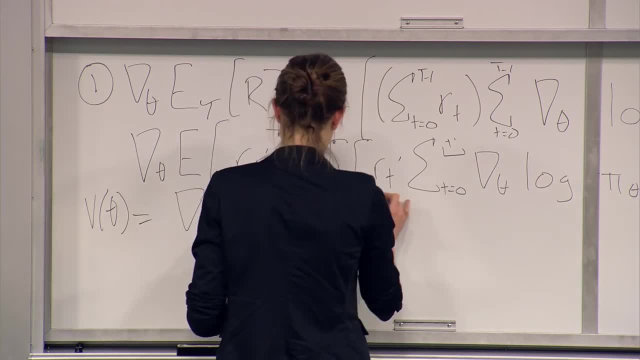 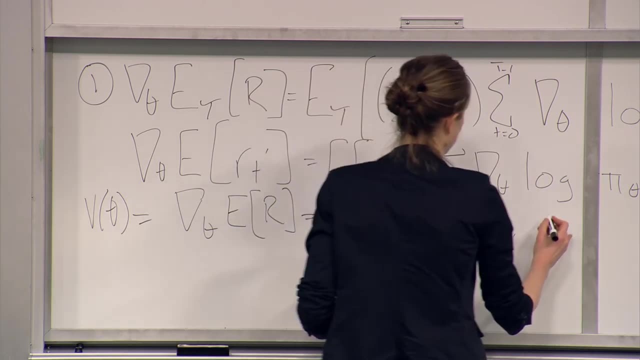 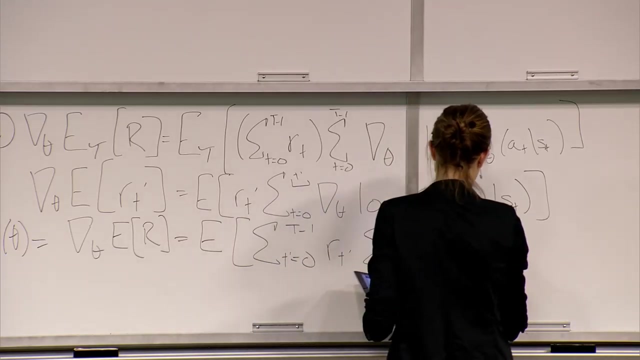 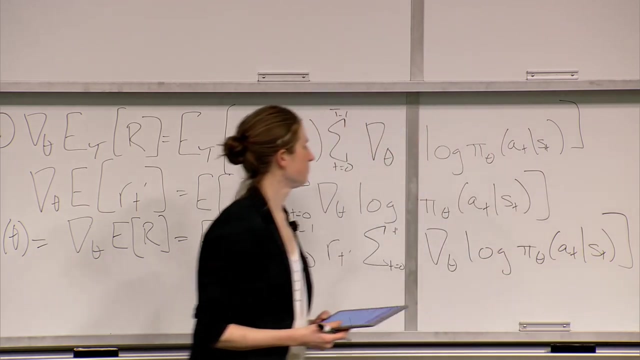 And I'm going to sum up that internal expression. So I'm going to sum over t prime is equal to zero to t minus one r t prime And then insert that second expression. Okay, So all I did is I put that in there and I summed over: t prime is equal to zero all the way up to t minus one. 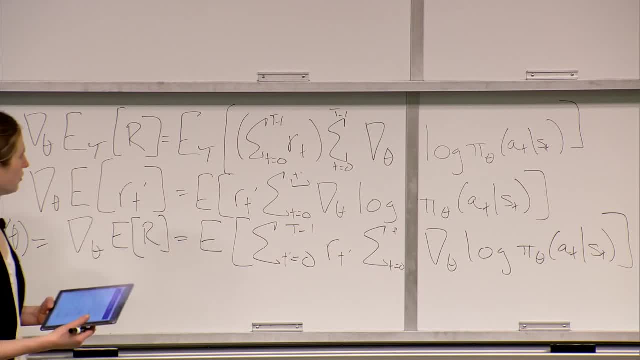 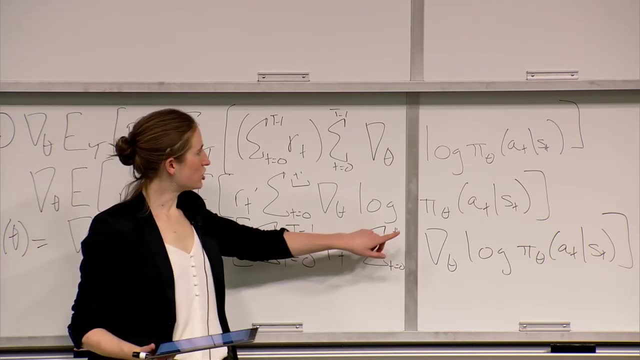 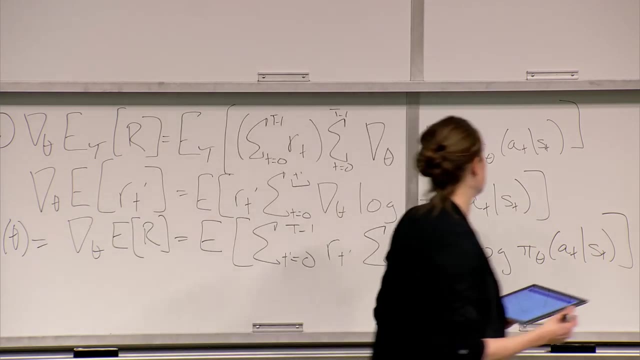 And then what I'm going to do is I'm going to reorder this and this by making the following observation: So, if we think about how many terms one of these particular log- pi theta, a, t, s, t- appears in, So if we look at log of pi theta of a, 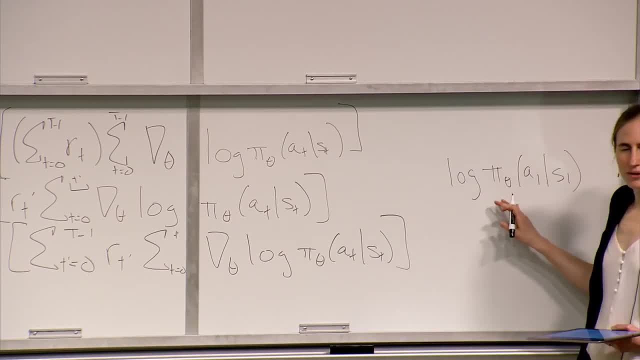 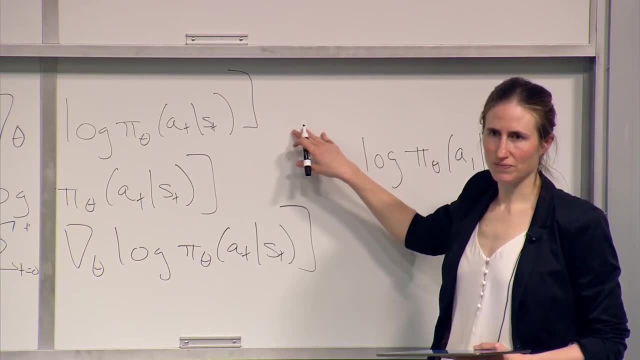 one s one. So if we look at how many times that appears, That appears for the early rewards and it appears for all the later rewards too. Okay, This is going to appear for r one. This is going to appear for r two. 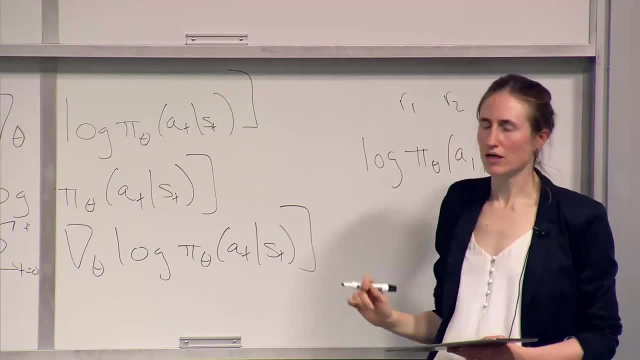 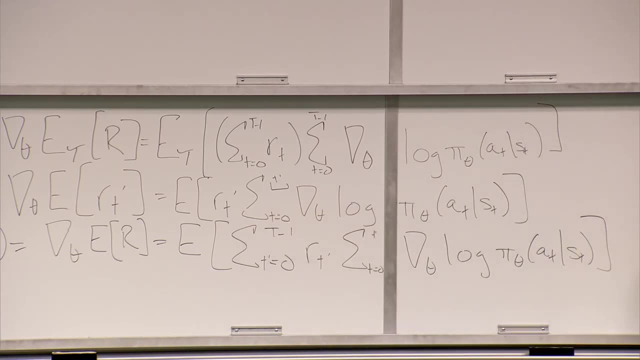 It's going to appear all the way up to r t minus one, Because we're always summing over everything before that t prime. Okay, So what we're going to do now is we're going to take those terms and we're going to just reorganize those. 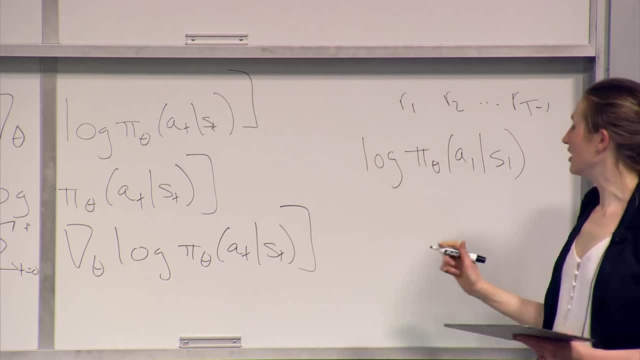 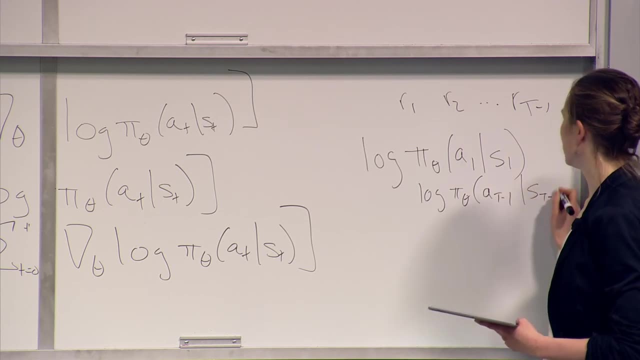 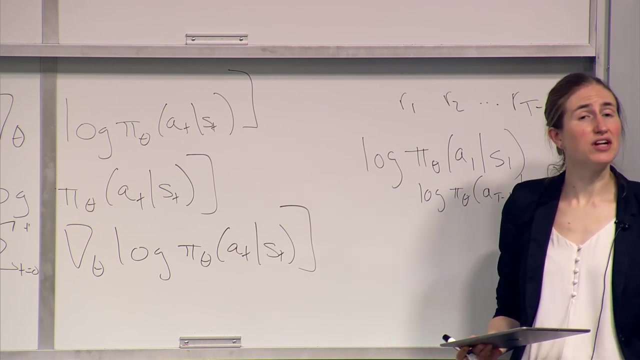 So some of these terms appear a whole bunch of time, Some of them. the last one, the log of pi theta of a t minus one, s t minus one. It's only going to appear once, It's only responsible for helping dictate the very final reward. 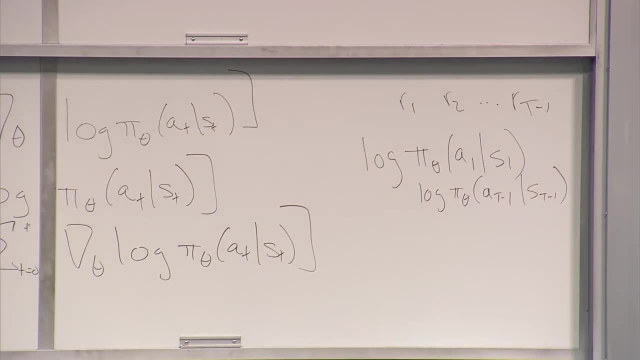 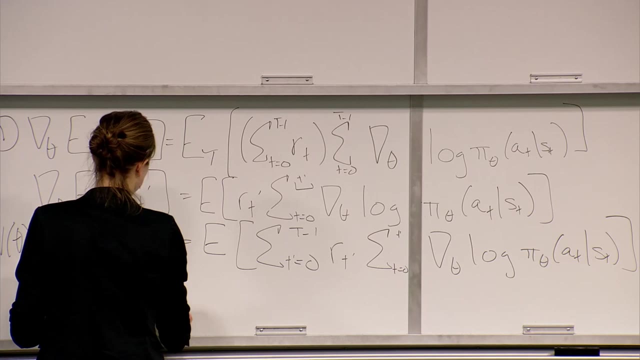 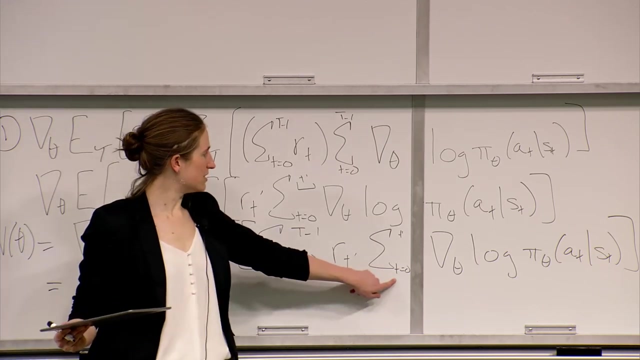 So we can use that insight to just slightly reorganize this equation as follows. So now we're going to say this is equal to the expected value of sum over t equals zero 0 to t minus 1.. So notice, before I had put the t prime on the outside and the t was on. 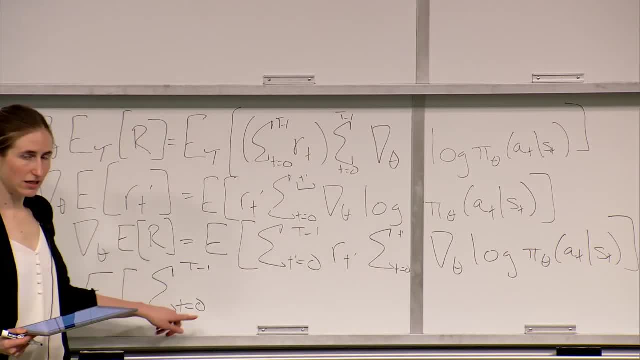 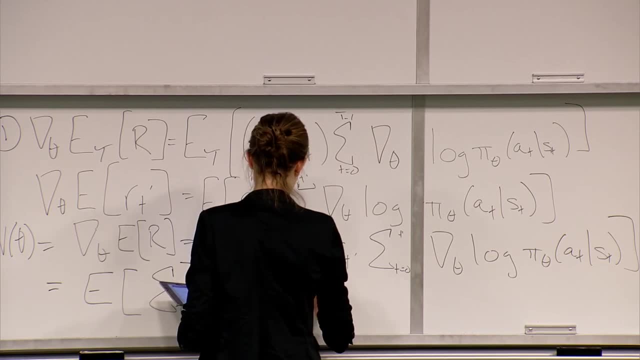 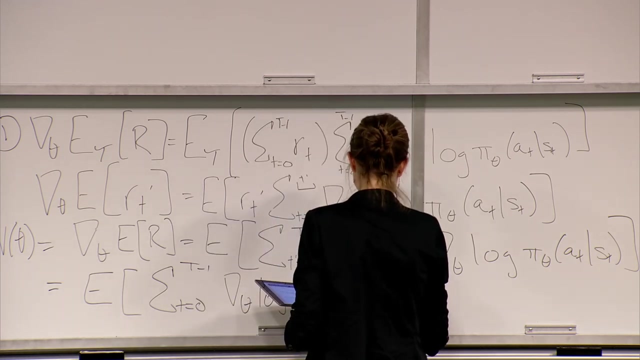 the inside. And now what I'm going to do is put the t on the outside And I'm going to say: I've got delta, theta, log pi theta, A, t, s, t times sum over t prime is equal to t, all the way to t minus 1 of r t prime. Okay, So all I've done is I've reorganized that sum. 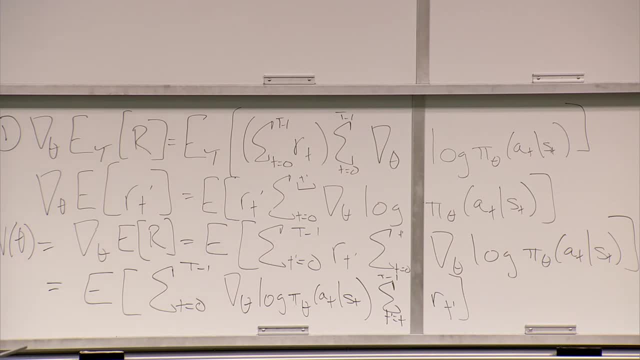 Yes, Is it? Yeah, Yeah. On the second line from the bottom, is it supposed to be the derivative The-? is that the value function with respect to theta? On the- at the very left: Yeah, Okay, Yes, Oh sorry. Do you mean this would be the derivative of this? 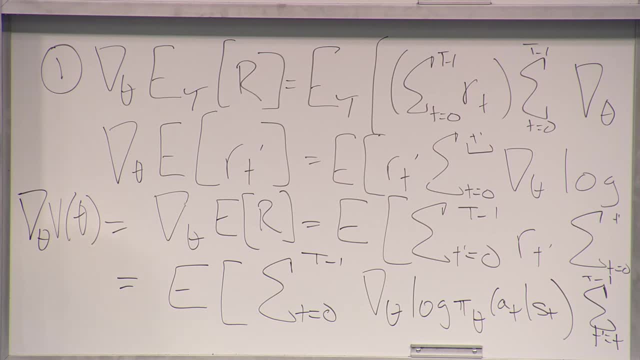 Yes, Yeah, Thank you, Okay. So what we've done in this case was we've reorganized the sum. we've reorganized the sum. we've just recollected terms in a slightly different way, But it's going to be done in a useful way. 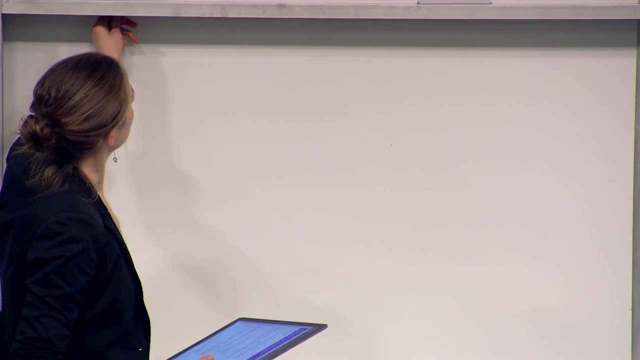 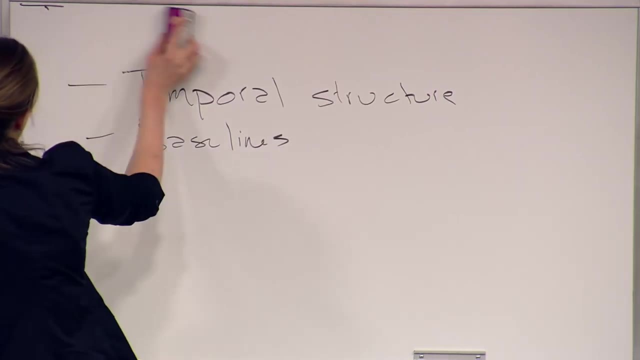 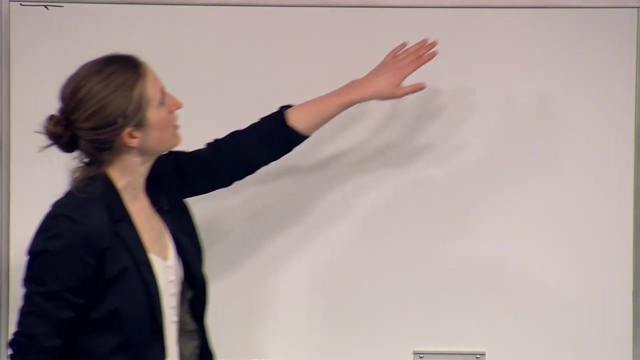 So let's move this up and I'll move this one down. Okay, So right now we're still working on the temporal structure. What is this going to allow us to do? Well, that second term there should look somewhat familiar. What that's saying here is that saying: 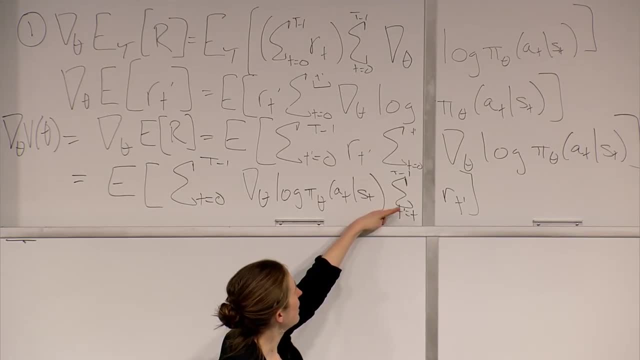 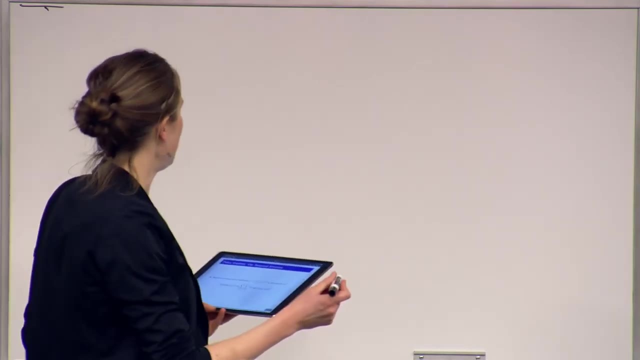 what is the reward we get? starting at time, step t, all the way to the end, And that's just the return. So we had previously defined that um when we were talking about like Monte Carlo methods et cetera, that we could always just look at. 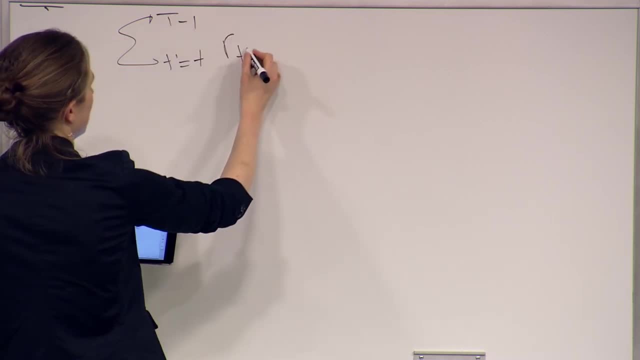 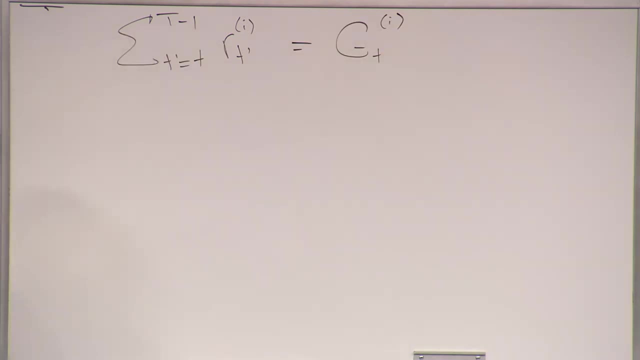 um rti, prime of i. This is just equal to the return, The return for the rest of the episode starting in time step t on episode i. So that- that should look very familiar to what we had seen in Monte Carlo methods. 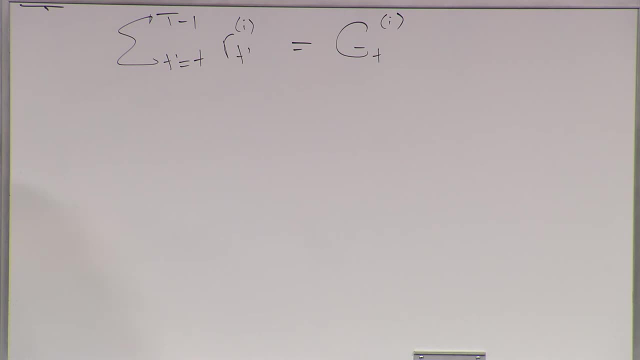 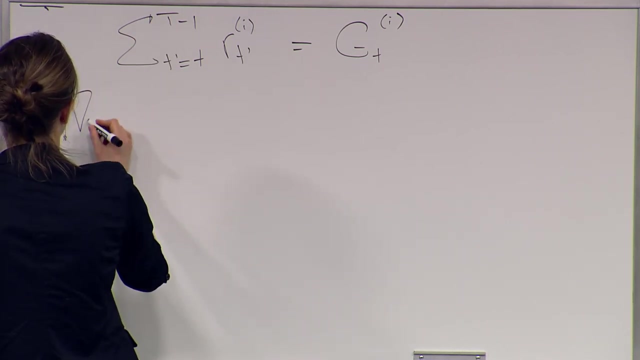 where we could always say from this state in action what was the sum of rewards we get, starting in that state in action until the end of the episode. Okay, So that means we can re-express the derivative with respect to Theta as approximately 1 over m. 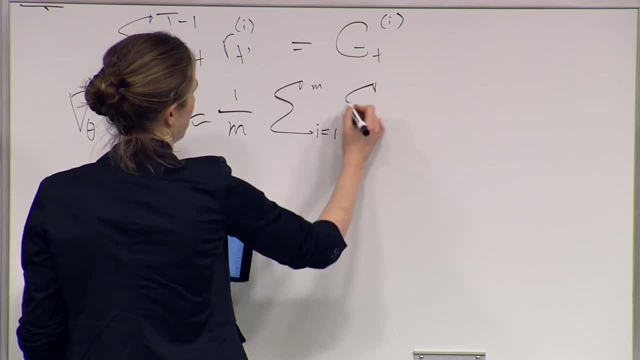 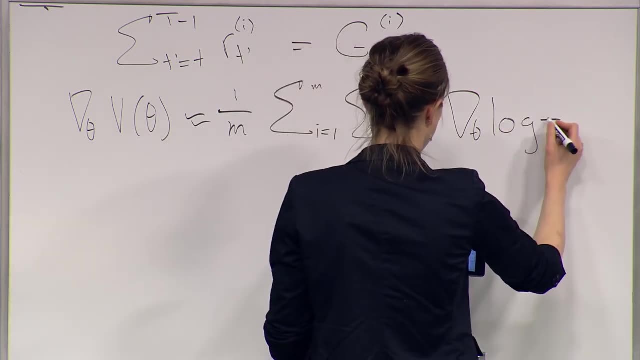 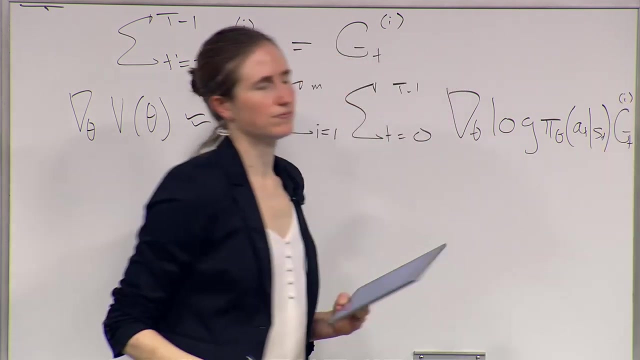 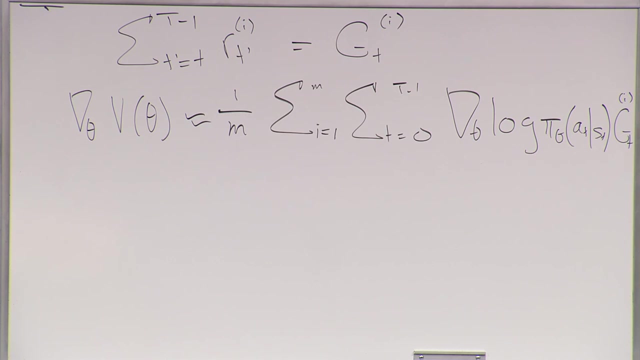 sum over all of the trajectories. we're summing over, sum over all the time steps. the derivative with respect to Theta of our actual policy parameter times, just the return, And this is gonna be a slightly lower variance estimate than before. Okay, So instead of us having to sort of separately sum up all of our words, 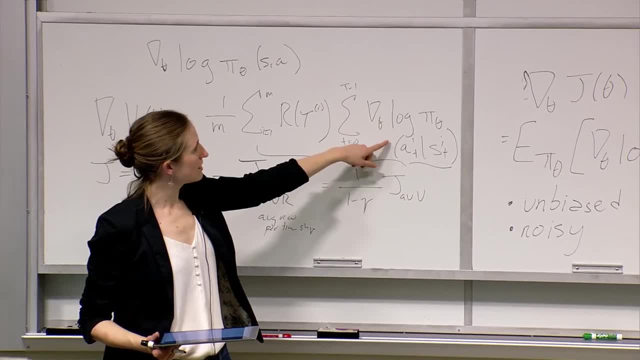 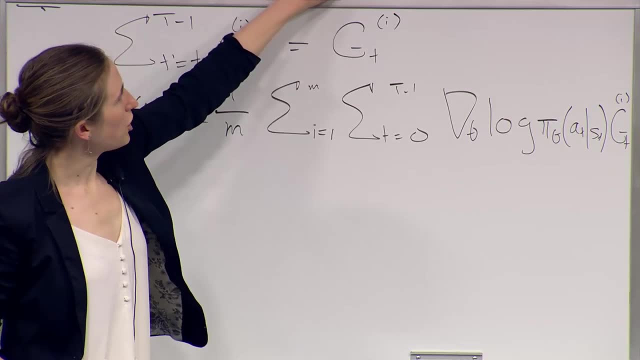 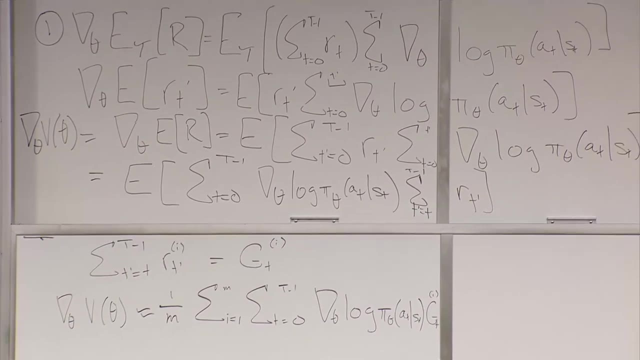 and then we multiply that by the full sum of all of these derivatives of the logs. we're only kind of needing to take this sum of the logs- erm for some of the Reward terms, essentially- And we can reduce the variance in that case. 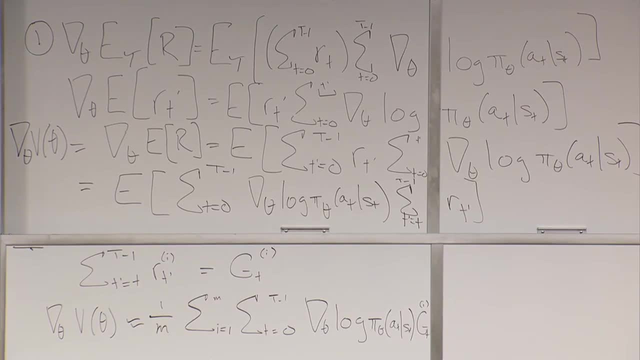 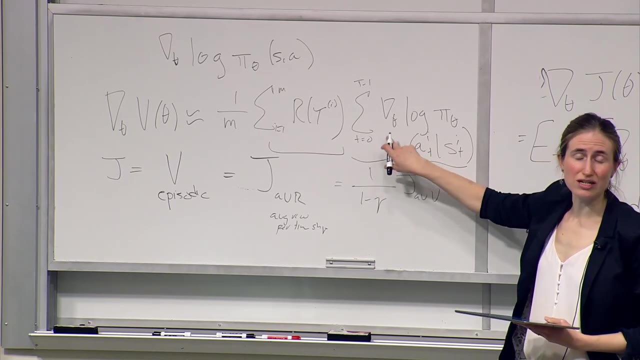 Cuz. in some ways, what this is doing, this is saying, like, for every single reward, cuz you could re-express this as a sum of rewards- For every single one of those rewards, you have to um sum it by sort of the tool trajectory in terms of the derivative of the gradient. 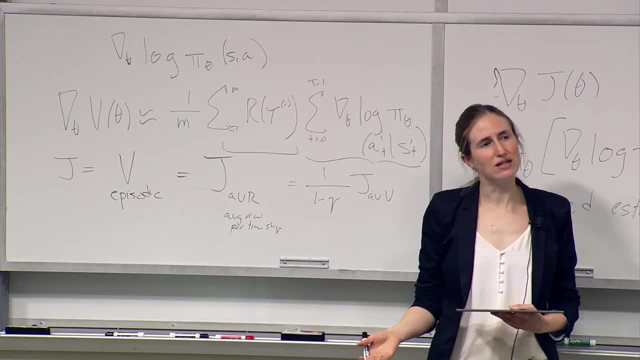 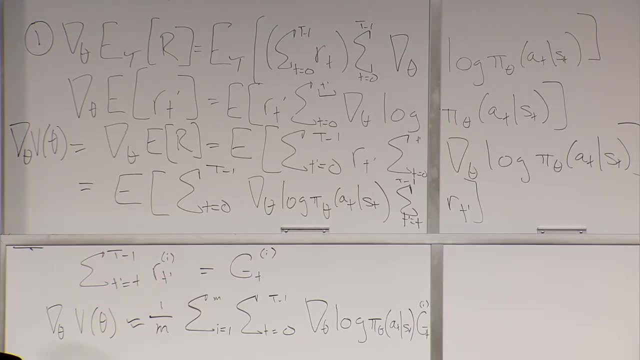 the derivative of the policy parameters. And now we're saying you don't have to multiply that by all of those, you only have to multiply it by the ones that are relevant for that particular reward. So that means that you're gonna have a slightly lower variance estimator. 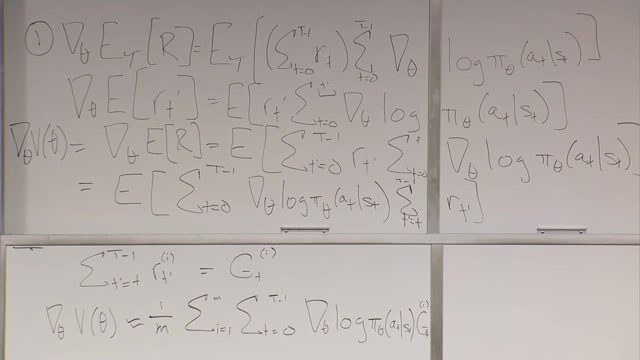 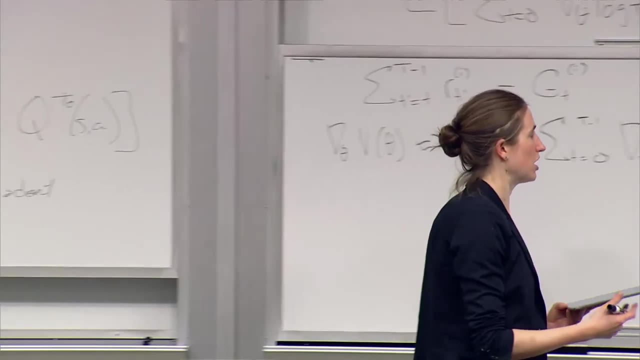 So when we do this, we can end up with what's known as reinforce, which, um, who here has heard of reinforce? Yeah, a number of people, not everybody. Reinforce is one of the most common reinforcement learning policy grading algorithms. 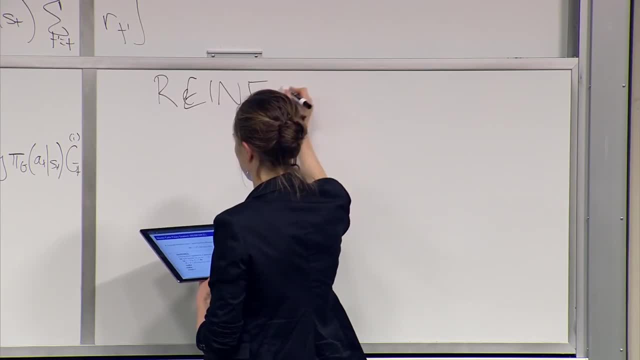 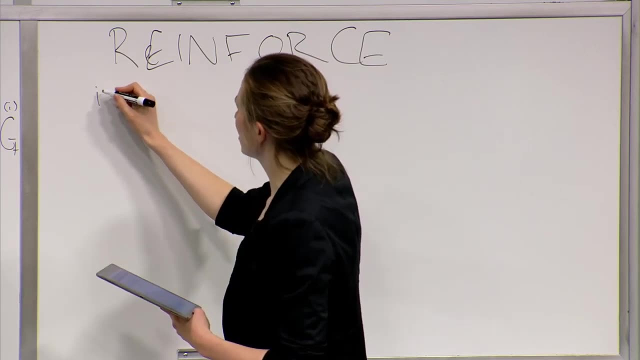 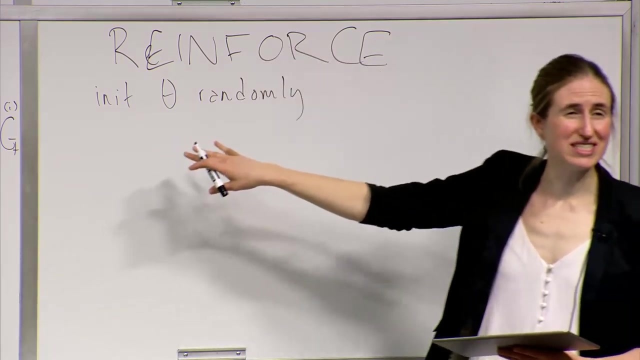 So you get the reinforce algorithm. So what- how it works, is you? um then the algorithm is you initialize init theta randomly. You always will have to first decide on how you're parametrizing your policy. So somewhere you already defi- decided how you're parametrizing your policy. 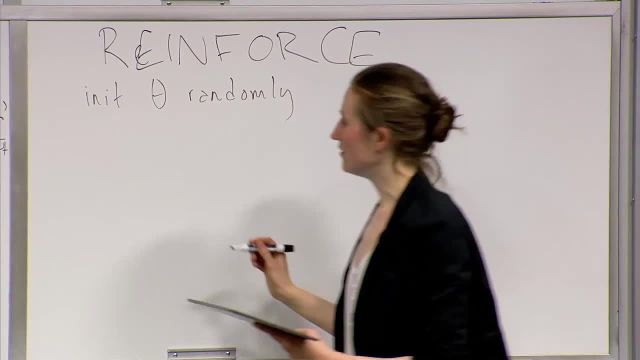 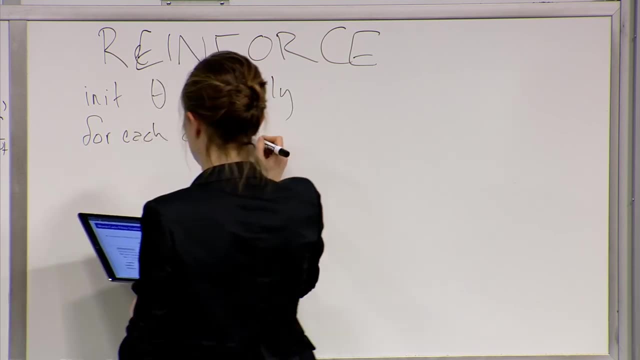 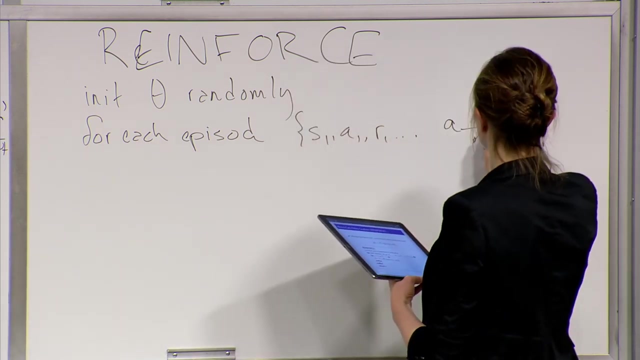 now you're gonna set the values for that policy randomly And then for each episode, so you're gonna run an episode, an episode with that policy, So, and you're gonna gather a whole bunch of actions and rewards, And this is sampled from your current policy. 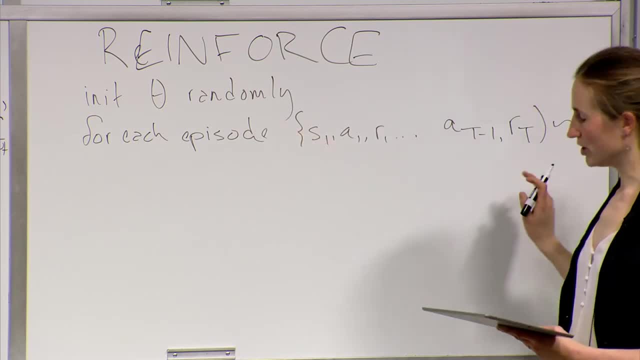 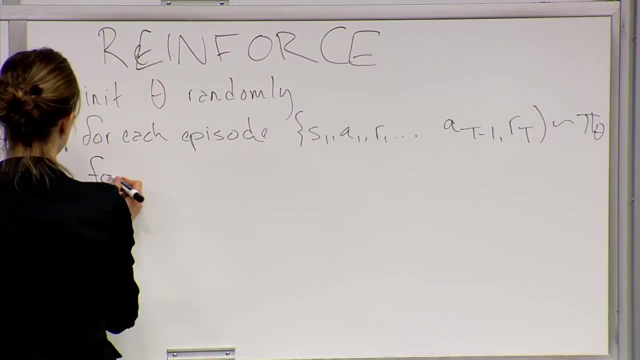 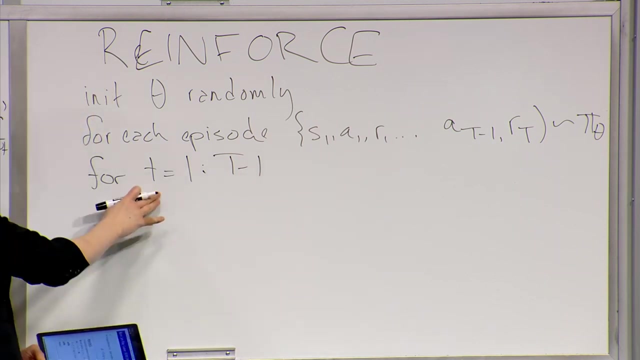 So you sample your current policy. according to um sample from your current policy, you get a trajectory And then for every step in that trajectory you're gonna update your policy parameters. So for every time-step inside of that episode, 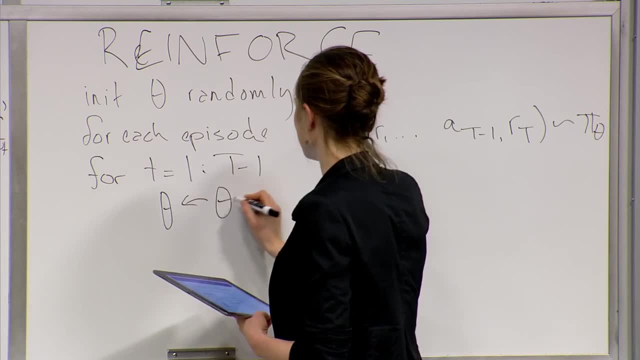 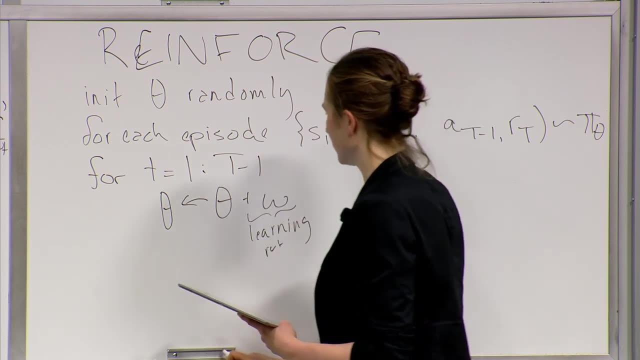 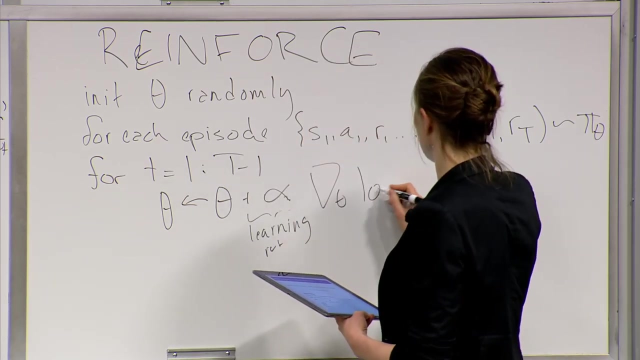 we're gonna update our policy parameters, So it's gonna be the same as before. times, some learning rate, Oop. I will not use W there, I'll use alpha times. the derivative with respect to theta, log pi: theta is 80.. 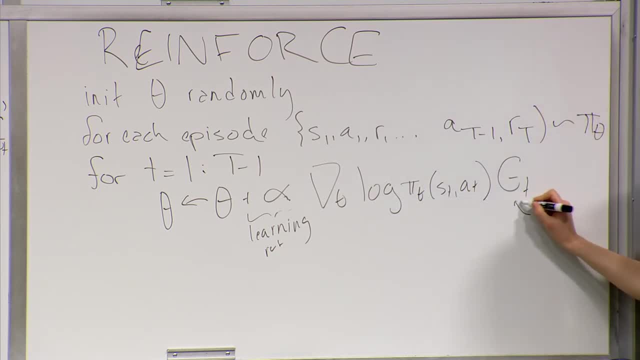 Okay, gt, where gt is just in this episode. what is the sum of rewards from ST AT onwards? So that's the, just the normal return, like what we had with, uh, Monte Carlo methods. So just like what we did when we were estimating, like the linear value function. 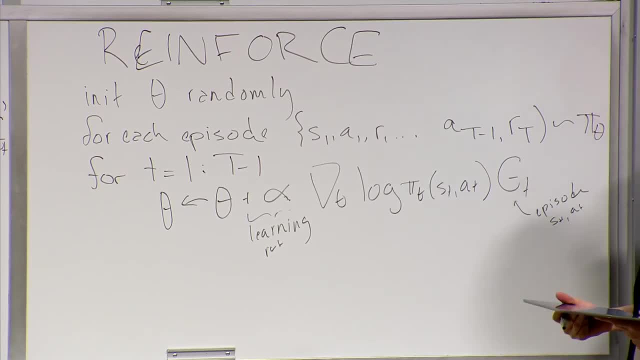 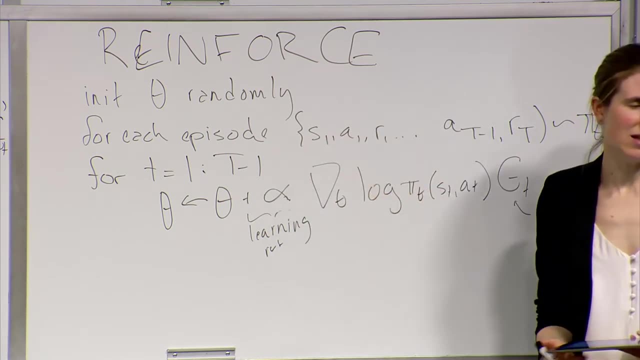 and we were using rewards from the state and action onwards. we're gonna do the same thing here, except for, um, we're gonna be updating the policy parameters, And we do this many, many, many times, and then at the end, we return the Theta parameters. Yeah, 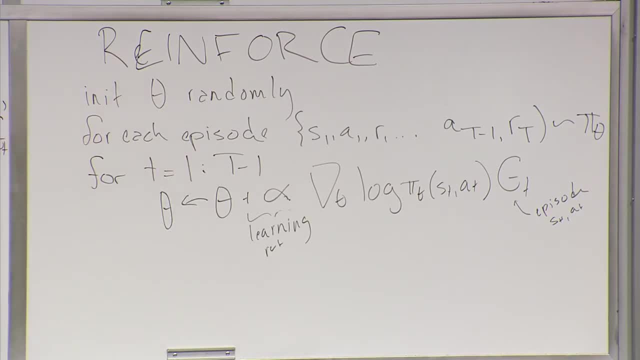 I have a question. So for each episode, do you sample from the updated uh policy where you've already updated? Oh, yeah, Yeah, So that is right. So in this case you um uh, after you do all of the updates for one episode. 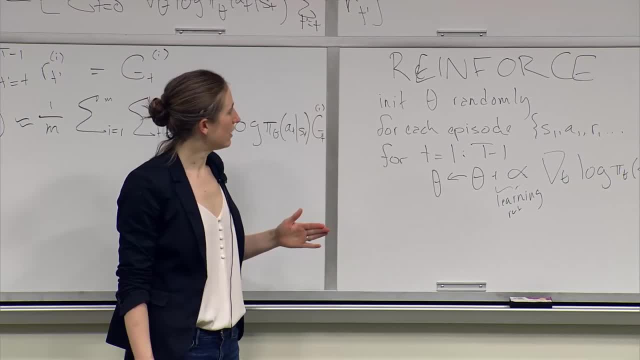 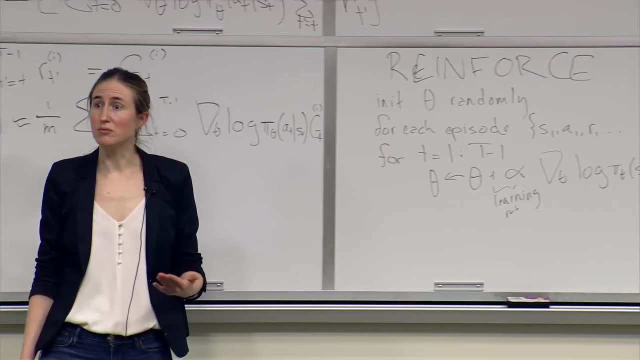 so you could do these incremental updates. um, uh, and then, at the end of doing all of your incremental updates, you can do these incremental updates. Then you get another episode with your new updating parameters. Yeah, Um, since we're doing every time updates. 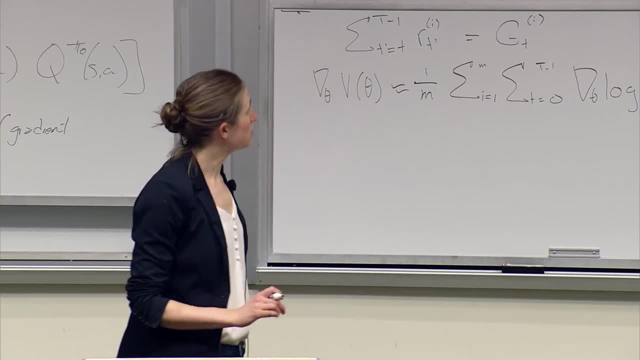 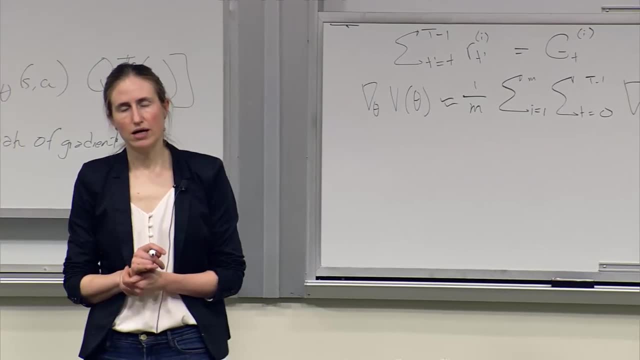 would this be a biased method? Um, good question. So since we're doing every time as it is, um, this should be an unbiased estimate of the? um. uh, this should still be an unbiased estimate of the gradient. It's stochastic. Um, but um, we. 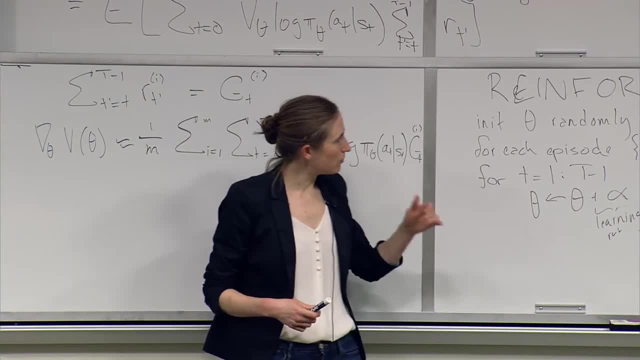 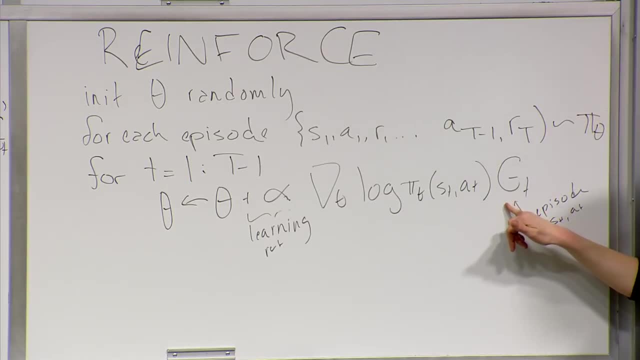 there's not a notion of state and actions in the same way, Um, this will be asymptotically consistent. It's a good question. So the notion of um- a state and action, in this case is different because we have just these policy parameters. 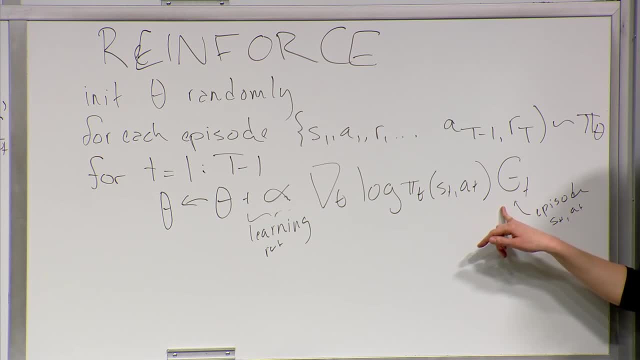 So we're not estimating the value of a state and action here. Um, so this is certainly asymptotically consistent. I think it's still just unbiased. Um, uh, if I- if I reconsider that later, I'll send a Piazza post. 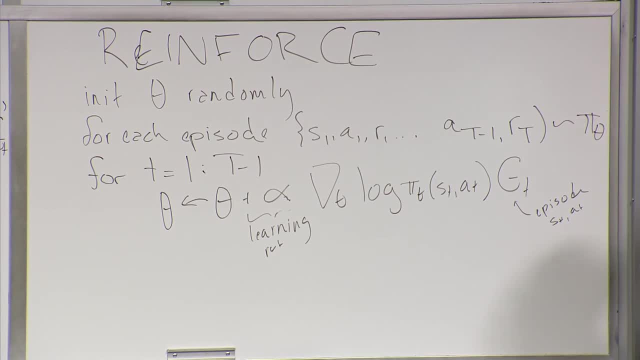 Um, but I think it still just, uh, an unbiased estimate of the gradient. It's a good question, Okay, So let me go back to my notes. Um, I think the last thing I just wanted. well, I'll, I'll mention a a couple of things. 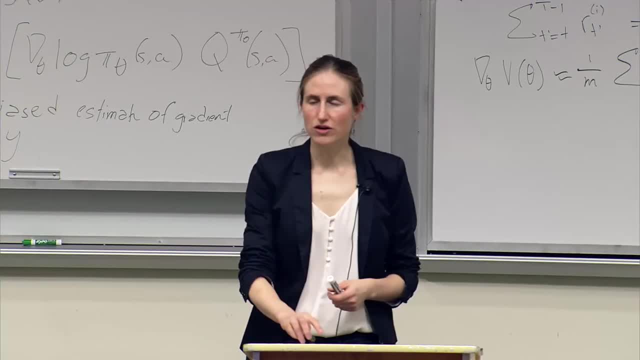 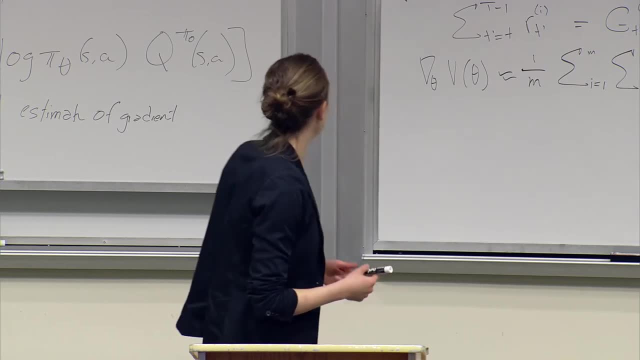 Well, um, one critical question here is whether or not or how to compute this differential with respect to the policy parameters. So I think it's useful to talk about, you know, what are the classes of policies that often people consider, um, that have nice differentiable forms. 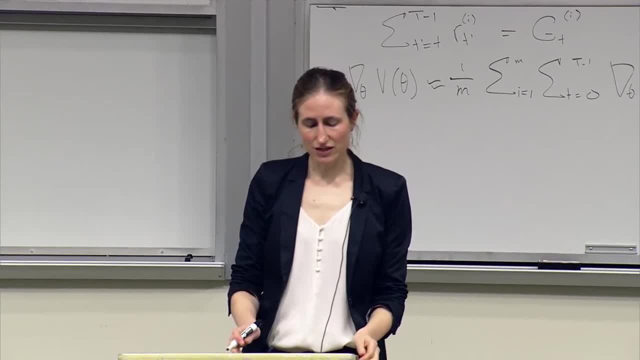 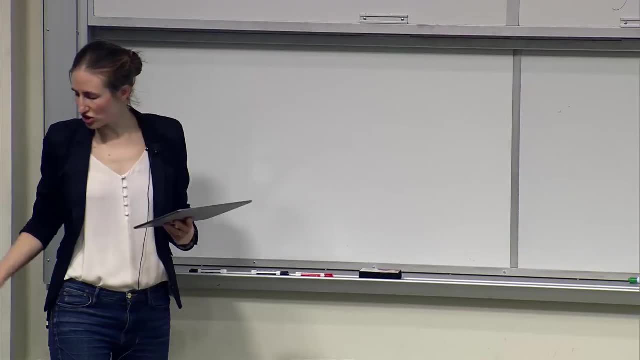 So, um, some of the classes people considers are things like softmax, Gaussians and neural networks. Those are probably the most common. So, and what do I mean by that? I mean that's how we're gonna actually just parameterize our policy. 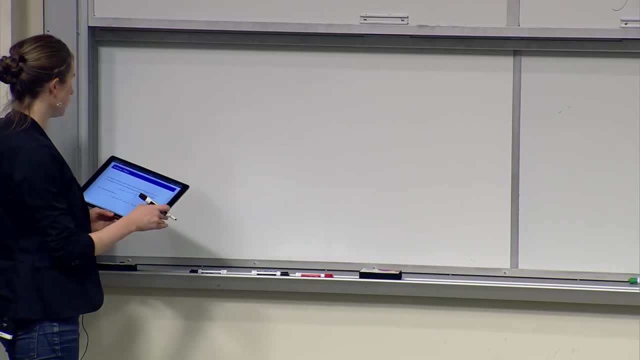 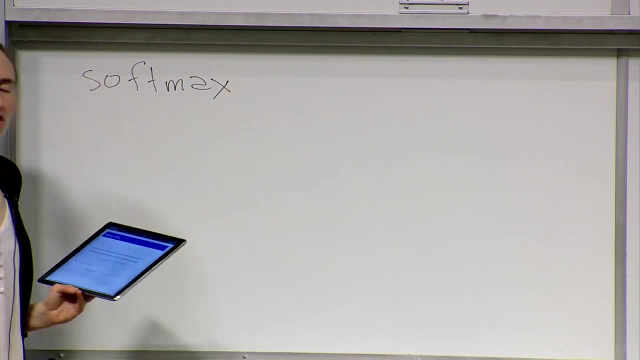 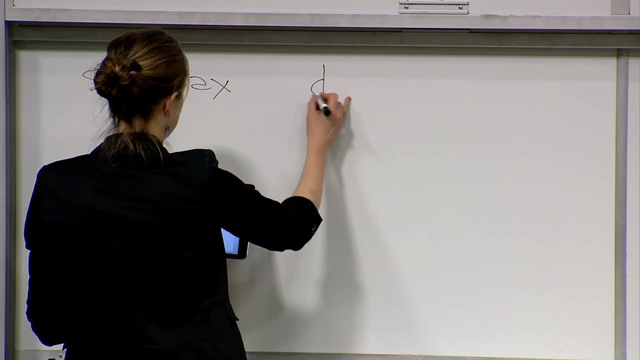 So let's just look at an example. So softmax is where we simply have a linear combination of features and we take sort of um an exponential weight of them. So what we're gonna do is we're gonna have some features of our state and action space. 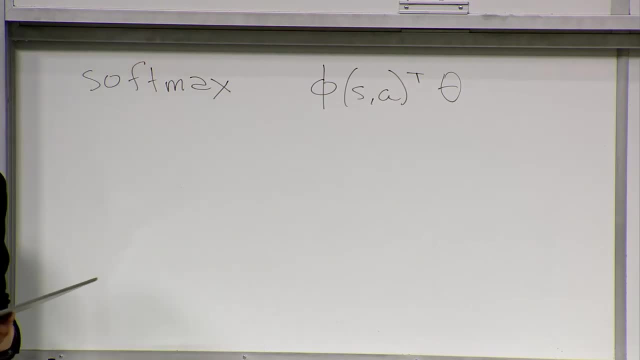 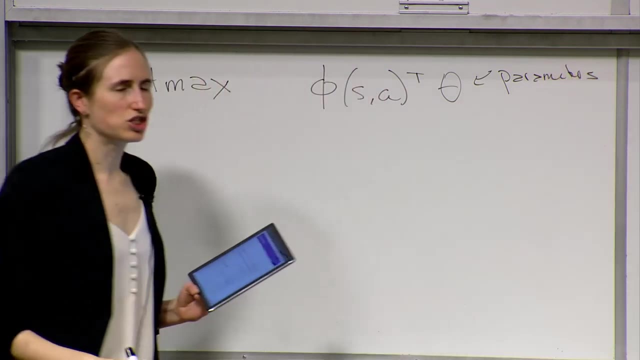 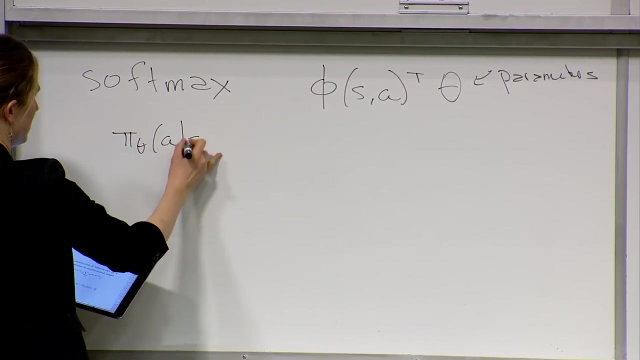 and we're gonna multiply them by some weights, our parameters, These are our parameters- And then to actually get a probability of taking an action. So if we wanna have our policy where we say what is the probability of action given a state? 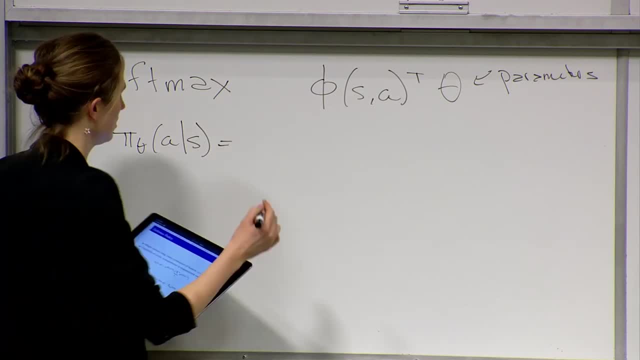 We're gonna take the exponential of these weighted states. Okay, So we're gonna take the exponential of these weighted states. We're gonna take the exponential of these weighted states. Okay, So we're gonna take the exponential of these weighted states. 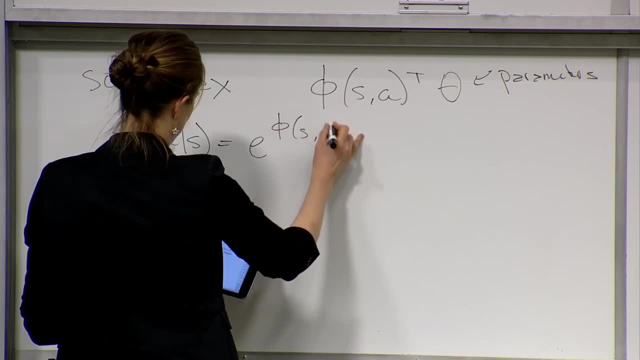 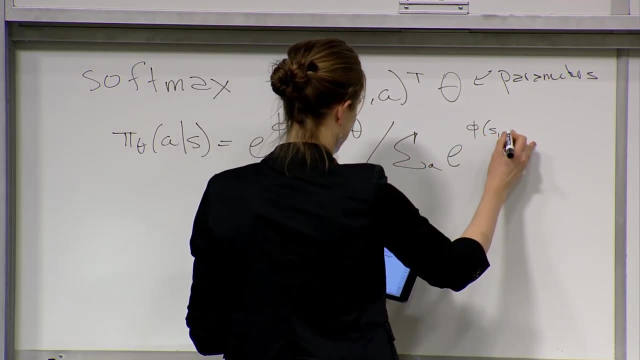 So we have e to the phi t theta divided by the sum over all actions. Okay. So we have e to the phi t theta divided by the sum over all actions. Okay, So we have e to the phi t theta divided by the sum over all actions. 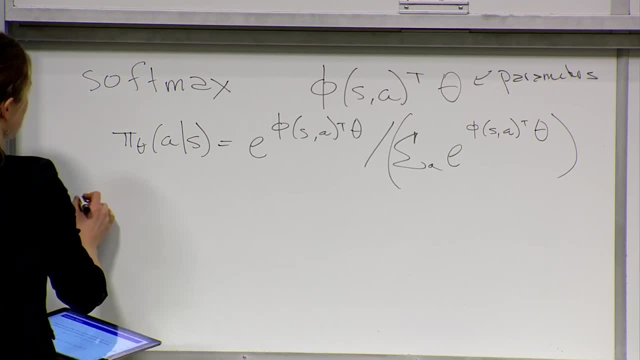 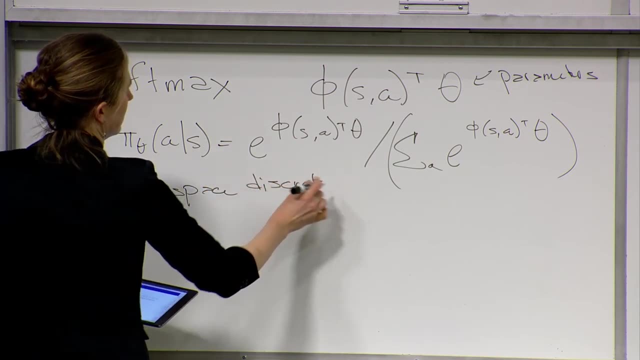 So notice, this is a reasonable thing to do when our action space is discrete. Action space discrete, So a lot of Atari games, a lot of different um scenarios. you do have a discrete action space, Um, so you can just take this exponential. 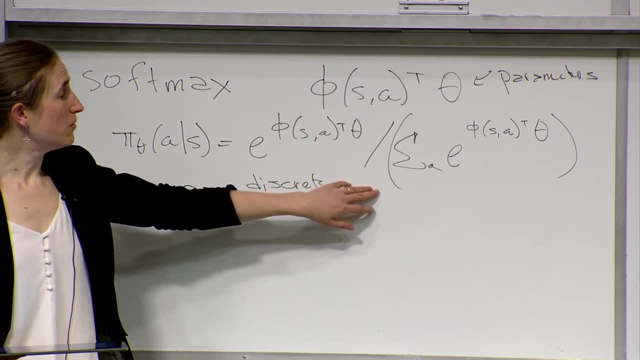 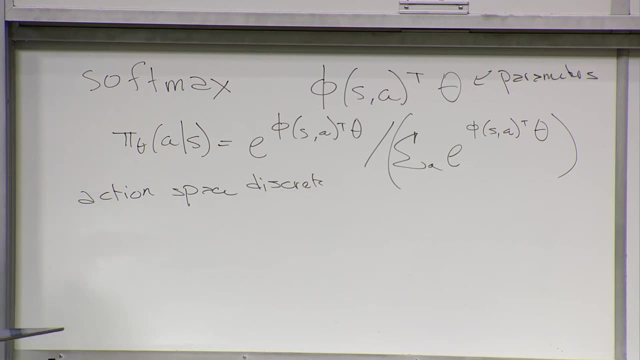 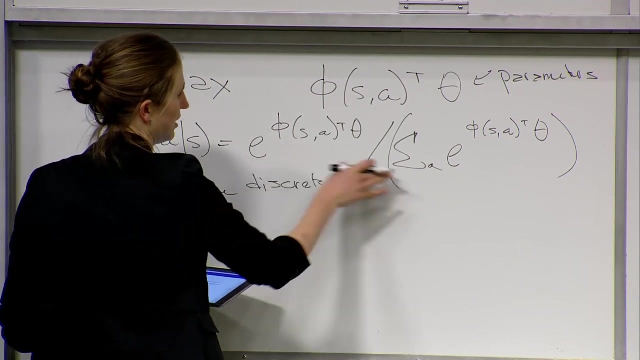 divide by the normalized um sum over the exponential, and that immediately yields our parameterized policy class. And so then, um, if we want to be able to take the derivative of this with respect to the log, that's quite nice, because we have exponentials here and we have log- we're taking the log of this. 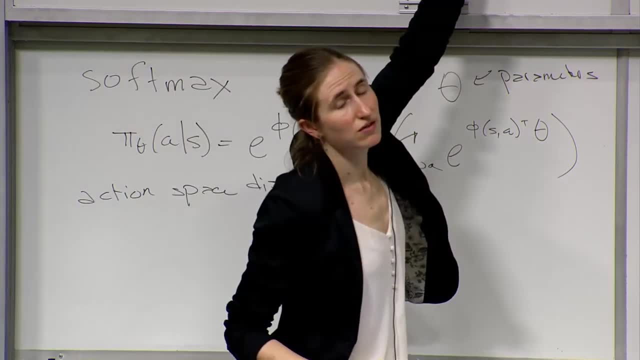 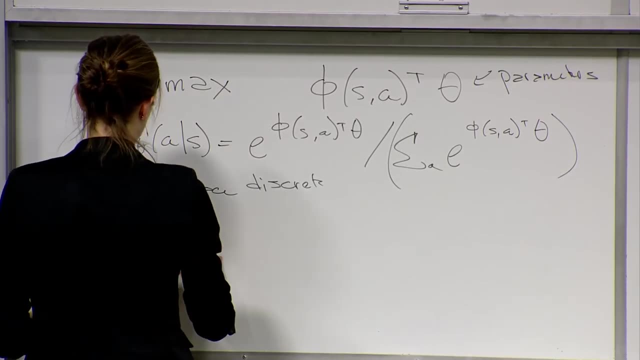 So, um, if we wanna be able to compute this term from this sort of um parameterized policy class, what we get is the derivative with respect to theta of log of this type of parameterized policy is just equal to our features. 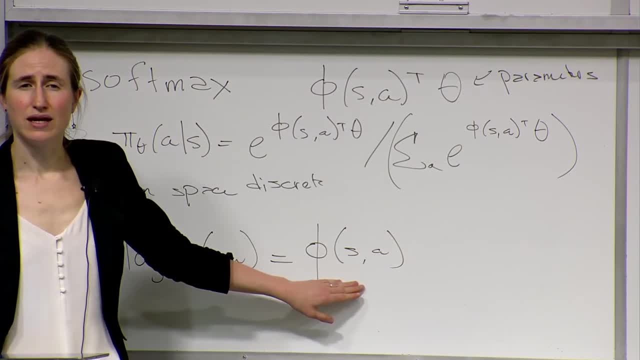 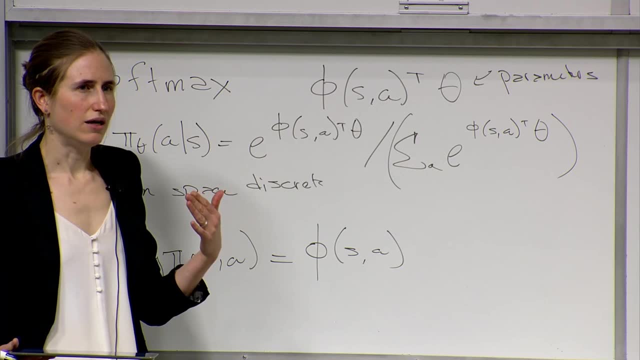 So this is whatever feature representation we're using, Like in the case of the- um uh, locomotion robotic case. this would be like all the different um uh, this could be something like, you know, angles or joints or things like that. 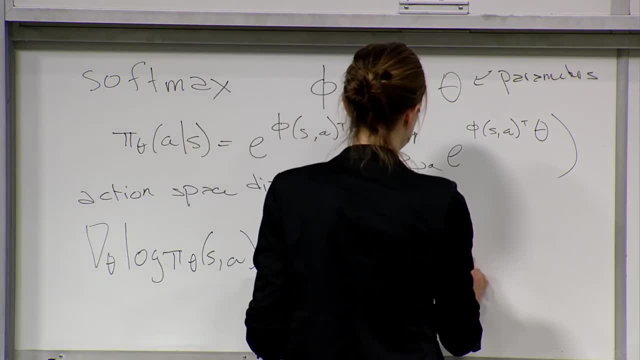 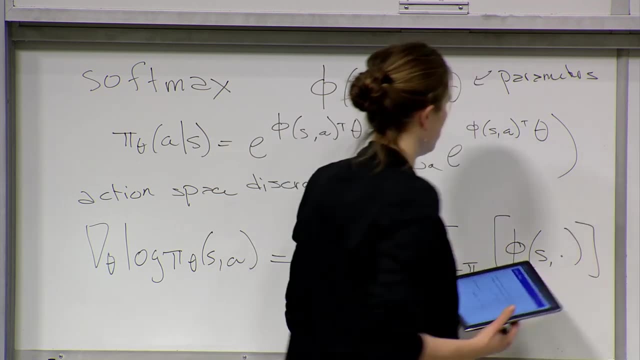 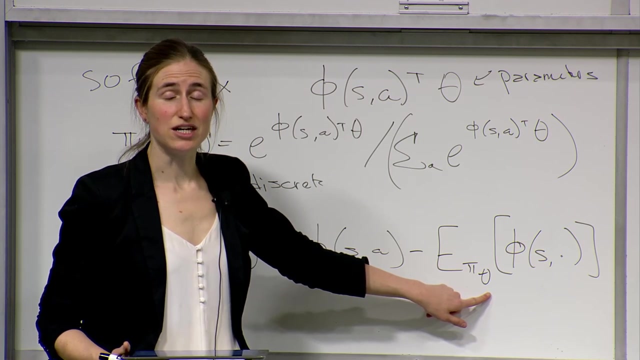 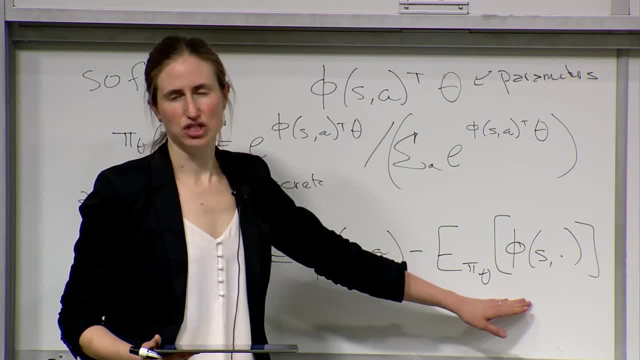 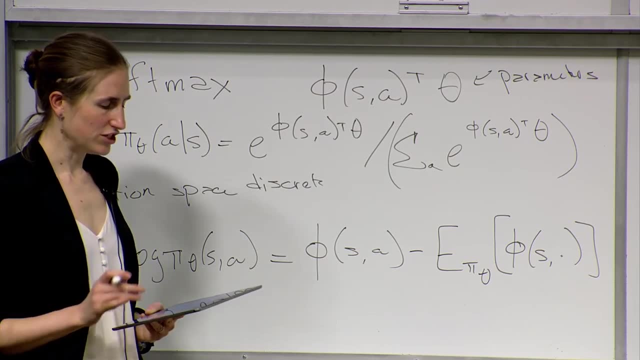 So it's sort of saying the features that you observed versus the sort of average feature, average- averaged over the action. Okay, So that's differentiable um and you can solve it. then it gives you an um, an analytic form. 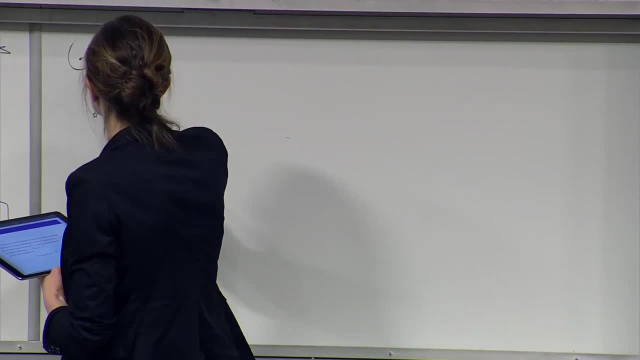 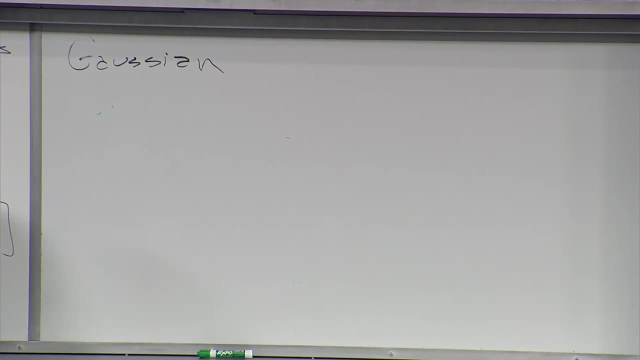 Um, another thing that's really popular is a Gaussian policy, And why might this be good? Well, this might be good because often we have continuous action spaces, So this is good if we have discrete action spaces. Often we have continuous action spaces. 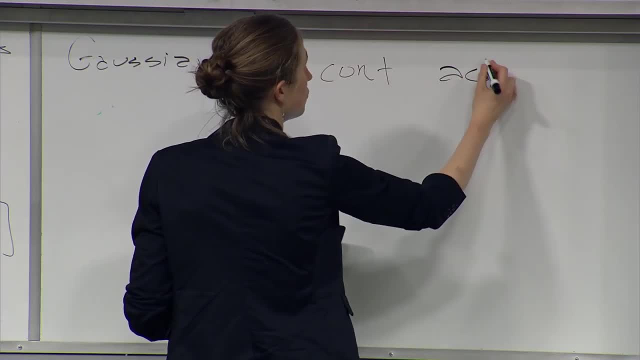 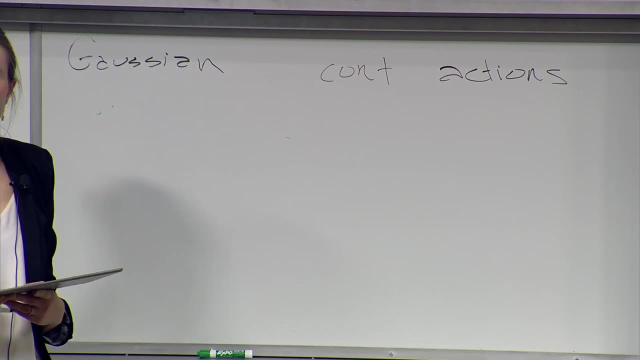 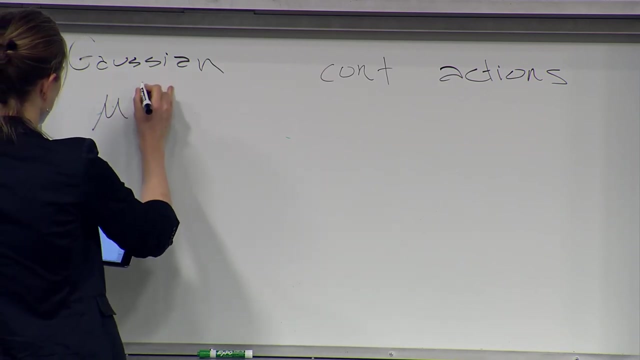 This is very common in um controls and robotics. So you have a number of different parameters in in in the continuous scalar values that you want to be able to set Um, and what we could say here is, let's say, we use mu of s. 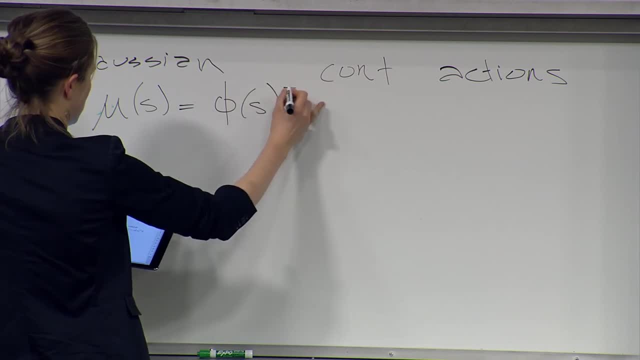 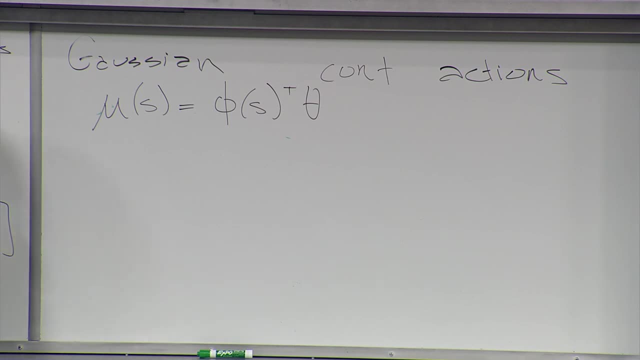 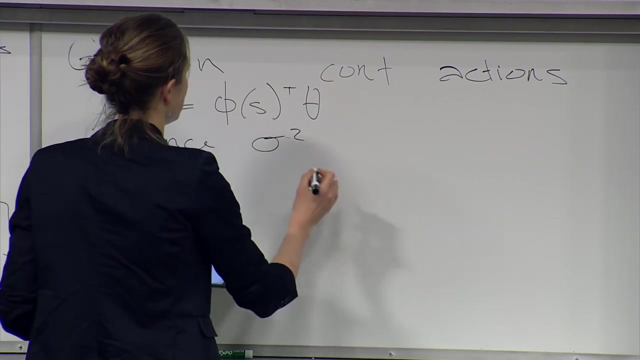 might be a linear combination of state features times, some parameter. Okay, And let's imagine for simplicity right now that, um, we have a variance, but that that's static. So we could also consider the case where it's not, but we're going to assume that we have some variance term that is fixed. 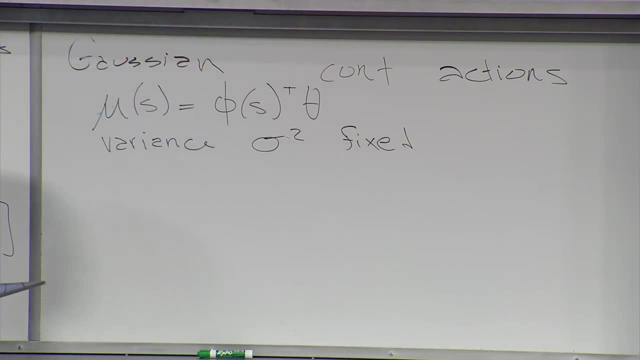 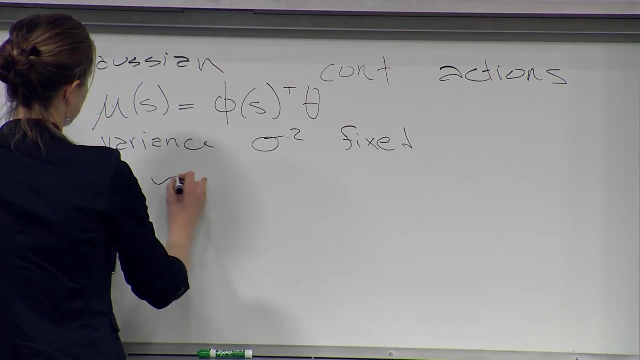 So this is not a parameter, This is not something we're going to try to learn. We're just going to be trying to learn the theta that's defining our mu function, And then our policy is going to be a Gaussian, So A is going to be drawn from a Gaussian, using this mean for features. 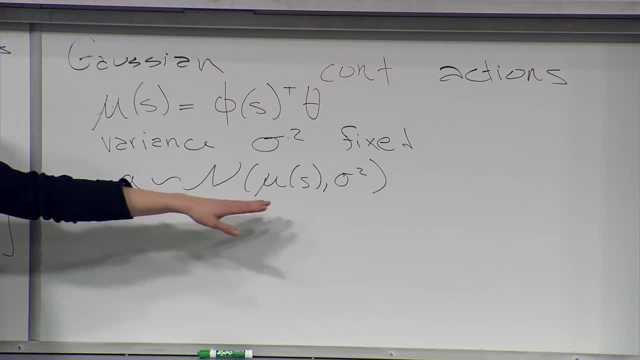 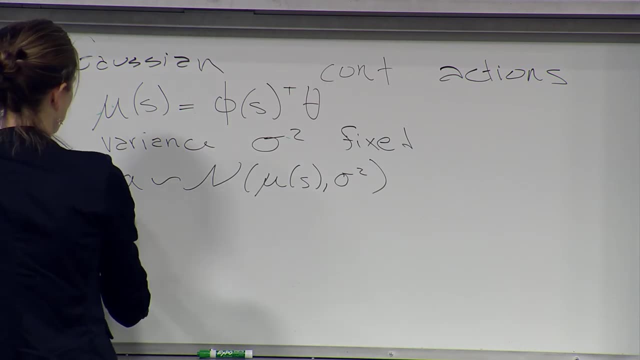 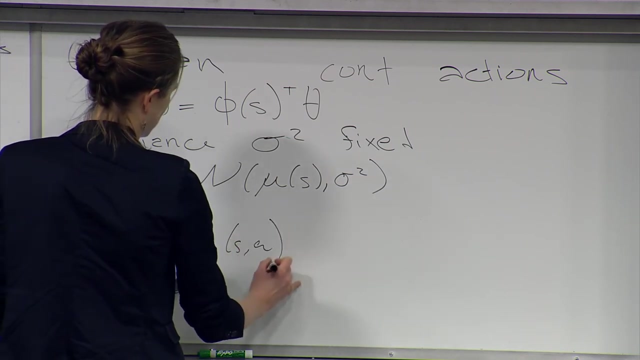 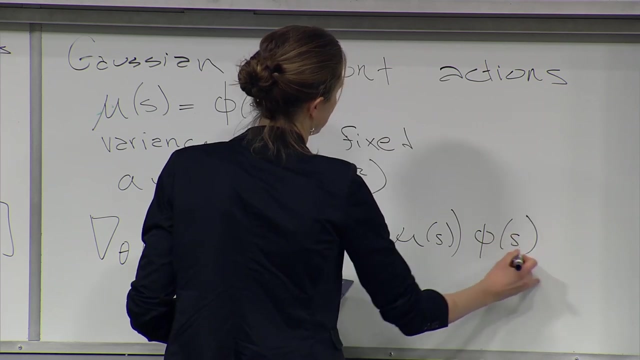 So we compare our current state to the mean and then we select an action with respect to that. And the score function in this case is the derivative of this Gaussian. So score is a derivative of this Gaussian function, Which ends up being A minus mu of s times our parametrization. 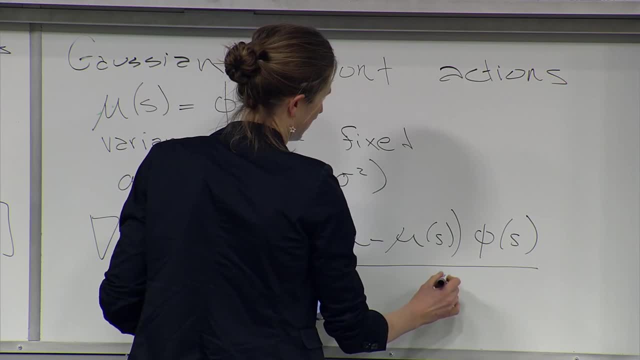 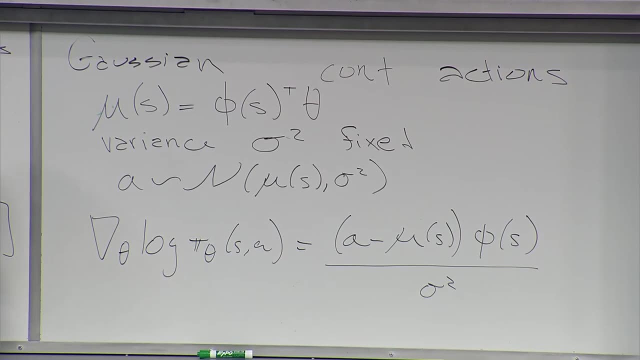 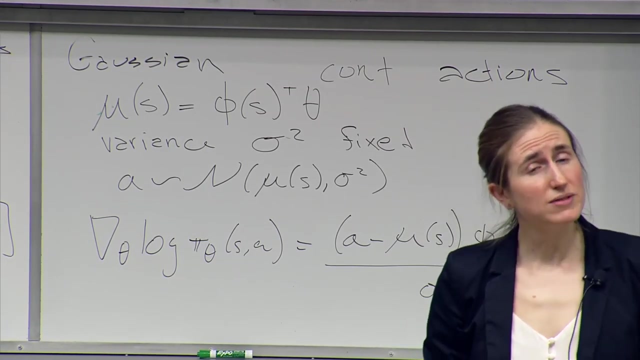 of the state features divided by sigma squared. So again it can be done analytically. And the other really common one is deep neural networks. So those are, um, those are the sort of very common forms, um, uh, that people use. 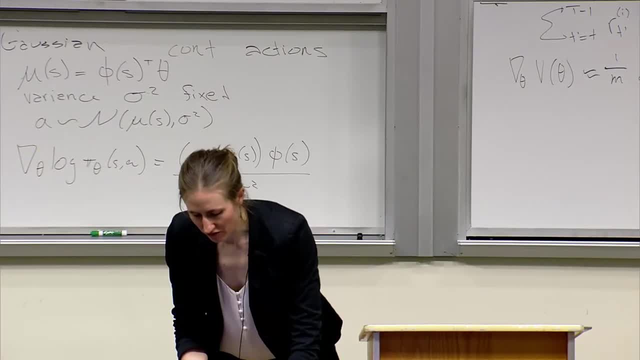 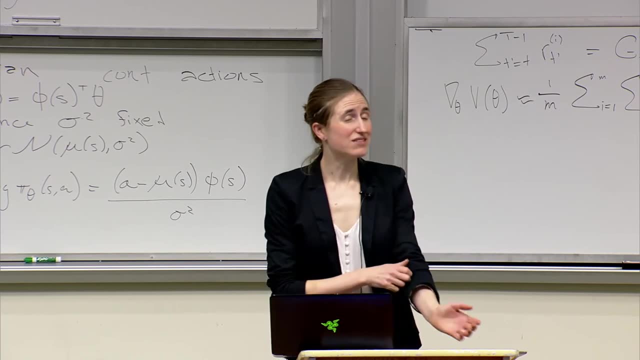 We're going to talk next time about another common way. Before we finish um, we're going to do um. spend about five minutes um to do some early class feedback. It's really helpful for us to figure out what's helping you learn. 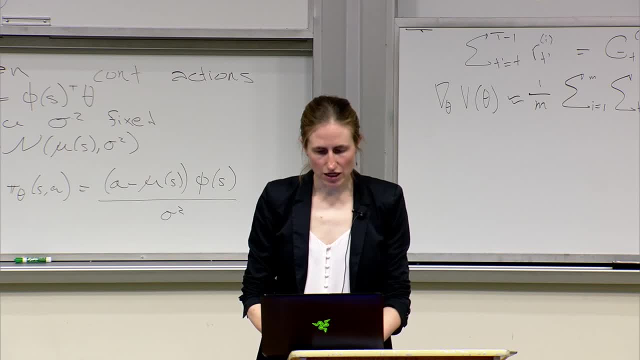 what things you think could be improved. Um, so what I'm going to do right now is open. if you guys could go to Piazza, um, it would be great if you could fill this out. All everything is anonymous, um. 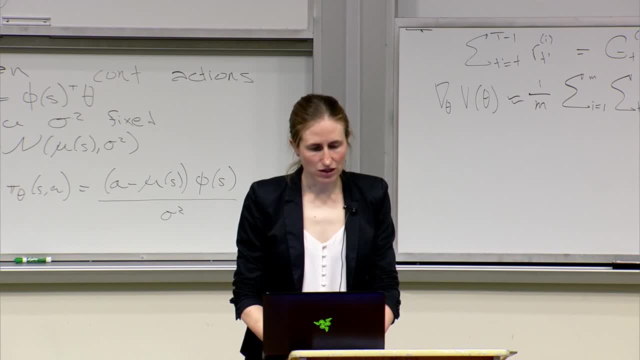 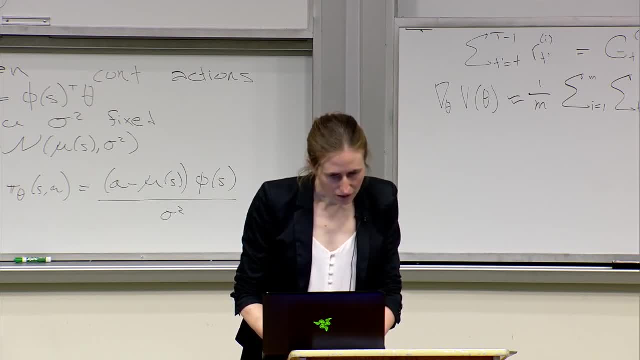 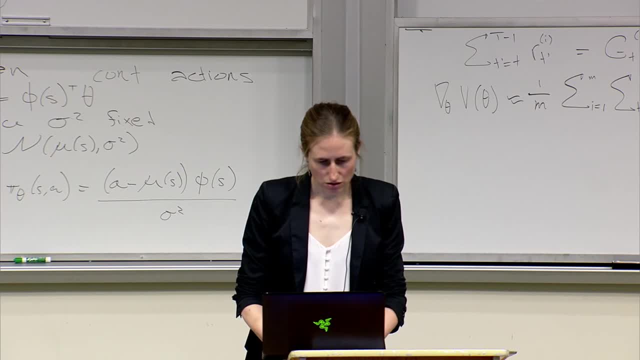 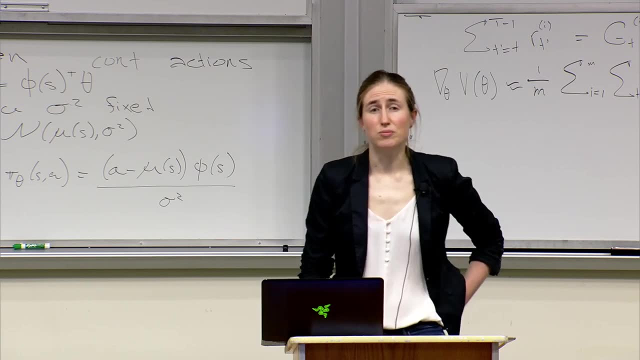 I'll pin it so it's easier to find. So it should be pinned now or at the very top: Yep, So mid-class feedback survey if you go to Piazza um. it's a very short survey. If you can give us information back, that would be great.